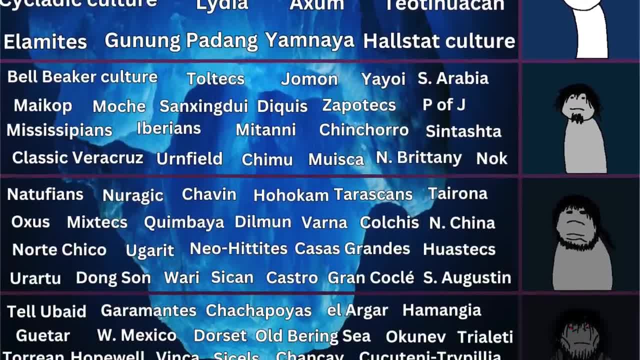 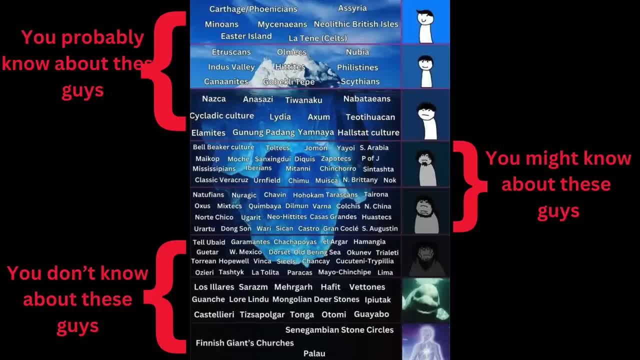 But I guarantee you that Even if you're a big archaeology buff, you'll learn about a couple cultures you haven't heard of before, Or at least you'll pick up a new factoid or two. The way the iceberg works is that the more obscure a civilization is, the deeper it'll be. 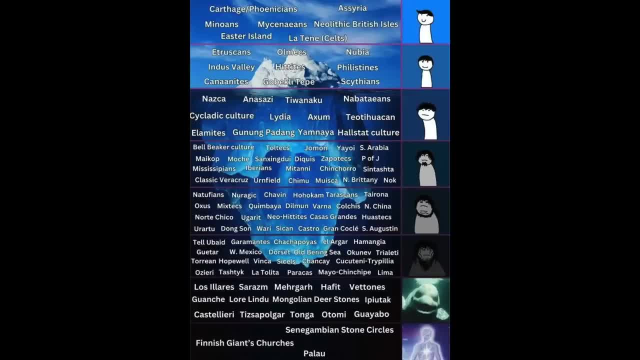 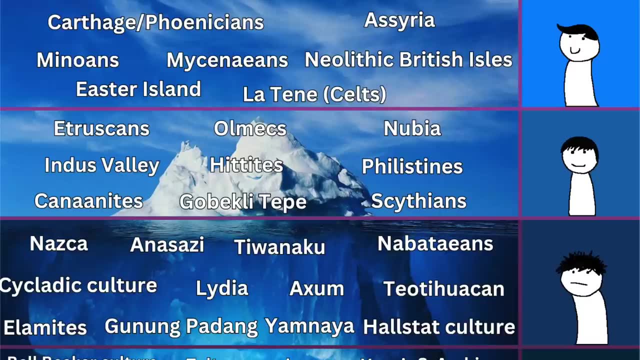 Unfortunately, the iceberg has so many names on it that this episode- yeah, there's gonna be more than one- will only be able to cover the first three layers of it. But that's still twenty-eight distinct civilizations, So the civs we'll be going through today aren't gonna be too too obscure. 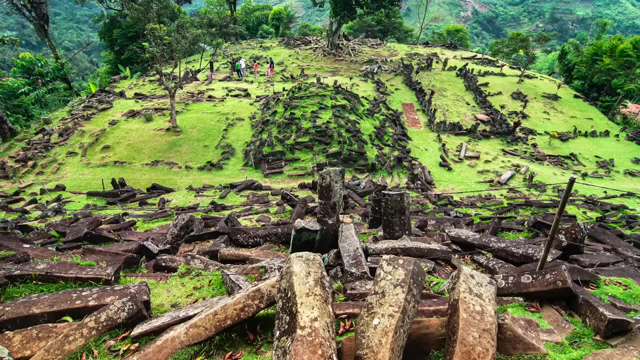 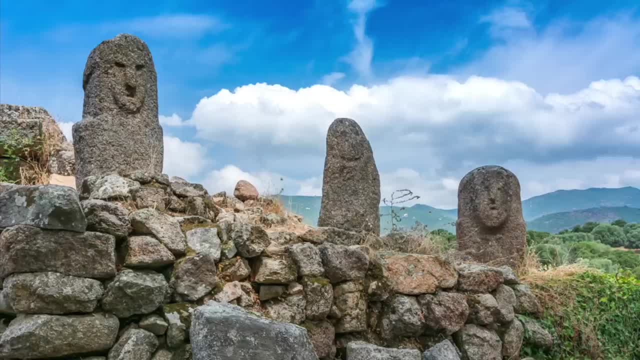 Also, you might say You might see a few that you might not regard as civilizations, and that's because I sort of use civilization and culture a bit loosely. As long as they left some sort of substantial mark on the archaeological record, like really cool art or huge monuments, I'm counting them in. 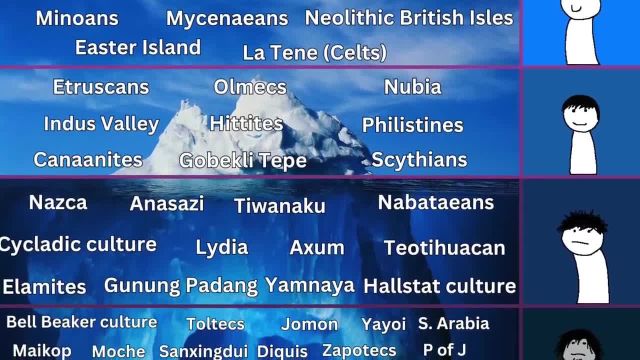 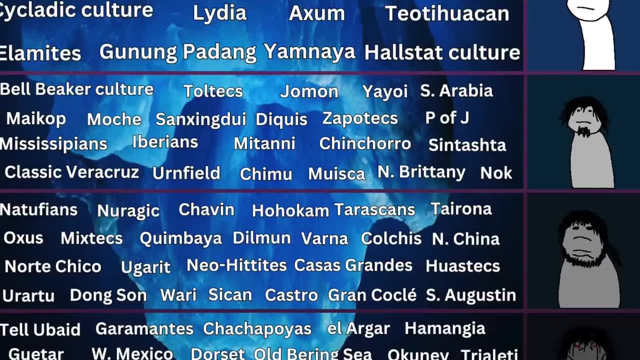 I try to cover every civ as quickly as I can, but I try to give as much of a rounded view as possible And generally I try to cover why I put it where it is, what its most impressive monuments and achievements are, the mark it's made. 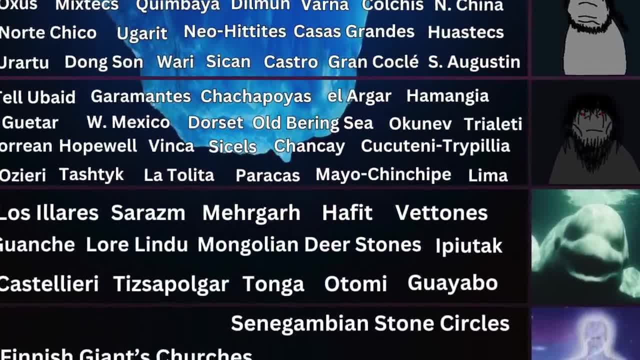 and what we know about it. I don't know if you guys know about its rise and fall, which is usually not that much fancy aggressiveness, and then when you back, it's a problem, you know. but there are still whole civilizations, so don't expect me to do them complete justice. 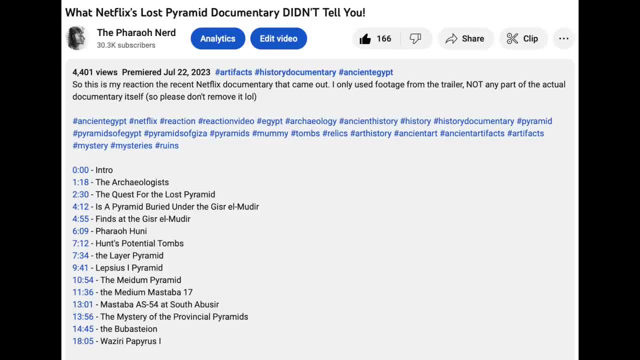 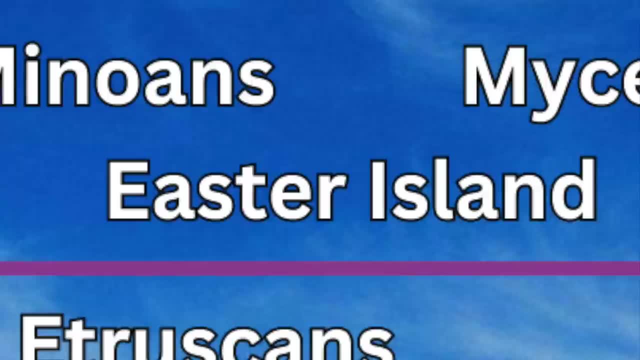 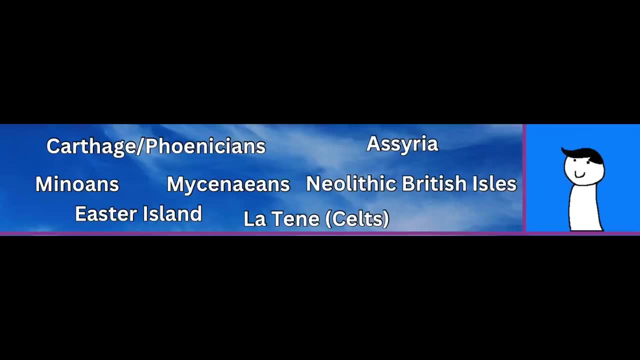 And ultimately, that's why this video is so long. so I would personally recommend using the time stamps I hopefully put in to skip around in order to find the civilizations that most intrigue you. Level 1 is filled with civilizations that most people interested in history or archaeology are already aware of. It's just that they're not as famous as civilizations like ancient Egypt. They need more research and guidance and think about how they can better help each other. So if you think You know, if your history can support that and you kind of decide what kind of civilization you want to go with, that's when you might see these kind of civilizations. 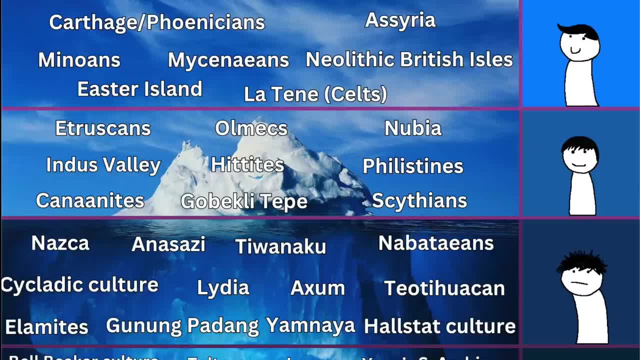 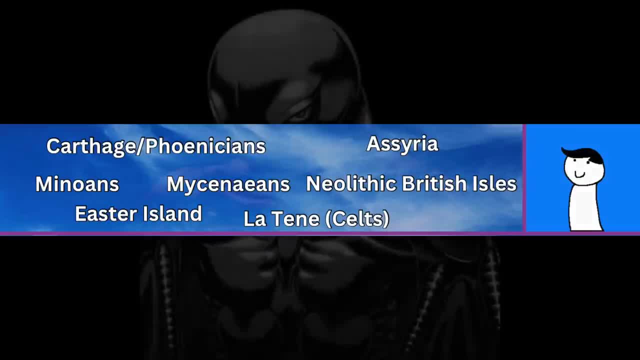 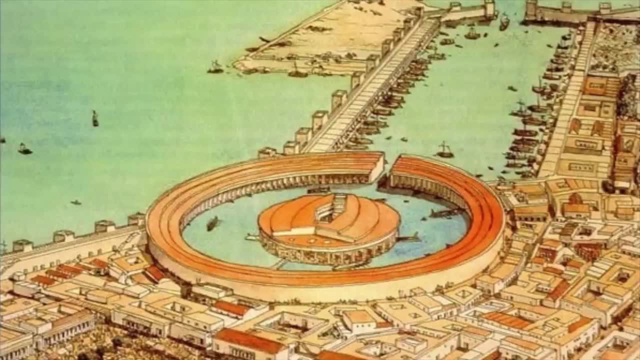 Look for tutorial and information or classical Greece. so that's why they're above the iceberg and next to this jolly chap. That's also why my descriptions aren't as descriptive as the ones I made for the civilizations which are more obscure and further down the iceberg. Carthage, slash the Phoenicians. I put Carthage. 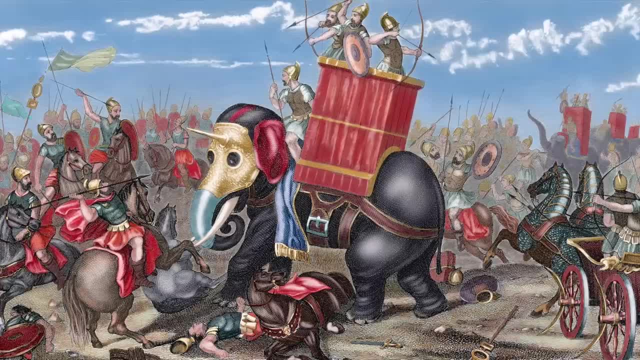 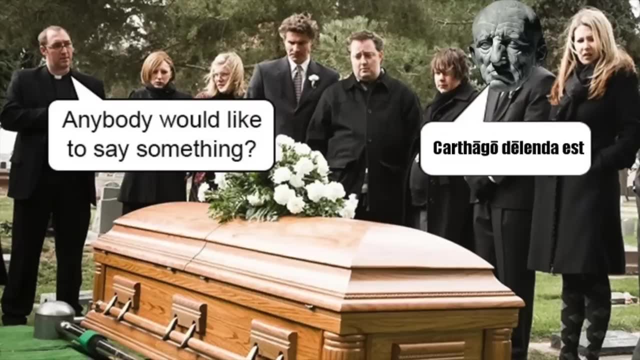 all the way up here, because if you're at all familiar with Roman history, you probably know about Carthage because of the Punic Wars, and that's why 14-year-olds think spamming Carthago de Lenda Est on history memes is somehow funny, and Hannibal Barca is probably. 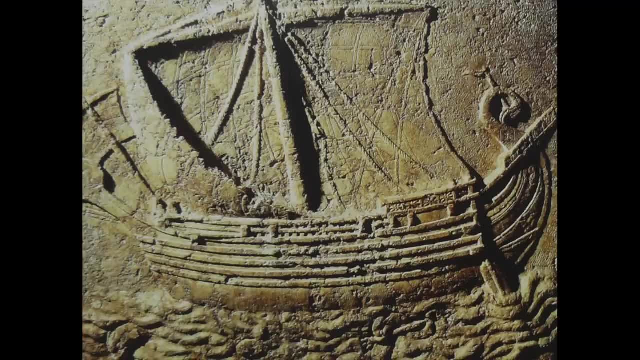 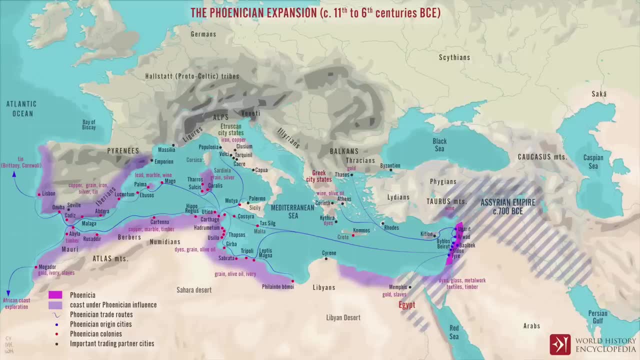 one of the most famous military geniuses in history. The Carthaginians and the Phoenicians as a whole were very mercantile people who flourished in the Iron Age and colonized a huge chunk of the Mediterranean in search of profit, including much of the coast of North. 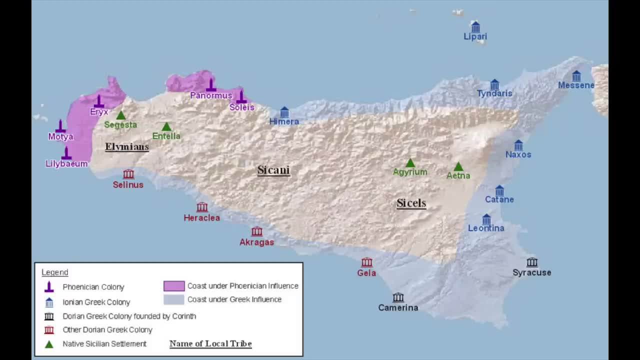 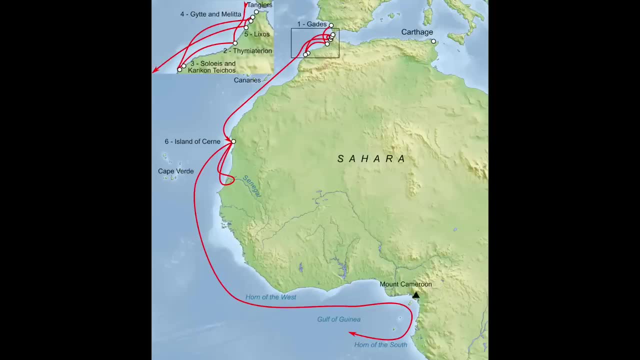 Africa, parts of Spain, the Balearics, Sardinia and Sicily. This was made possible by their seamanship, exemplified by the fact that they explored far-off regions of sub-Saharan Africa in a contingent way. A contingent of them possibly even circumnavigated the whole continent. on behalf of the 26th. 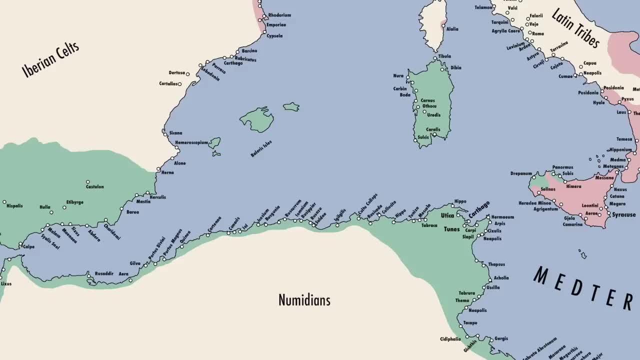 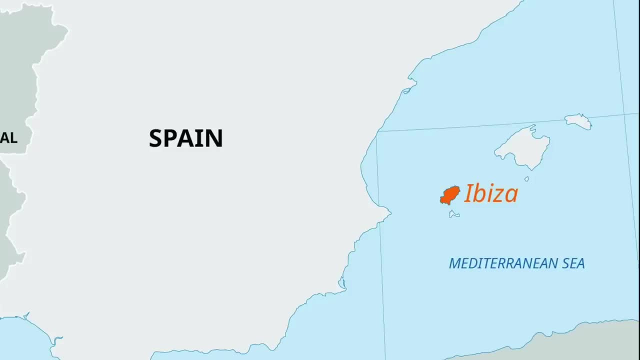 dynasty Egyptian pharaoh Necho II, And some of the names they gave to the places they encountered are still in use today, like Cartagena, Cadiz and Ibiza, which they named in honor of the Egyptian god Bess, because Phoenician culture was heavily influenced by Egypt. They're 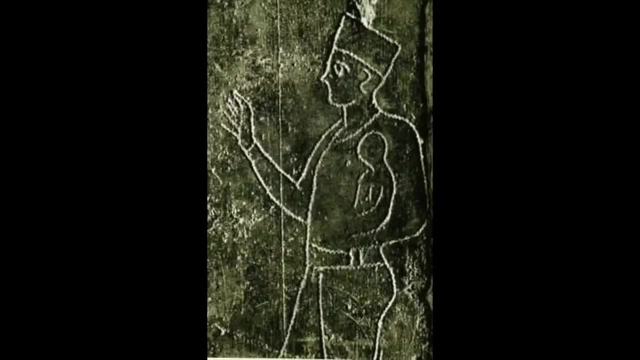 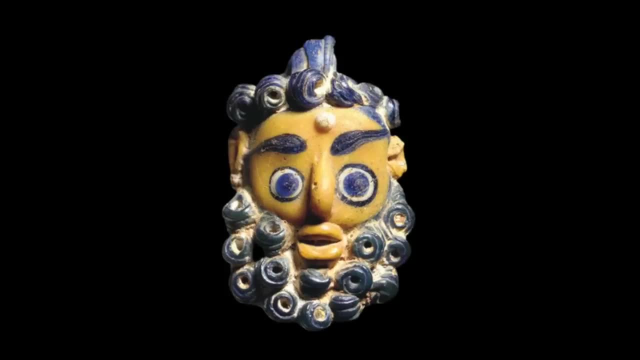 also notorious for sacrificing their own infant children to their gods and burying them under stelae in cemeteries known as tophets. I included the Phoenicians and Carthaginians together because the Carthaginians were just an offshoot of the Phoenicians that left their homeland. 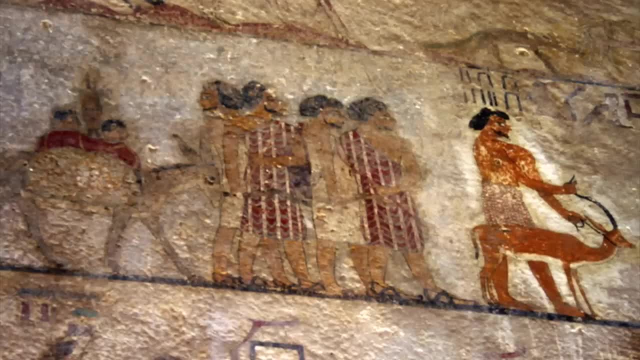 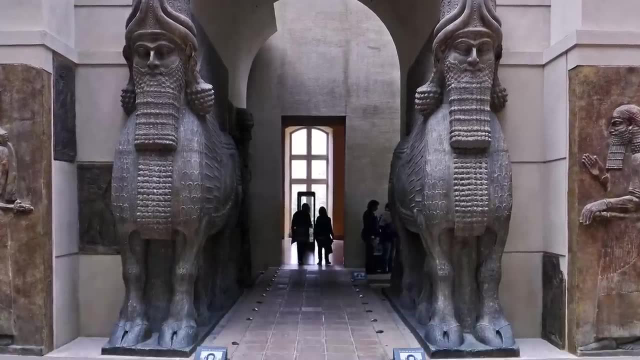 in the Levant and in reality, the Phoenicians as a whole were just a form of Canaanite, which we'll get to later. Assyria: Assyria is pretty well known, especially since it conquered pretty much the entire Near East. 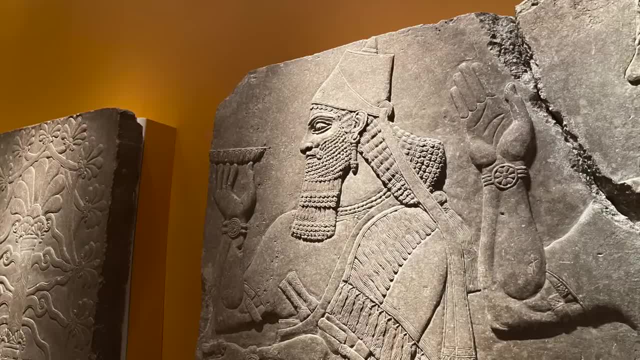 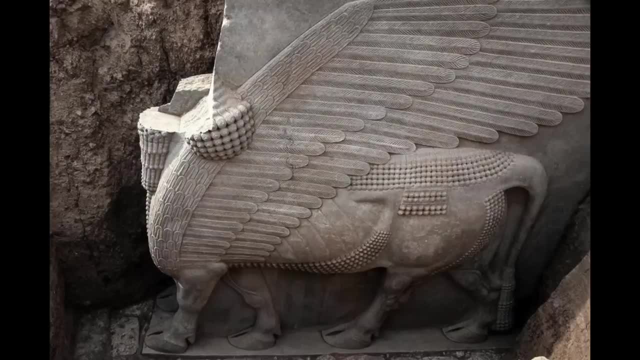 even including Egypt, between the 9th and 7th centuries BC. The imposing very finely cut reliefs and human-bull hybrid gate guardians, or Lamassu, that once decorated their palaces at sites like Nimrud and Nineveh can be found in various museums around the world, Apparently. 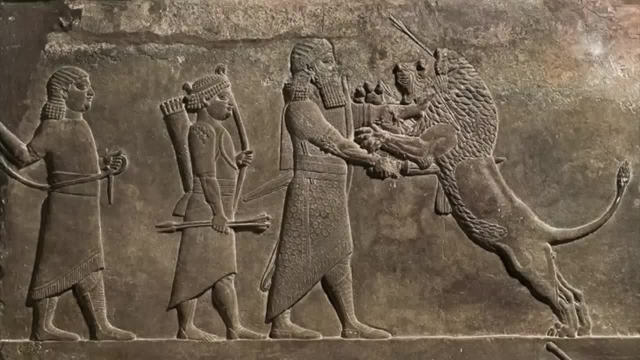 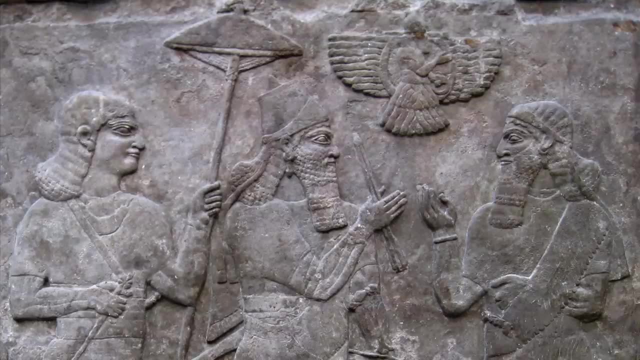 they were meant to make foreign ambassadors shit themselves in awe at the king's power, and after seeing some in person at the Brooklyn Museum, I can see how they'd react like that. The version of the Assyrian state that dominated the Near East is known as the Neo-Assyrian. 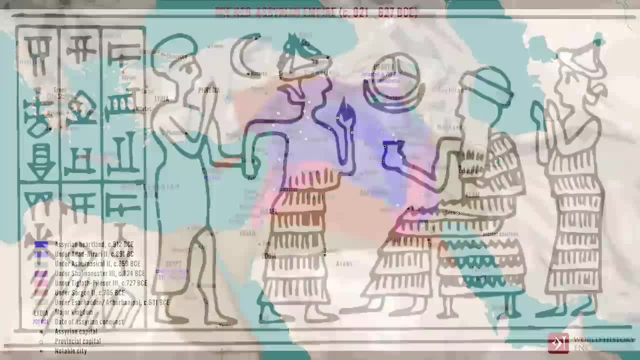 Empire because it was the fourth version of Assyria, which began as the city-state of Assyr around 2025 BC and did pretty well for itself throughout the Bronze Age. They're also pretty well known for conquering the ancient Kingdom of Israel and for conquering 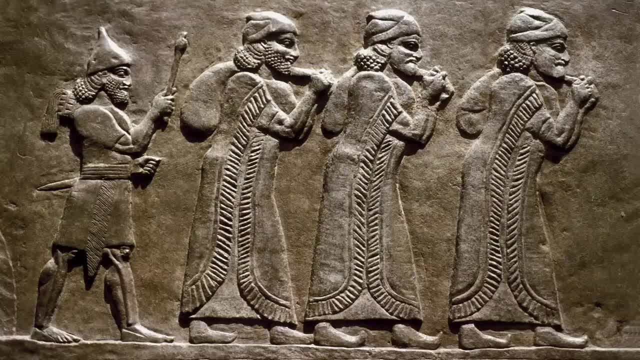 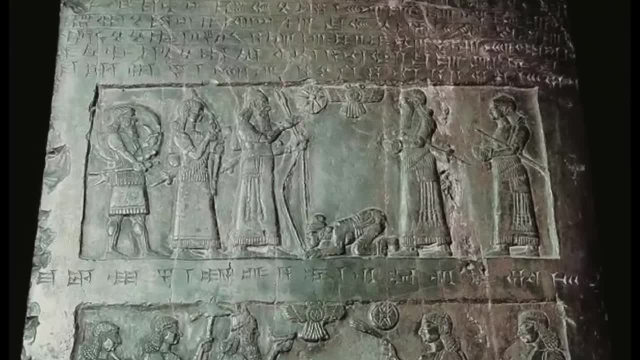 the ancient Kingdom of Israel And resettling the tribes living there, which became known as the Ten Lost Tribes. But ironically they're like the most important non-biblical source on the Israelites, as well as the earliest Arabs And a whole bunch of other people But the non-Assyrians who lived under the Assyrian boot, like the Chaldeans who would soon take over Babylon and the Medes hated them. So they all revolted at once and the empire collapsed really quickly, with Assyr falling in 614 BC. But the Assyrians still existed as a people and they even have their 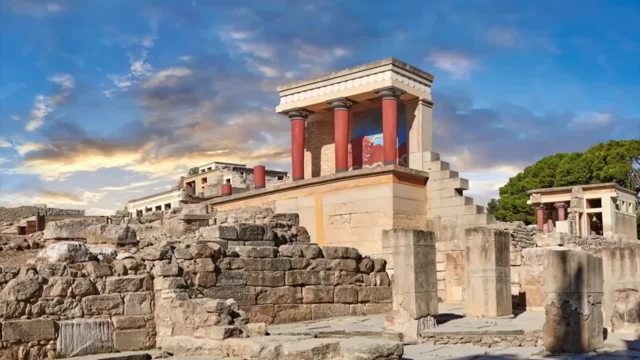 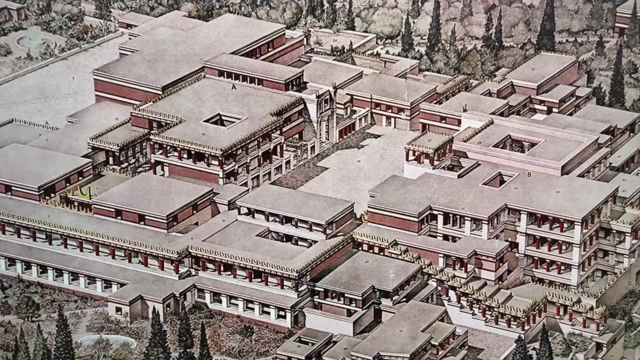 own church. Minoans, Famous for being one of the first real civilizations in Europe and precursors to ancient Greece, the Minoans inhabited the island of Crete and built huge, multi-story palace centers, like the ones at Knossos and Phaistos, covered in amazing frescoes, which 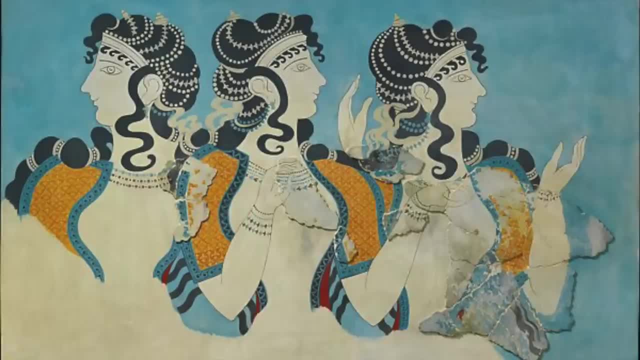 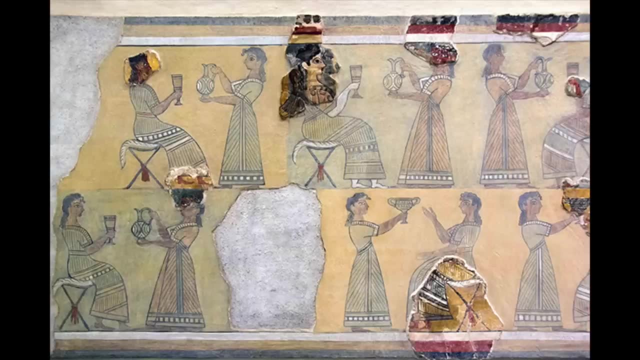 are unfortunately usually pretty fragmentary, Which you might not realize, since most have been heavily, heavily restored stuff done for the guy who basically discovered the Minoans, Sir Arthur Evans, But it's still pretty controversial among scholars: They're called the Minoans. 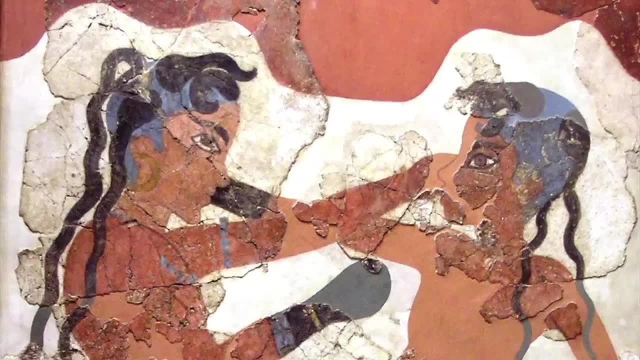 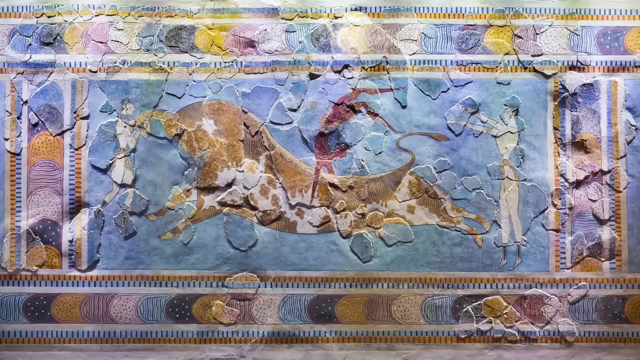 because they were around at the same time and place at which the legends of King Minos and the Minotaur's labyrinth are set. Anyways, it makes sense. They were obsessed with bulls and from their frescoes we know that they even held bullfighting tournaments, like the. 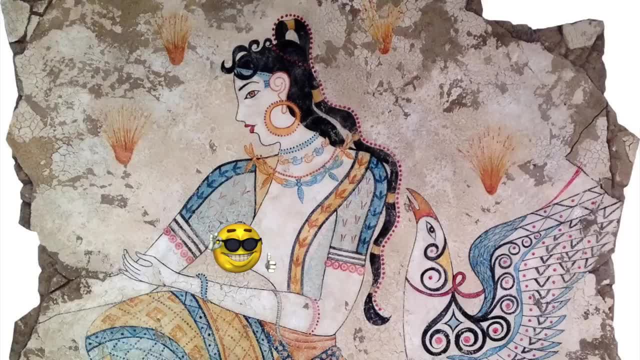 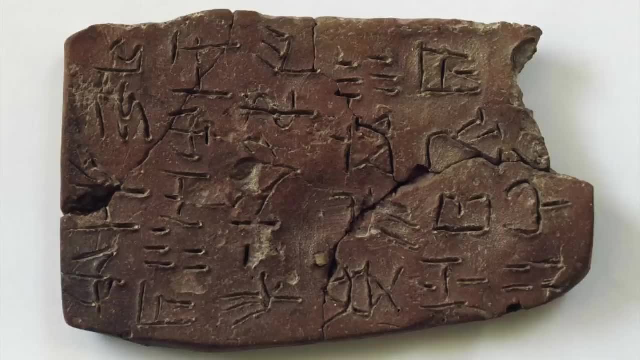 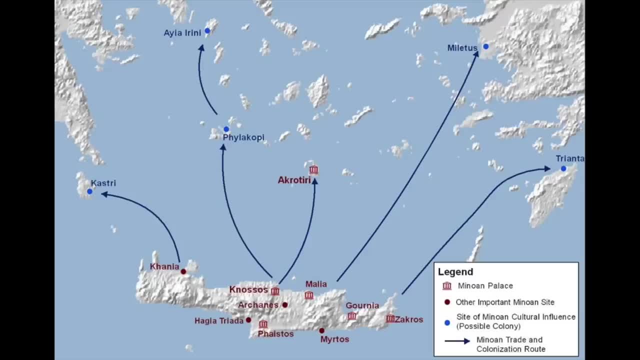 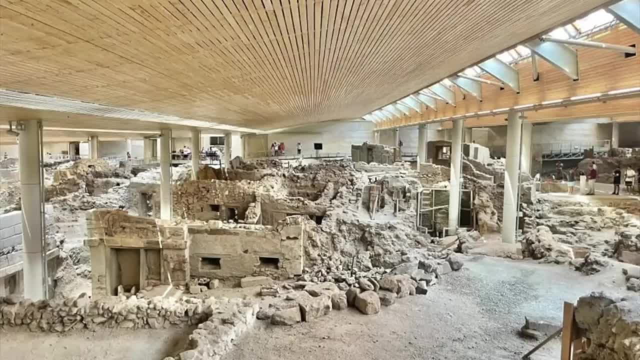 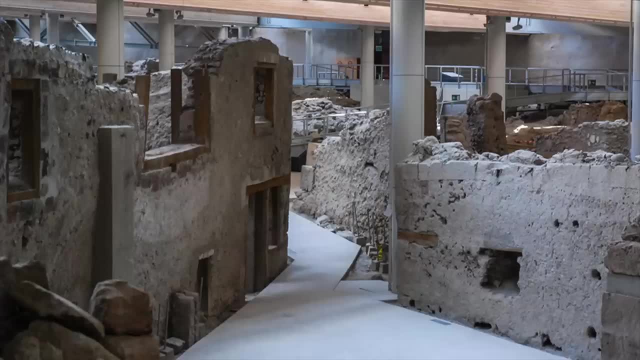 to it Well, a huge volcanic eruption And the settlement that the Minoans built there, Akrotiri- filled with beautiful frescoes, by the way- was buried in ash. But luckily, unlike at Pompeii, its citizens had ample warning and escaped just in the nick of time. 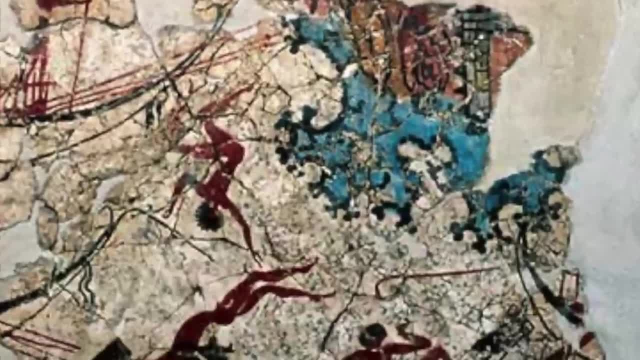 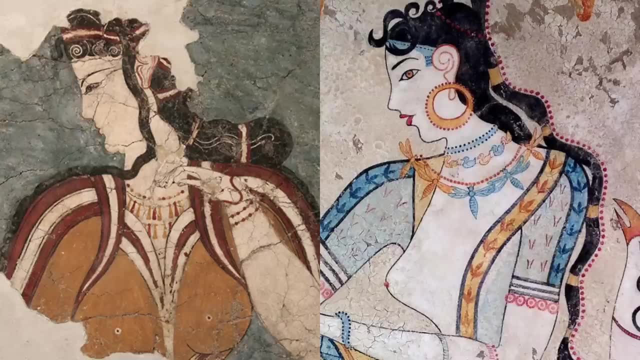 it might have contributed to the downfall of Minoan culture, which also involved Mycenaeans. The Mycenaeans and Minoans come as a pair. You can't know about one without finding the other. Their major sites include Mycenae, obviously, Pylos, Tiryns, and they even had a presence at 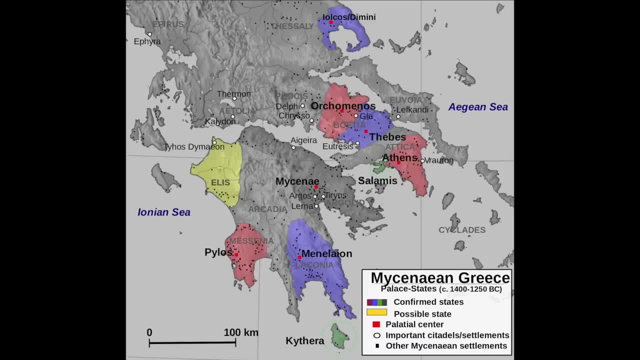 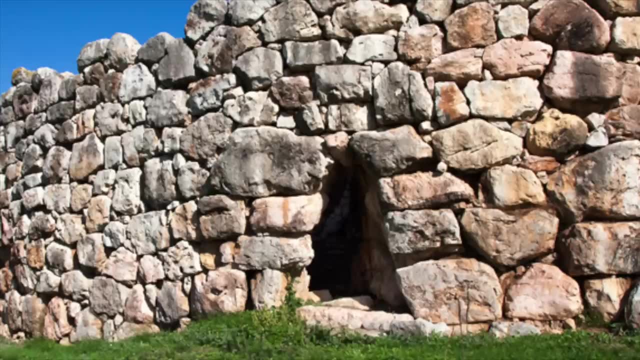 Athens and Thebes. Like their classical successors, they were also split up into various city-states. They were big fans of what's known as Cyclopean Masonry, where they'd fit huge limestone boulders roughly together, which they used to build the walls of their palace centers and which later. 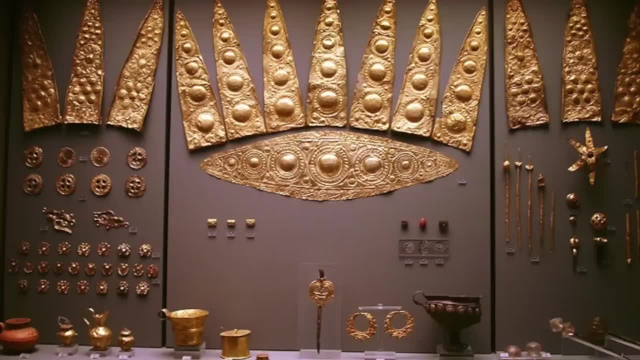 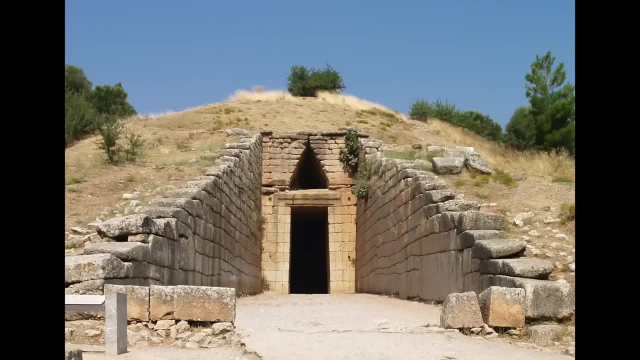 Greeks considered the work of Cyclops. They also buried their elites in richly furnished tombs, which were often these huge structures shaped like beehives, known as Tholos tombs, like the magnificent treasury of Atreus at Mycenae. But the most famous artwork of theirs has to be the. 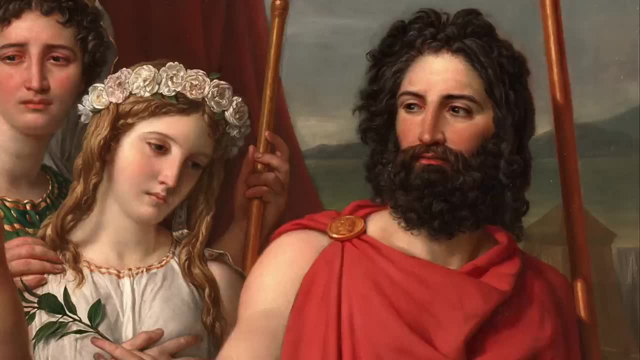 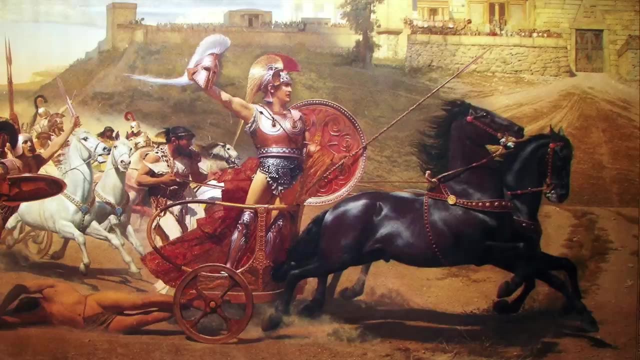 so-called Mask of Agamemnon, attributed to the ancient king of Mycenae who figured prominently in the Iliad, But unfortunately it dates to the 16th century BC, so predating the Iliad. but I totally get it. 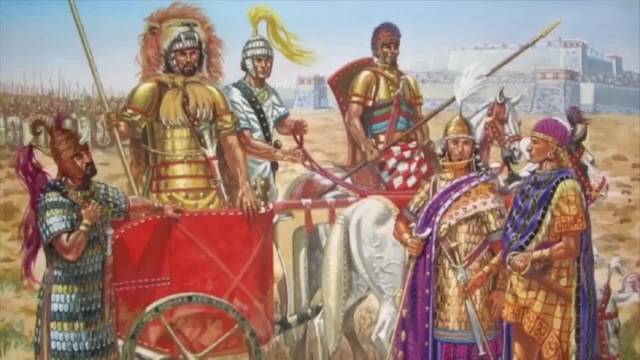 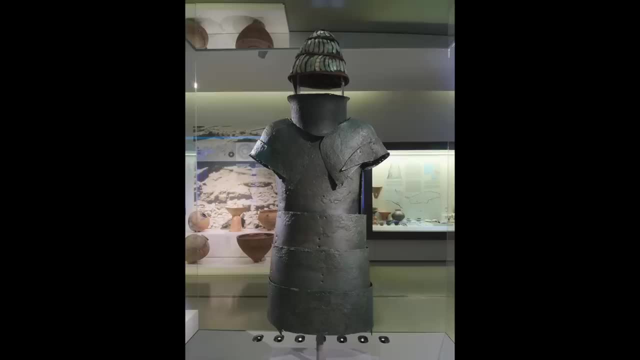 the urge to assign a name to the face. That's because these are the people who would have fought in the Trojan War, and that urge to find those ancient heroes led to the discovery of their civilization in the first place. They also had really cool armor, like this: 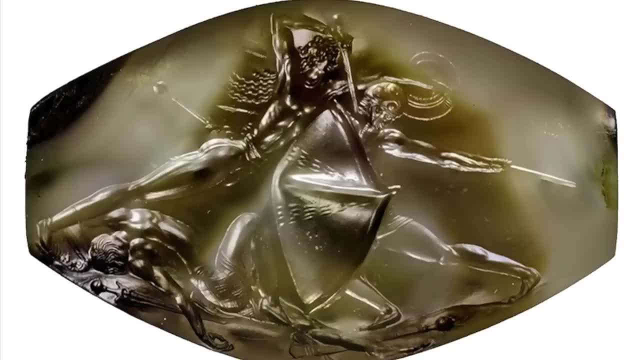 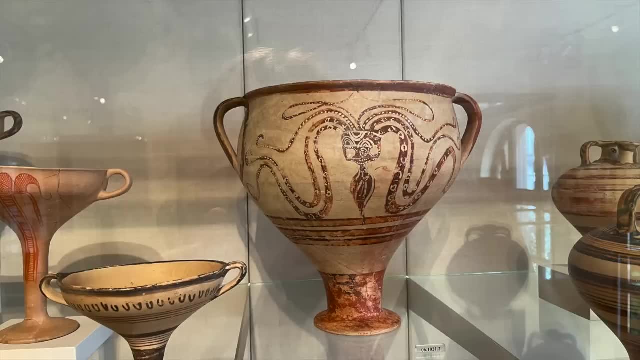 bronze panoply and their boar tusk helmets. In addition, they carved really, really intricate little designs into their signet rings and gems, and I personally really like the octopi they painted on their pottery. Around 1450 BC they seemed to have conquered Crete and eventually Minoan culture was a. 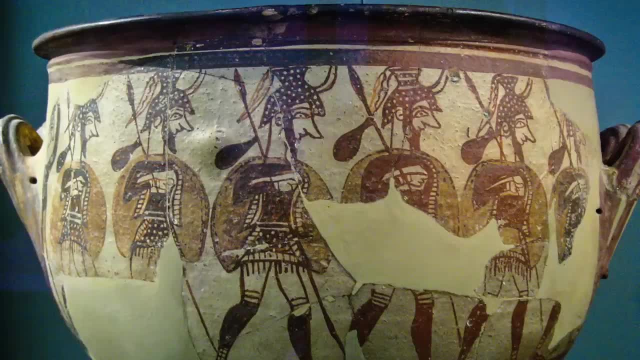 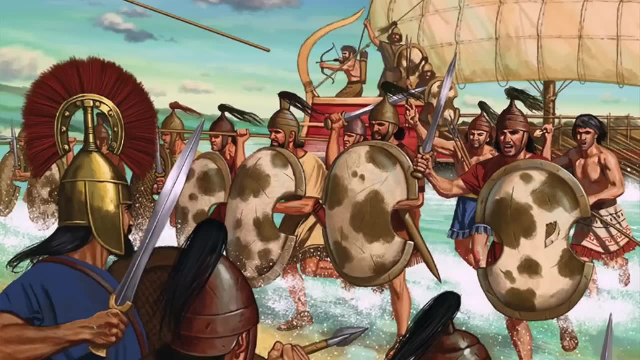 part of their civilization. But soon enough they collapsed themselves and like any good civilization, we have no fucking idea why. Maybe it was earthquakes, maybe it was new people coming in, maybe they became part of the Sea Peoples which pillaged the rest of the Eastern Mediterranean and brought other civilizations down with them. Who knows Neolithic British Isles? These are the guys who made Stonehenge, so by virtue of that, these guys aren't too obscure. You might think it's odd of me to include them, since they lived in the Stonehenge. 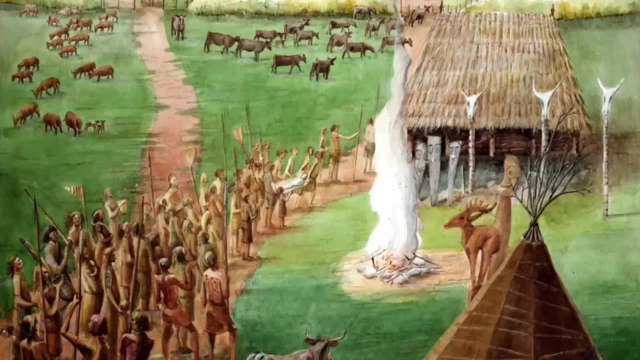 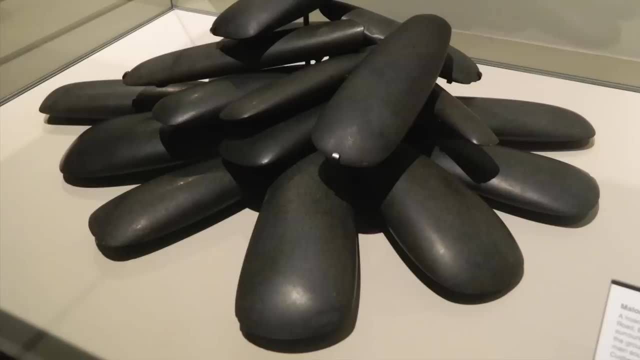 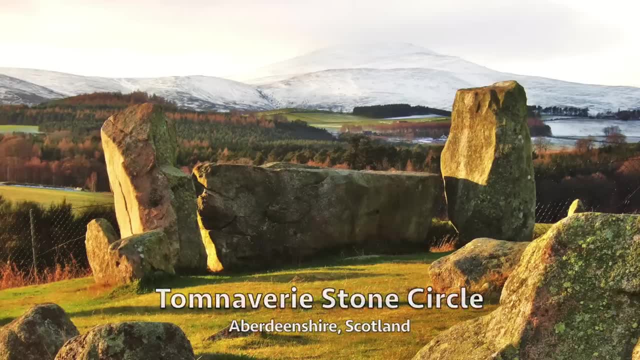 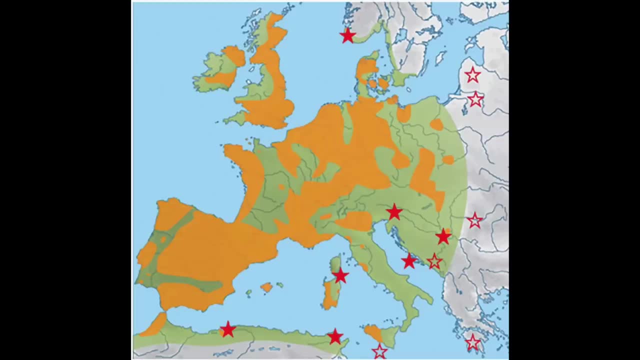 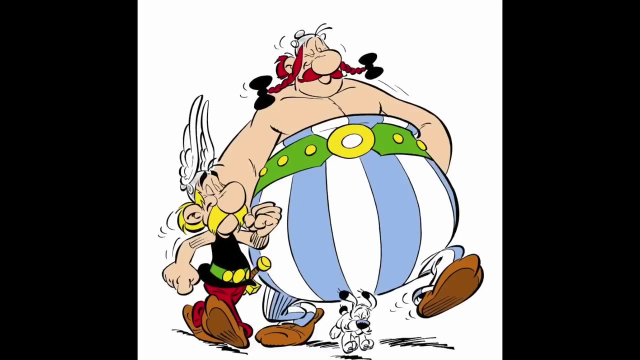 they built huge passage tombs like Newgrange and Noath. It's just unfortunate their fate wound up somewhere in between being totally wiped out or being totally assimilated in to the Bronze Age culture that came after them. La Tène is just the fancy archeological term for the Late Iron Age Celts. Think Asterix. 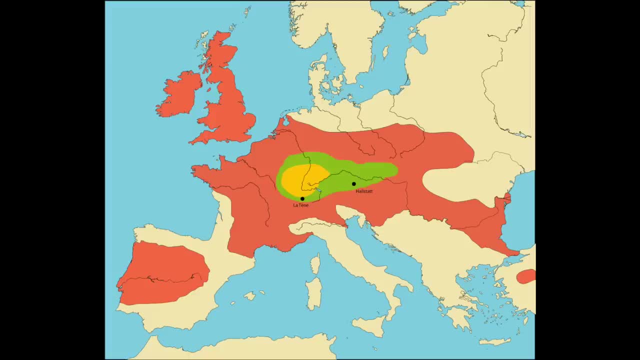 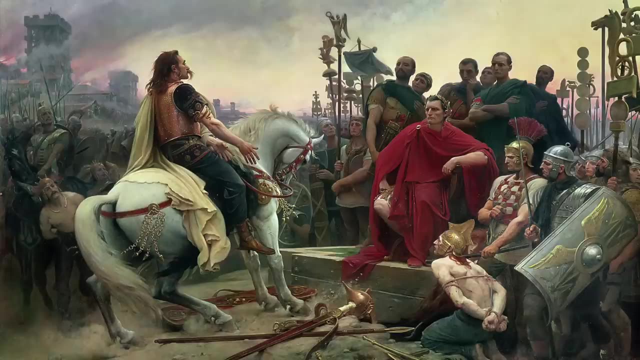 and Obelix, Once widespread across Europe and even setting up shop in the Centre of Anatolia. of all places, these fierce torque bearing, ever nude warriors fought hard against but were ultimately defeated, conquered by the Romans, like Julius Caesar, of course, except in fiercely independent regions. 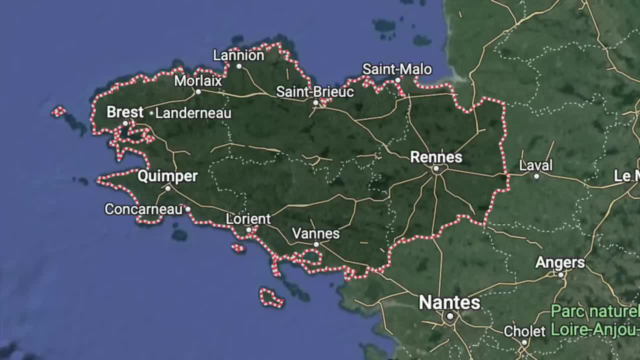 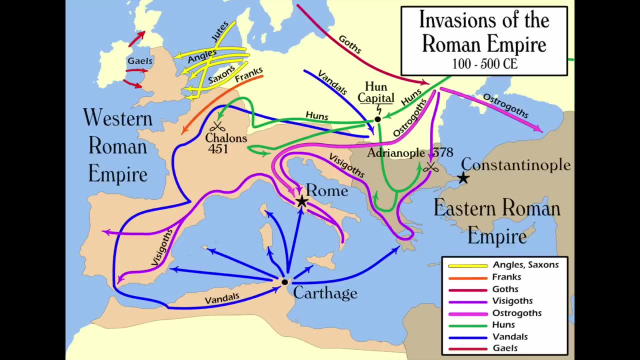 like Scotland and Ireland. People from there and from places like Brittany, Cornwall, Wales and the Isle of Man are still incredibly proud of them being the last bastions of Celtic culture, as they managed to hold out, at least ethnically, against the Germanic peoples who overran the 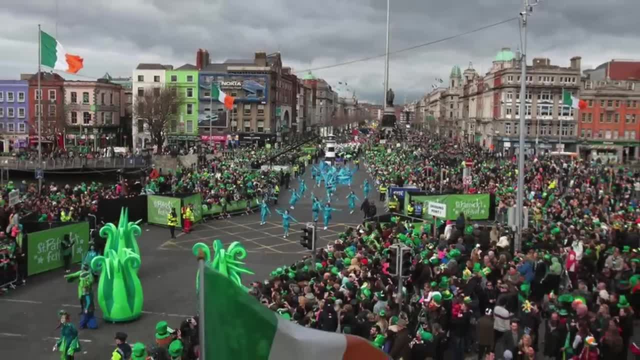 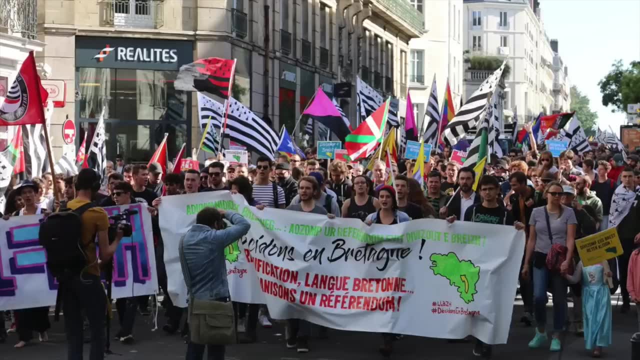 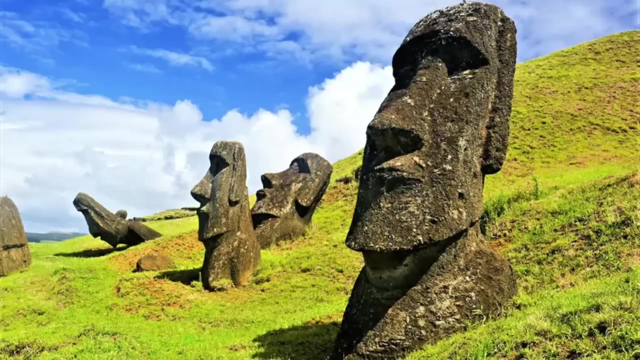 Romans, Because so many people like myself are descended from Celts and proud of it, and the desire to preserve Celtic languages and ways of life were and are such big deals in Celtic countries. I couldn't put them any lower on this list. Easter Island: Everyone knows about the big 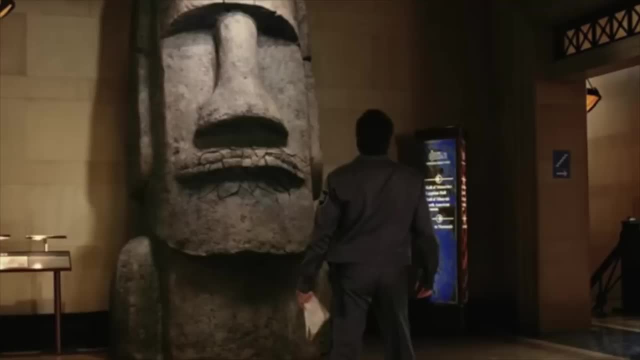 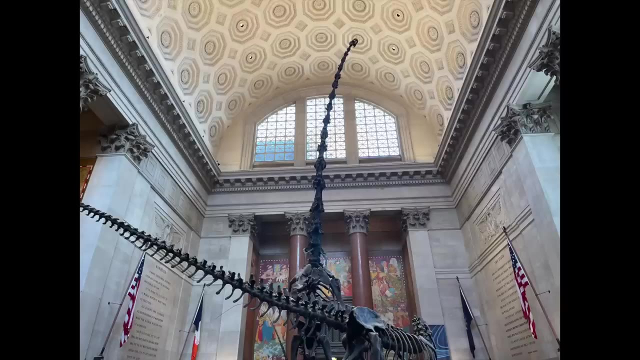 Moai heads on Rapa Nui, also known as Easter Island. Everyone remembers Gum Gum from Night of the Museum and I actually got to see him in person at the American Museum of Natural History recently, so that was pretty cool. Unfortunately for me and fortunately for the modern people. 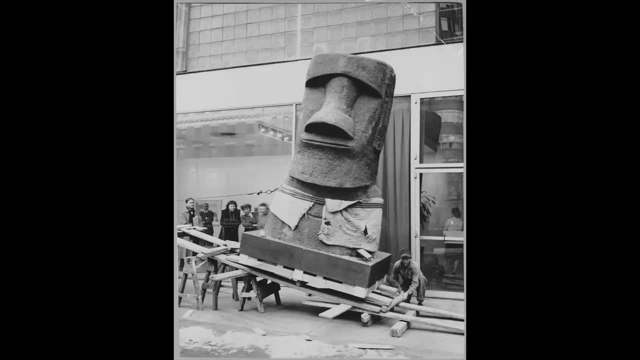 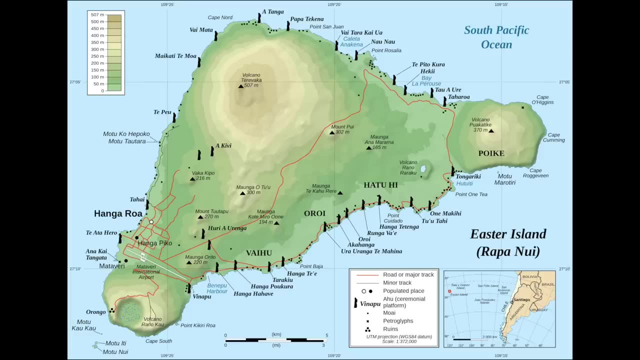 of Rapa Nui. it's actually just a plaster cast of an original, Not the real deal. No one knows what possessed the islands and inhabitants to make so many of these enormous stone statues- nearly 900, to the point where they may very well have stripped the entire. 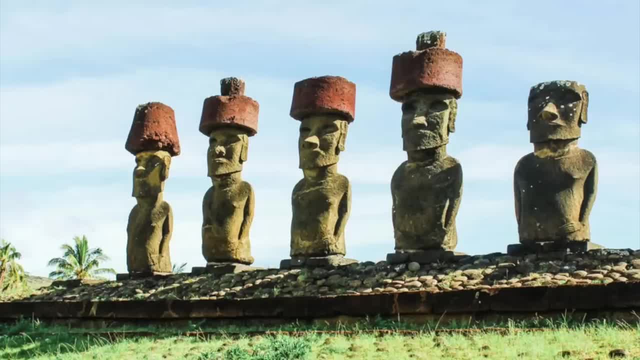 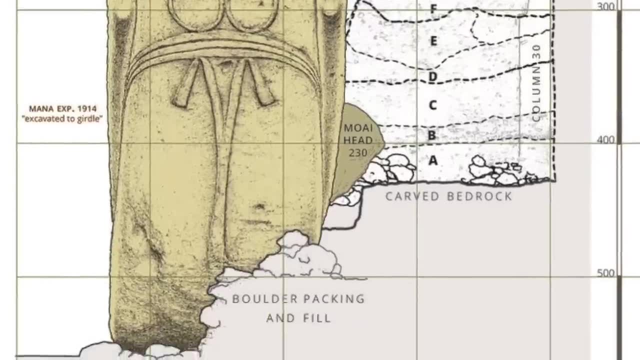 island of all its trees. but I mean, come on, they were damn good at it. And it's becoming more well known that they aren't just heads. Some have incredibly long bodies with petroglyphs carved into them, Some also had inlaid eyes made of coral and some have red top knots. 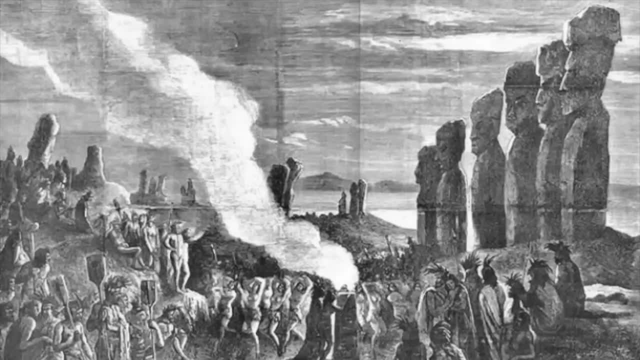 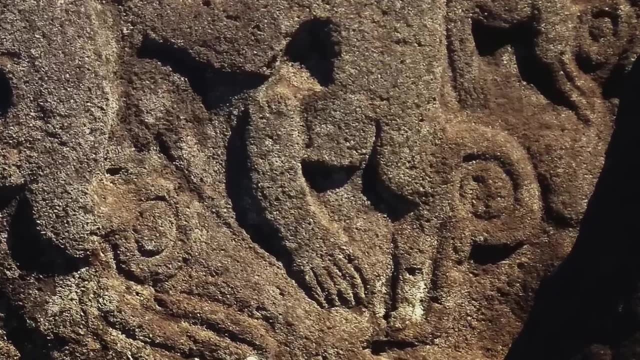 called pukao. The tradition of making Moai, which lasted from 1100 to 1650, roughly, might have been replaced by something called the Birdman Cult, which involved this deadly competition where people had to dive into the ocean from the top of an incredibly 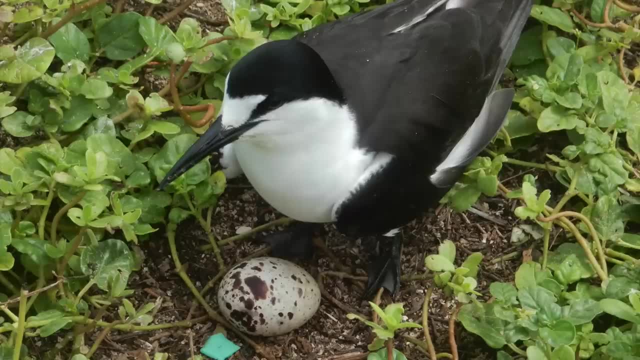 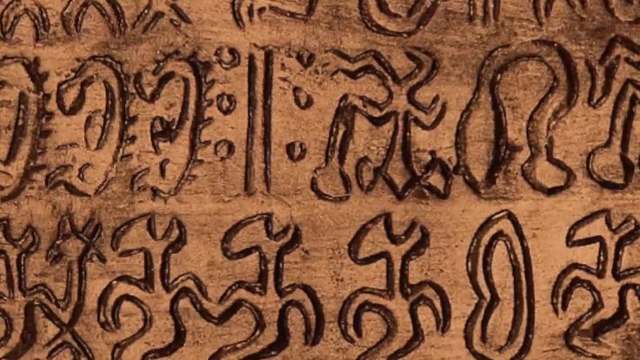 high cliff, swim to a nearby island, collect the very first egg of the bird mating season and then come back with it, alive, hopefully. They also had a totally unique writing system called rongo rongo, mostly written on wood, which still hasn't been deciphered to this. 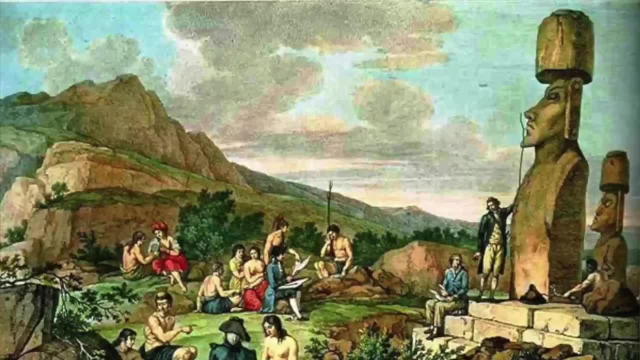 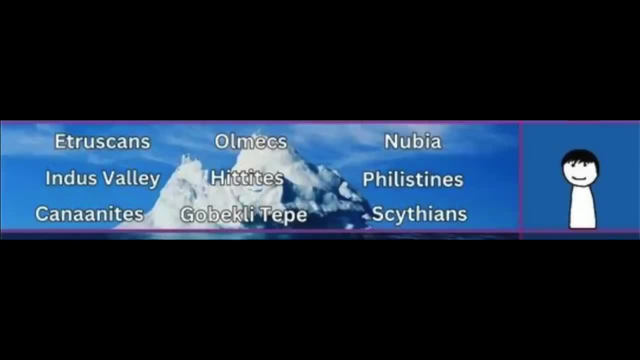 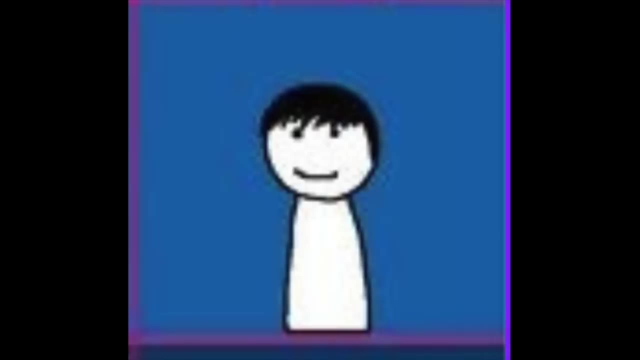 day. Unfortunately, the island was devastated by contact with Europeans and almost all the Moai had been toppled by 1868.. Second Level: Okay, so we're finally on the iceberg itself now. So these guys are still relatively well known. Just look at the guy next to it. He looks… fine. 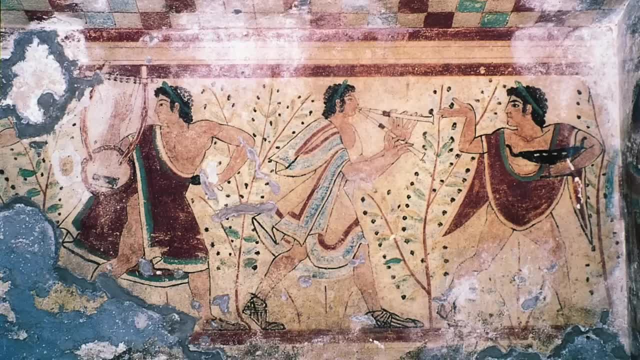 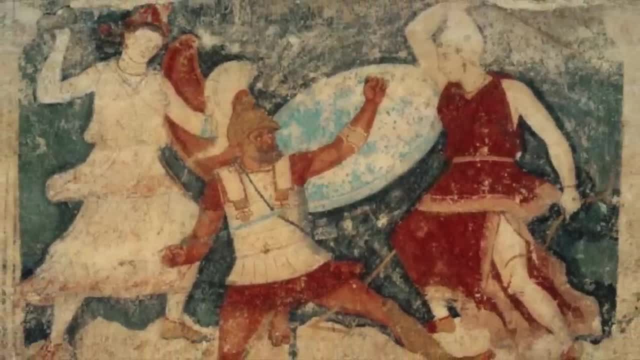 The Etruscans. The Etruscans figure prominently in the early history of Rome, given their dominance over northern Italy from around 700 BC until they were eclipsed by Rome itself in the 4th century BC And, according to legend, Rome's last three kings. 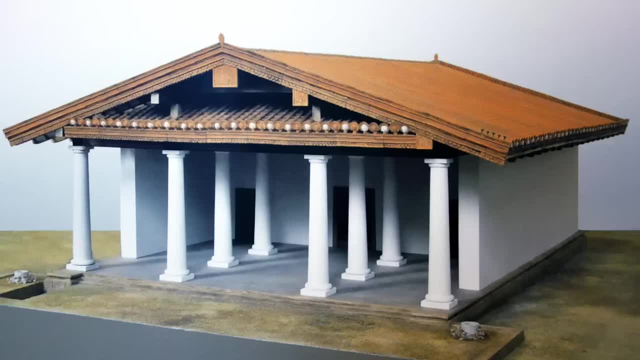 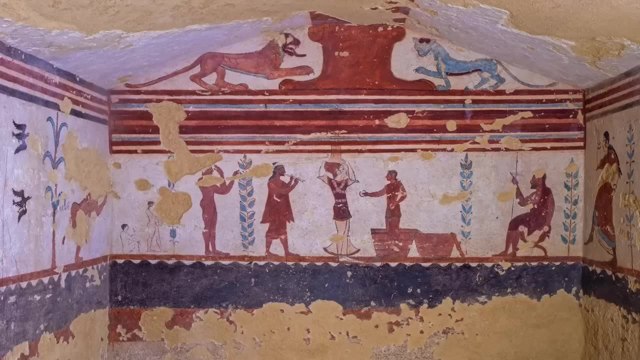 were Etruscans, so of course they heavily influenced Roman culture. They left behind some pretty spectacular art, like their lively sarcophagus effigies, their vividly decorated rock cut tombs, like the ones at the necropoli of Monterosi and Banditacea, and superb bronzes. 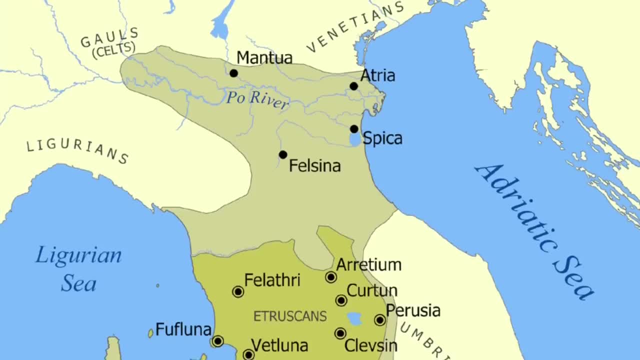 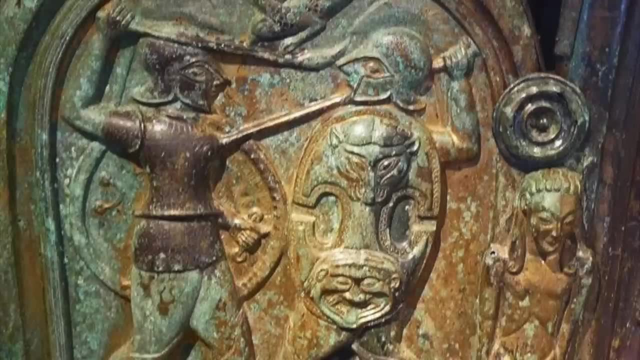 like the Chimera of Arezzo or the Mars of Todi. As you might have guessed from the names, they were divided up into a number of independent city-states that cultivated fierce rivalries between one another, but they also formed a loose confederation known as the Deceit. There were also a number of cities that were 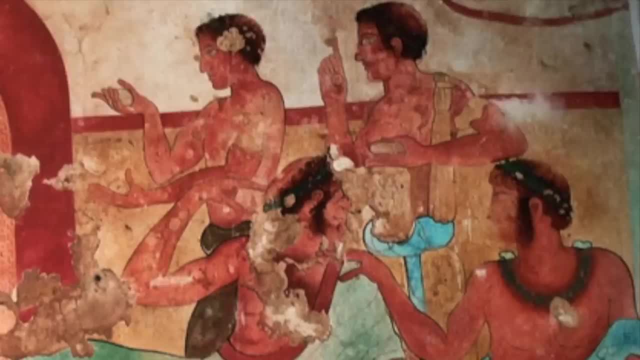 divided up into a number of independent city-states that cultivated fierce rivalries between one another, but they also formed a loose confederation known as Deceit. The Deceit was the League of Twelve Peoples. to promote their common goals, They also established 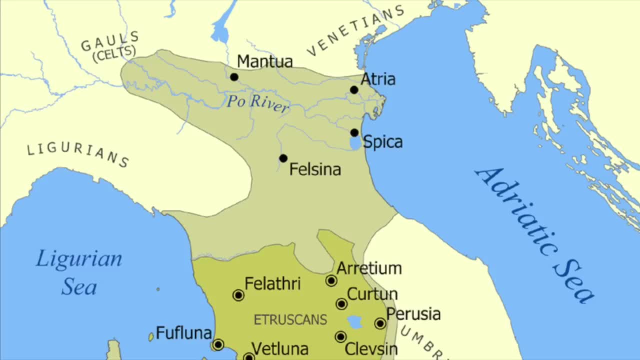 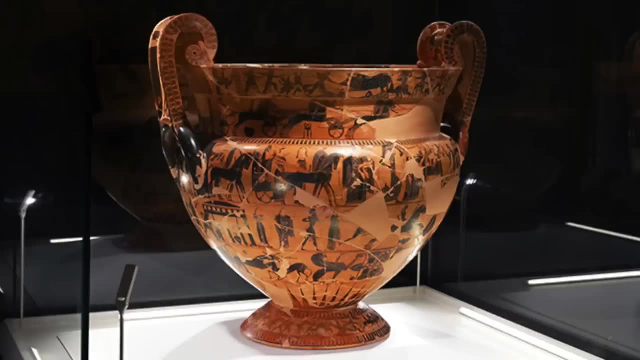 colonies all across Italy, from Campania in the south to the Po Valley in the north. Their art was, of course, heavily influenced by the Greeks, and they imported tons of Greek luxury goods, but, as you can see, they added their own really distinct flair to it all. They 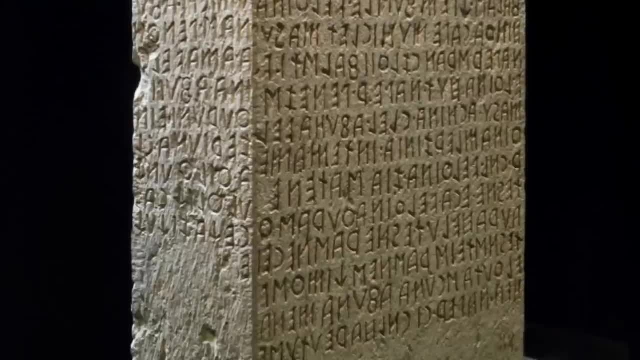 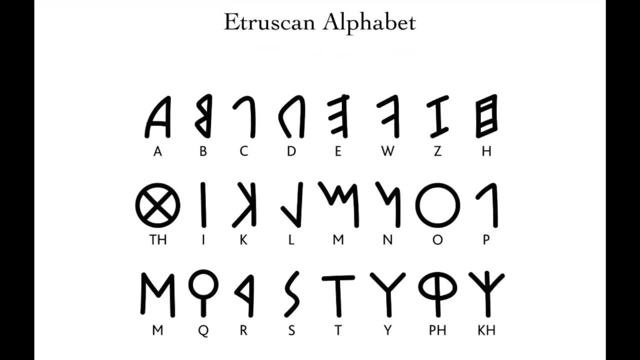 spoke a pre-Indo-European language and wrote using their own distinct alphabet taken from the Greeks, and it just so happens to be the direct ancestor of the Latin alphabet we still use to this day. I'm proud to say that I spotted this in the early 1800s. 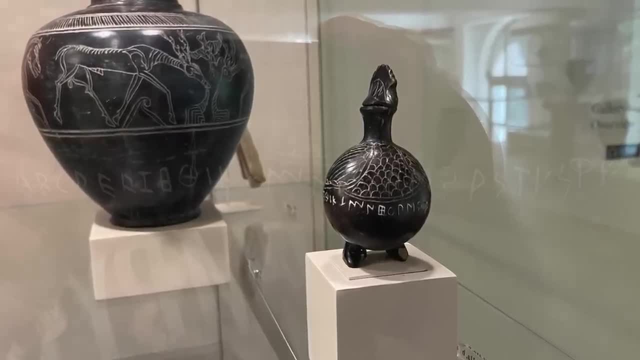 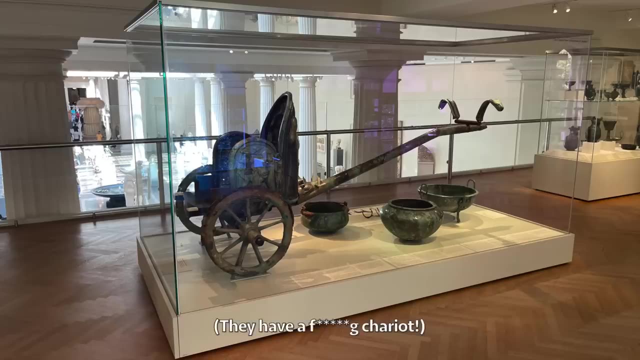 Let's not take a minute and say that. I spotted this little 7th century bottle statuette, inscribed with their entire alphabet and on Wikipedia, in the corner of a display case in the Met which has an amazing little sub-floor partially dedicated to them. Despite that, the Etruscan language still hasn't been fully deciphered, Partially because of how unique their language was. Their origins were hotly debated in antiquity and a lot of historians championed the idea that they were Lydians who had left Anatolia due to. 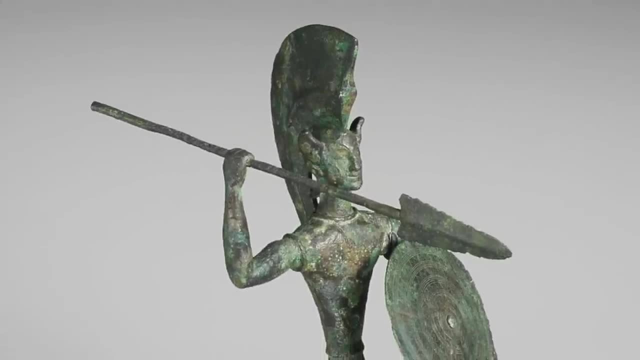 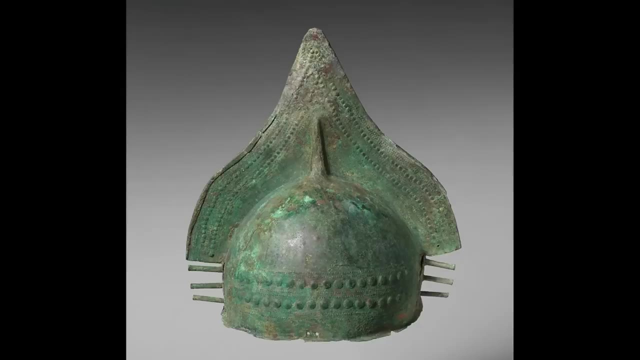 a famine, but in reality we know that they were probably indigenous. So thank you for watching. and emerged from the earlier Villanovan culture, which is also sort of seen as the first phase of Etruscan culture. They also had really cool helmets. 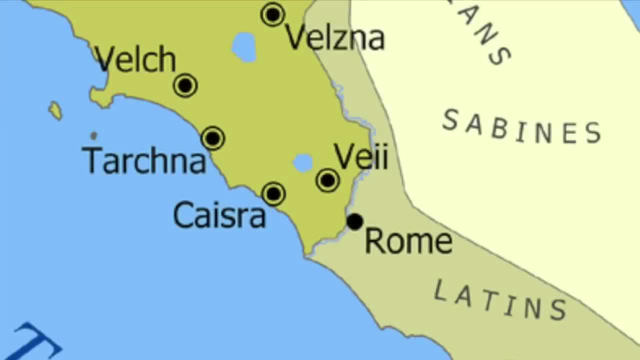 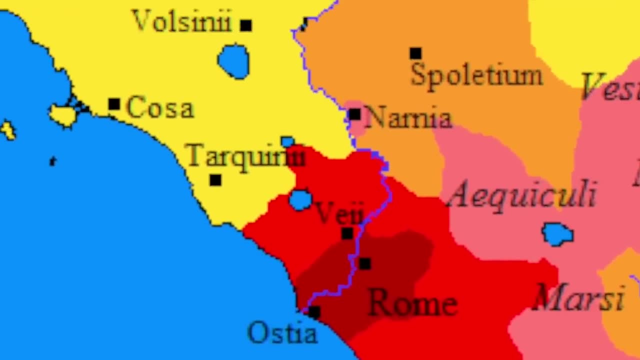 Eventually, the Etruscans were totally superseded by Rome. They conquered their first Etruscan city, Veii, in 396 BC, and just over a century later, in 264 BC, they conquered the last independent Etruscan city-state, Volsini. 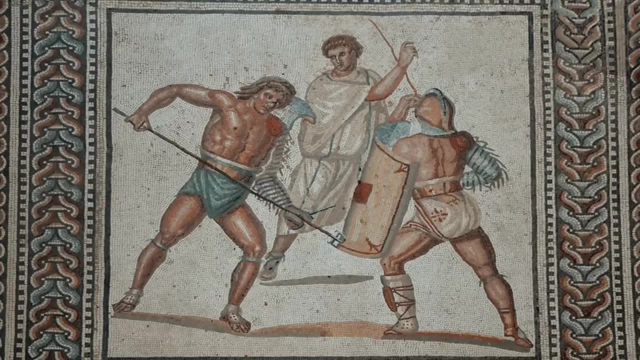 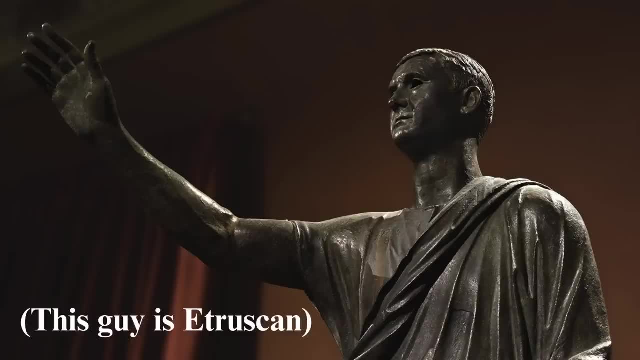 And some of its citizens found themselves participating in the first ever recorded gladiatorial game held later that same year. But eventually they became citizens of Rome during the Social War in 90 BC, The Olmecs- Anyone who's delving into ancient Mesoamerica. 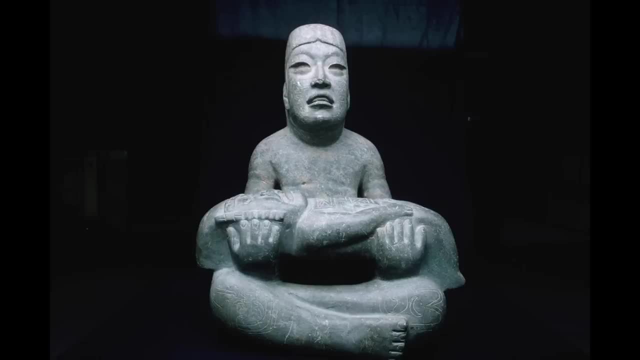 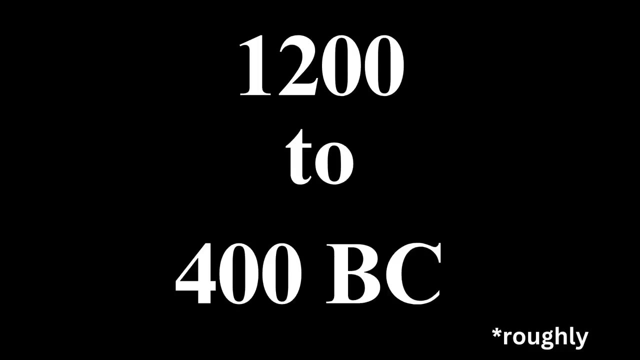 is gonna come across the Olmecs sooner rather than later, because it's Mesoamerica's mother civilization and it lasted from 1200 to 400 BC. in Mesoamerica's formative period, Their three major cities were near the Gulf Coast of Mexico. 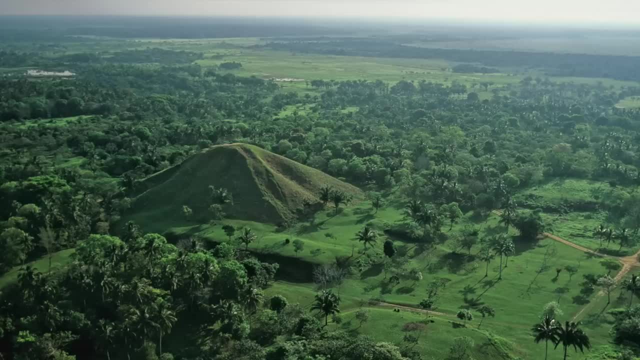 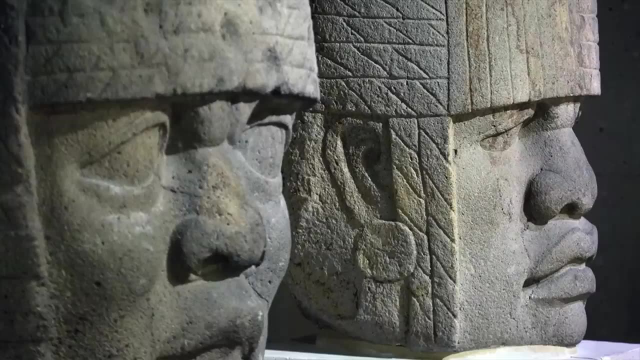 in the states of Tabasco and Veracruz, San Lorenzo, La Venta, where they built a huge pyramid called the Great Pyramid, and Tres Apotes. They're best known for making colossal stone heads, possibly representing their rulers, and they were very, very skilled sculptors in general. 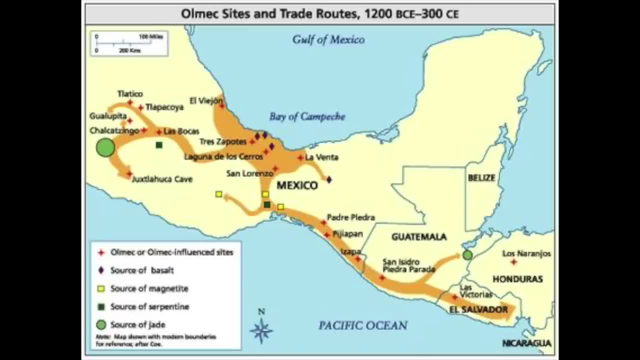 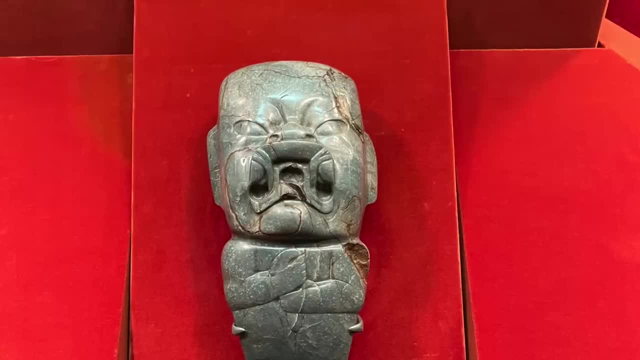 They were also really good at working with jade from really far off mines in the Guatemalan highlands which they used to make masks which you might recognize from a certain anime, and votavaxes bearing the likenesses of one of their chief gods. 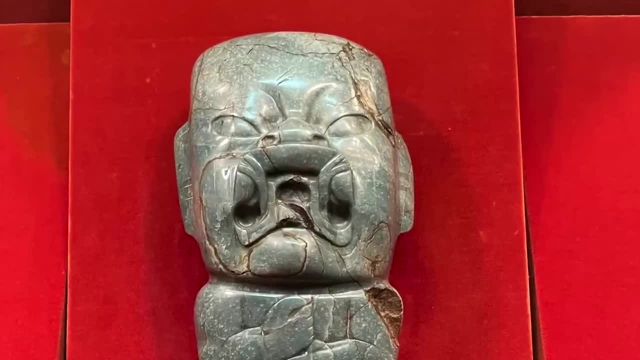 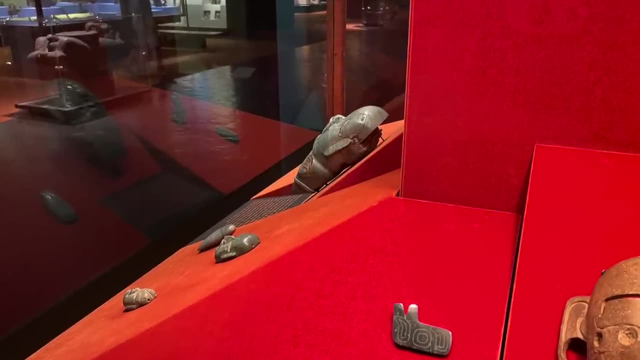 a bizarre hybrid between a chubby human baby and a jaguar. It was really weird to see one in person at the American Museum of Art, and you can see that chunks had been taken out of it by later peoples as souvenirs, and the masks as well were highly prized by later civilizations. 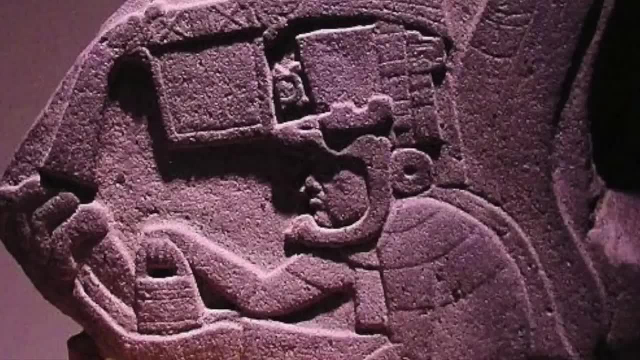 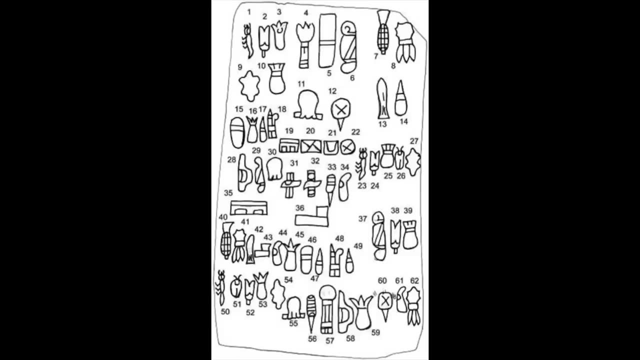 They started a bunch of Mesoamerican traditions that would survive long after they disappeared, like the Mesoamerican ball game and bloodletting, and they may have even invented the first writing system in the Americas, based on the Cascayal block and other finds. 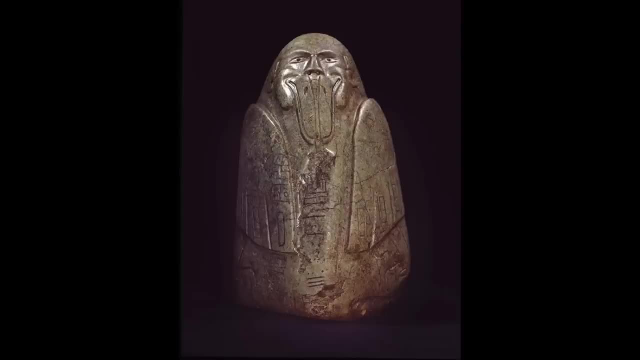 as well as an enigmatic script known as the Isthmian script, which may represent the intermediary between Olmec and Maya glyphs. Their immediate successor, the Mesoamerican script, is the Mesoamerican script, which may represent the intermediary between Olmec and Maya glyphs. Their immediate successor, the Mesoamerican script, is the Mesoamerican script, which may represent the intermediary between Olmec and Maya glyphs. Their immediate successor, the Mesoamerican script, is the Mesoamerican script, which may represent the Mesoamerican script, which may represent the Mesoamerican script. 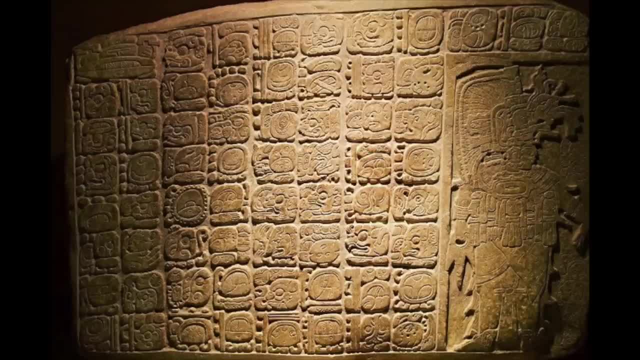 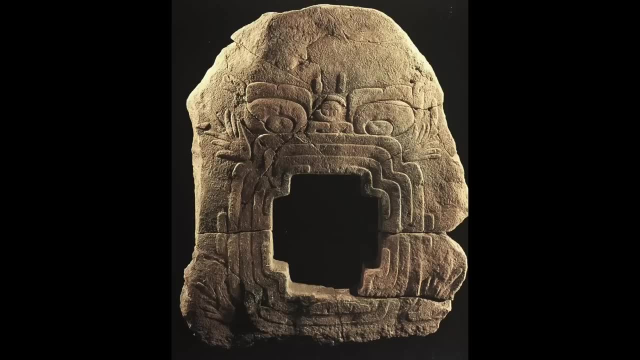 which are probably familiar with if you've looked into the Maya In their day. Olmec influence spread far and wide across Mesoamerica and Olmec style art is found hundreds of miles away from their homeland at sites like Calcadcingo in central Mexico. 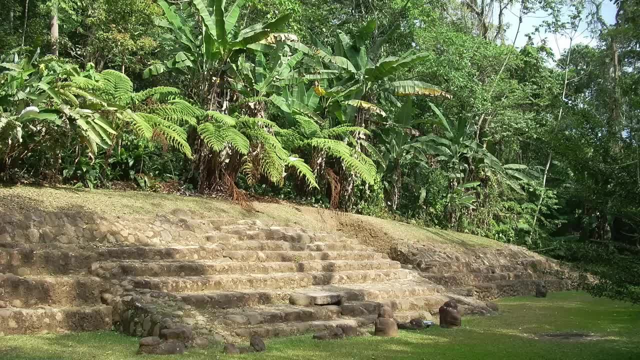 the cave of Octotitlan in western Mexico and Tacology-Cabache in the southern Maya lowlands in Guatemala, possibly because they were running them or because others just wanted to imitate them, or because others just wanted to imitate them. 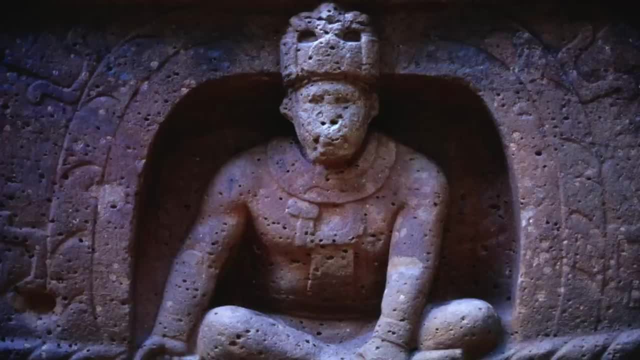 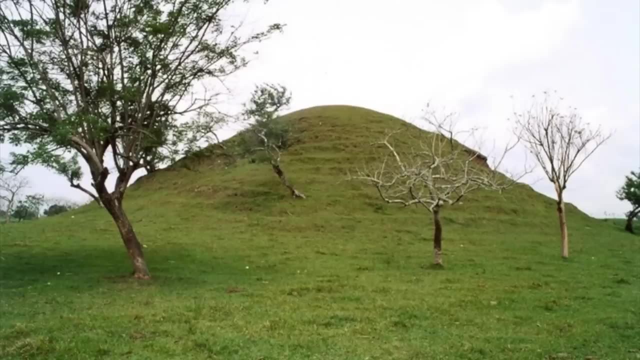 No one knows why exactly the Olmecs disappeared. maybe because of the science, maybe because of the science, maybe because of the science, environmental factors- but the culture that succeeded them was so influenced by them that they're known as the Epi-Omex and they continue to occupy Trezopotes. 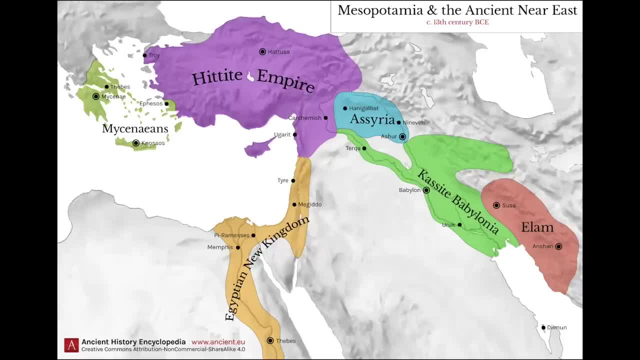 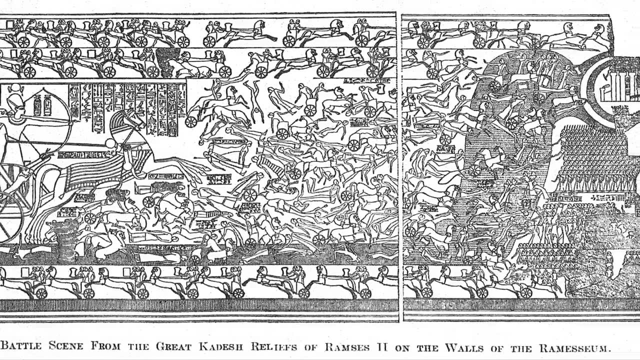 If you've ever delved into the Bronze Age Near East, you'll be familiar with the Hittites, briefly, the arch-rivals of Egypt. Ramses the Great's reputation was built on the famous battle he fought with them over control of the Levant, the Battle of Kadesh Heck. 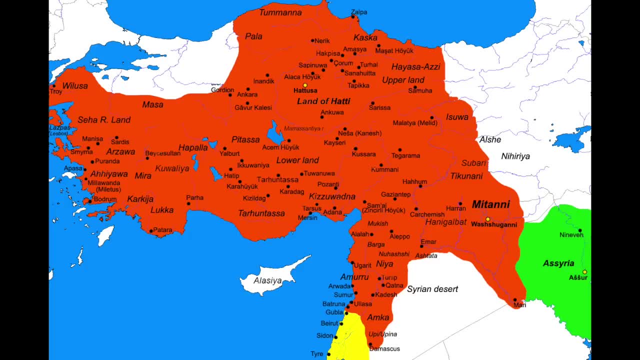 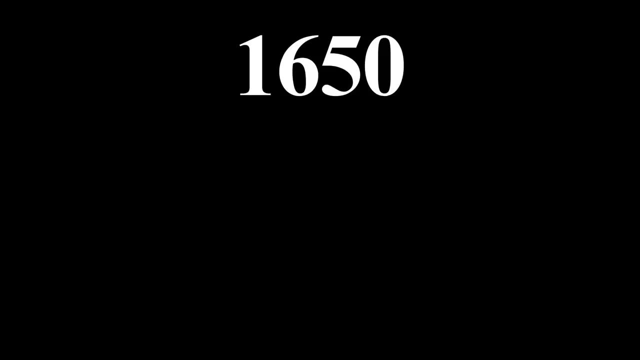 they're even mentioned in the Bible. The Hittite Empire, whose core was referred to as the Land of Hatti by the Hittites themselves, spread over much of Anatolia, the northern Levant and Mesopotamia between 1650 and 1180 BC. Like ancient Egypt, its history is divided into old 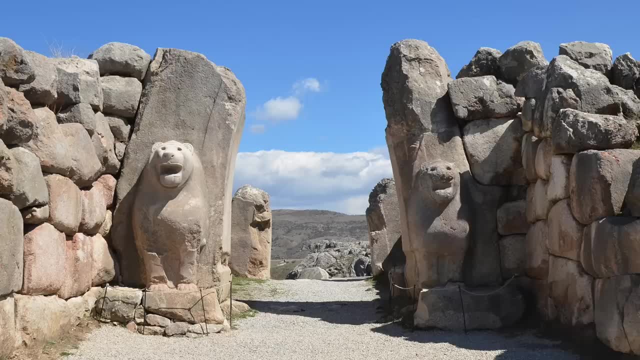 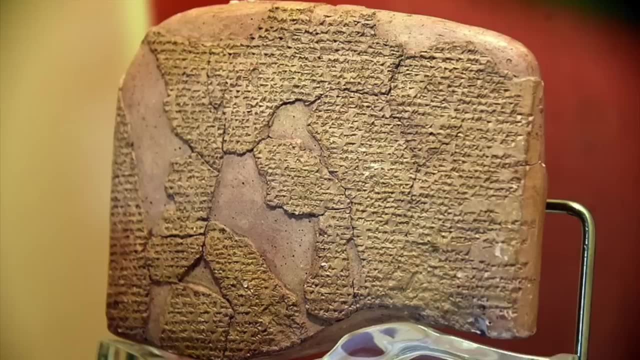 middle and new kingdoms, and its capital was the grand city of Hattusa. They didn't leave behind nearly as many monuments as the ancient Egyptians, but we still know really intimate details of their history because they were meticulous record keepers and they've left. 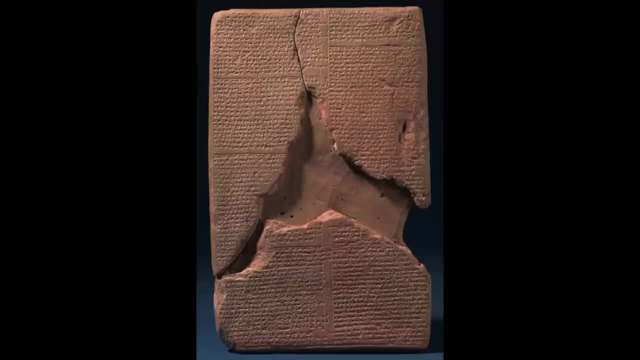 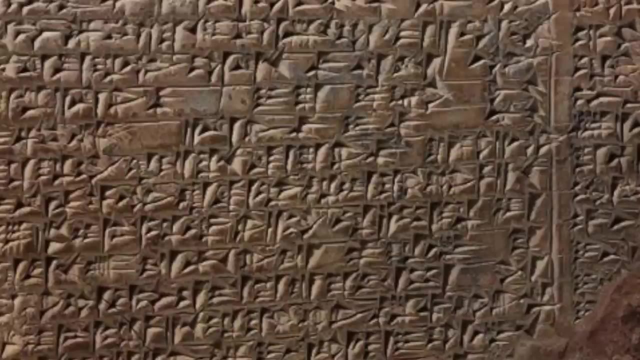 behind their royal archives, which contain tens of thousands of claims tablets inscribed in Akkadian, as well as Hittite and Luwian cuneiform, the oldest recorded Indo-European languages. Fun fact, just like Egyptian, Luwian could also be written in. 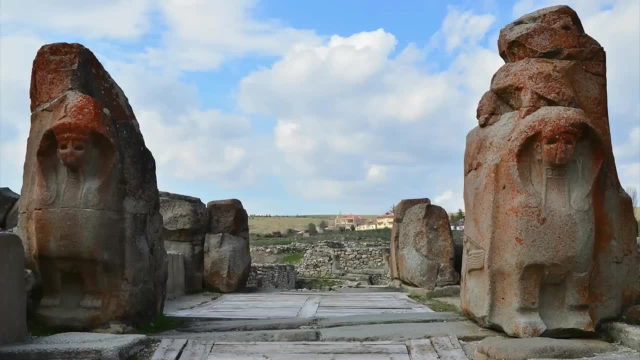 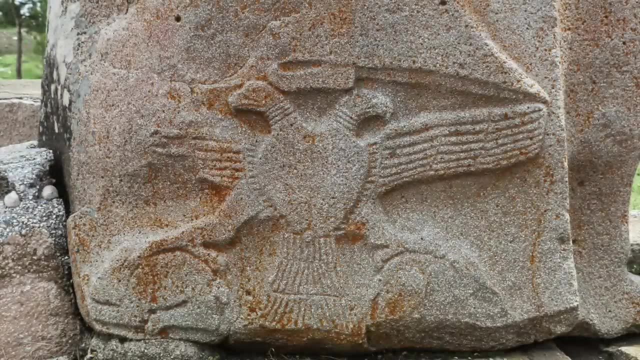 hieroglyphs. That isn't to say there aren't any cool Hittite sites. There's Alacha Hoyuk, which has nice big Egyptian-inspired sphinxes, one of which is decorated with a double-headed eagle. You know where that's gonna go. The rock sanctuary of Yazilakaya, the massive Fasilar. 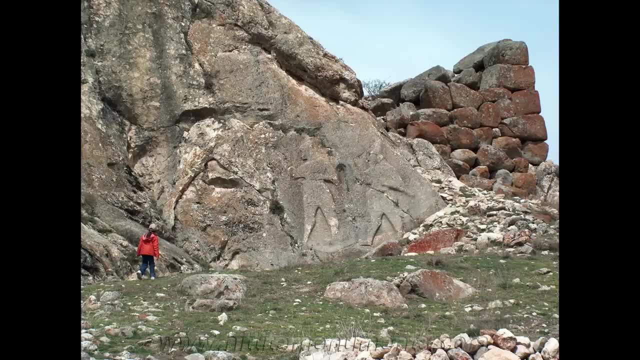 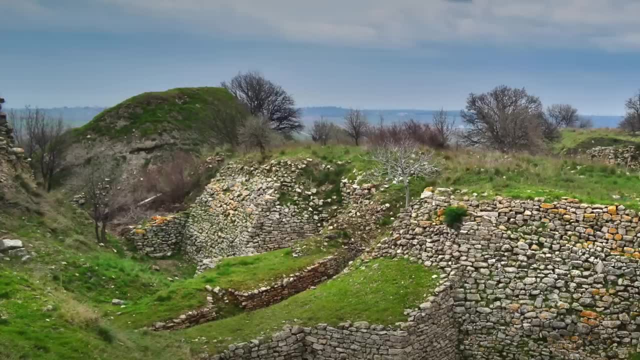 Monument, Eflatun Pinar, And a bunch of rock reliefs absolutely everywhere which the Greeks interpreted in a variety of weird ways. Also, Troy was a vassal kingdom under the Hittites for a bit, and they called it Walusa. Ultimately, though, the Hittite empire was a victim of the Bronze Age collapse. 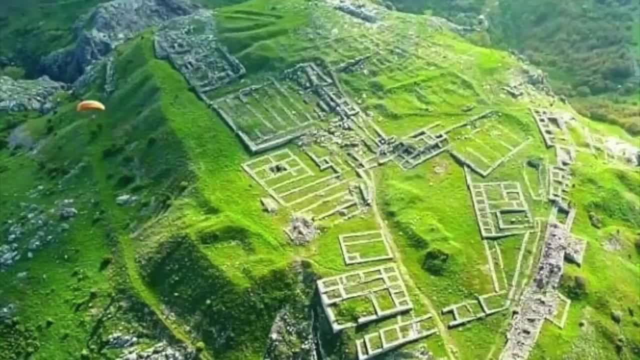 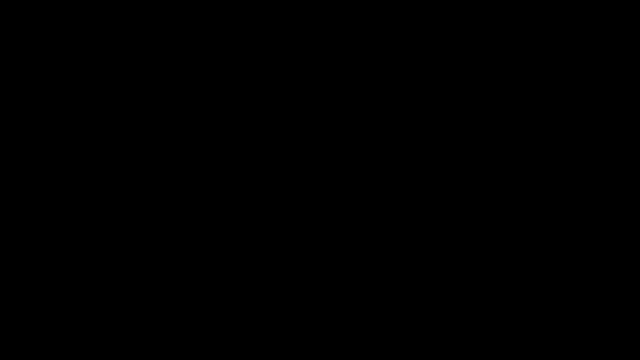 and just couldn't hold up against the constant assaults they faced from the Assyrians, the Sea Peoples and a ton of other various barbarian groups. The Indus Valley Civilization- The Indus Valley Civilization. From the name alone, it's pretty obvious that the Indus Valley 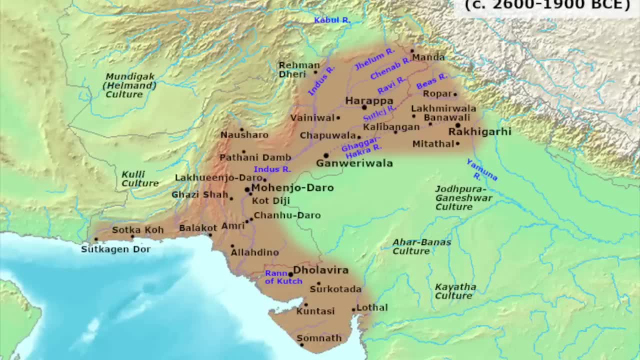 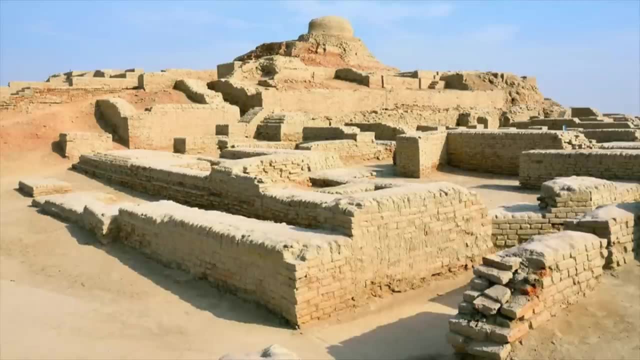 was where they primarily lived along the Indus River Valley, although they did have many sites elsewhere, And the sophisticated, well-planned cities they built, which housed tens of thousands of people, can be found in Pakistan, India and even Afghanistan. They're also called: 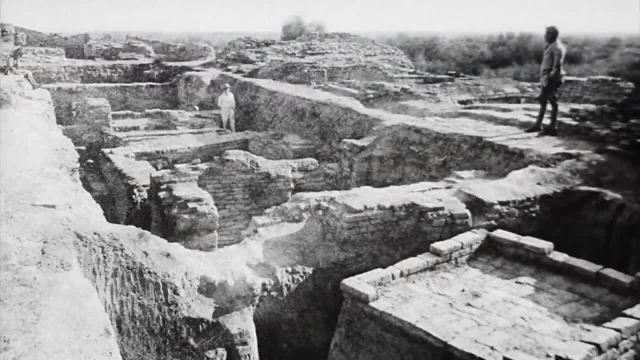 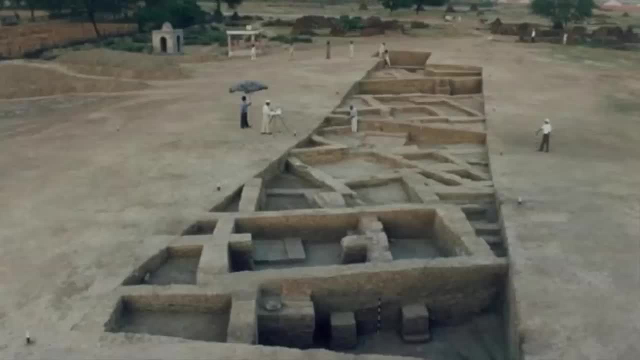 the Harappans, after the site of Harappa, the first of their cities to be excavated, But just as famous, is the city of Mahenjo-daro, the largest and best-preserved one, And they had even more cities, like Dolavira, Rakigarhi and Ganarawala, as well as Lothal, They existed. 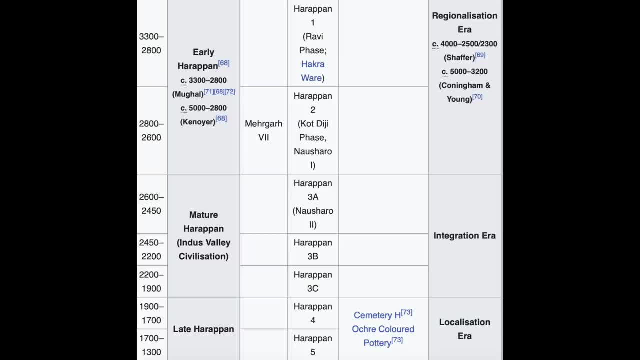 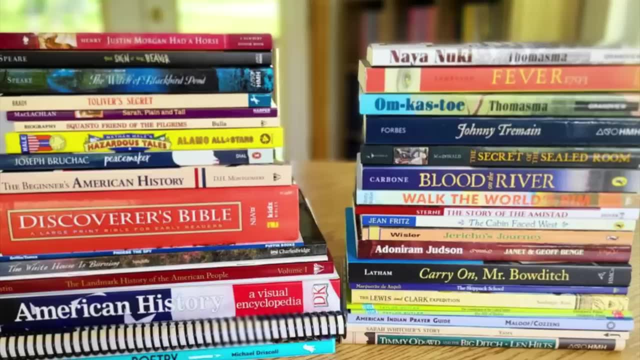 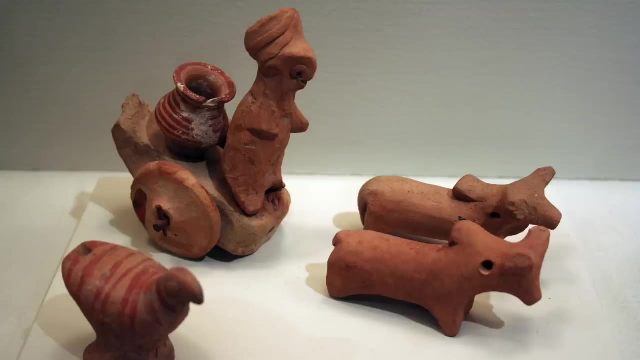 from around roughly 3500 BC to 1300 BC. I'd say they're decently well-known and they're mentioned alongside Egypt and Mesopotamia in a lot of textbooks, mainly because they're one of the early urban river valley-inhabiting civilizations. They were also capable of producing. 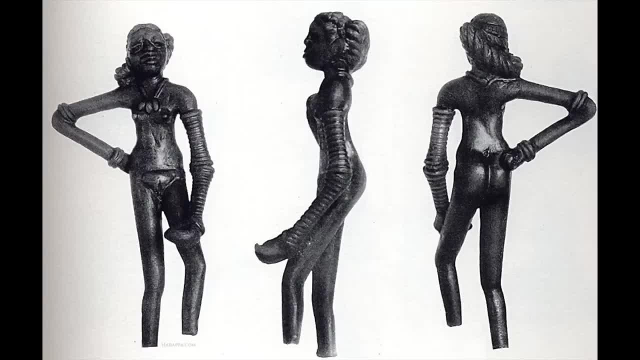 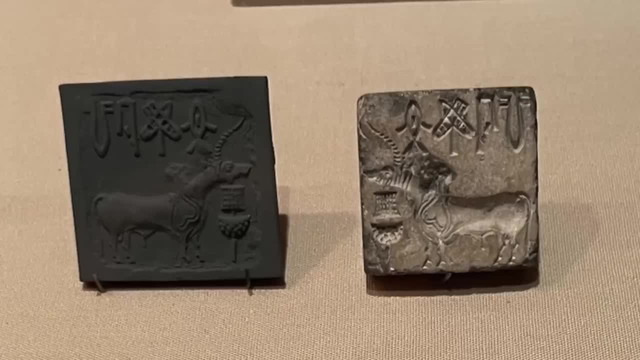 some pretty sweet statues, like the Stone Priest-King or the Bronze Dancing Girl, And they also had a penchant for making tons of terracotta figurines. They had written language called the Indus Script, which has been found on tons of seagulls. 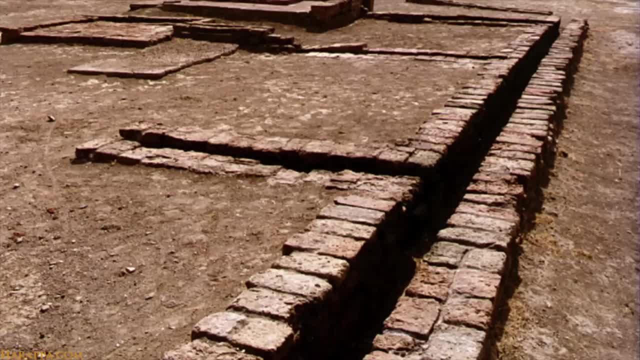 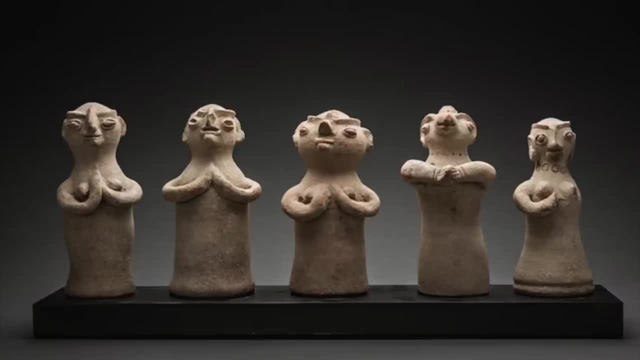 But it's never been deciphered. They also constructed elaborate sewage systems to maintain their cities, as well as baths, toilets and hundreds of wells. In addition, they were oddly egalitarian and their cities don't really feature any palaces or royal tombs. 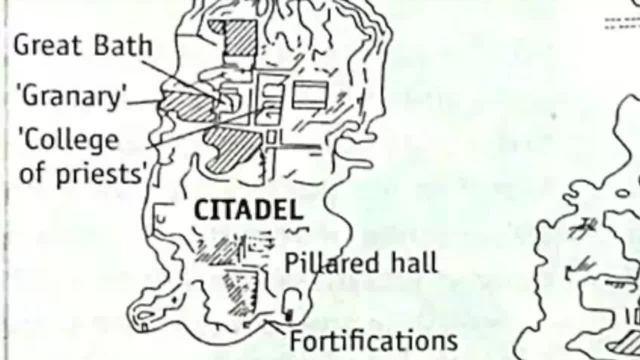 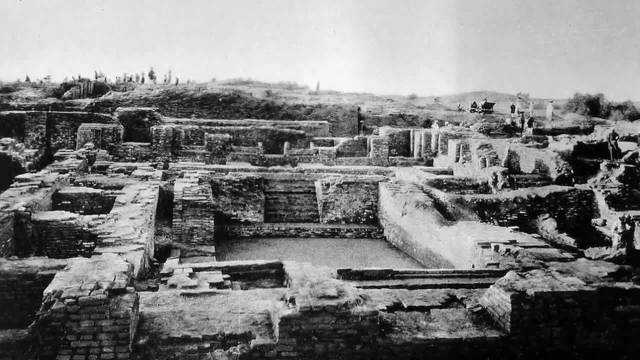 even though they were usually made up of a higher part, or citadel, and a lower part for the upper and lower classes respectively. Mahenjo-daro famously having a great bath in their citadel, possibly ritual in nature, Their history is divvied up in. 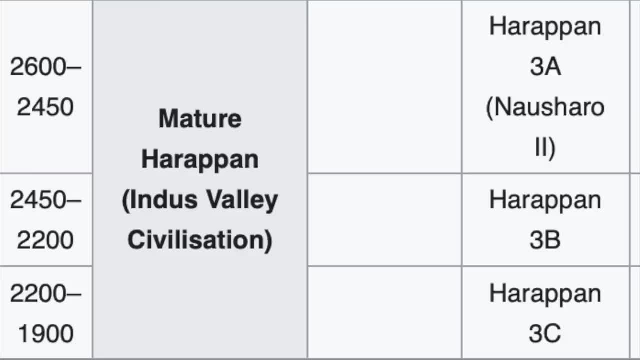 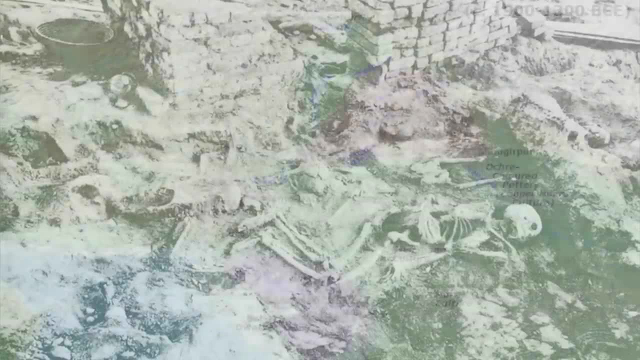 an early phase, when they were first developing, a mature phase which was their golden age, and a late phase which featured the decline of their cities and their abandonment in favor of little villages in the Himalayan foothills, And there are lots of theories about why they. 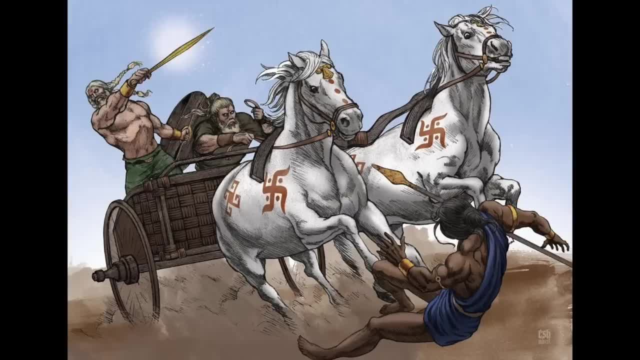 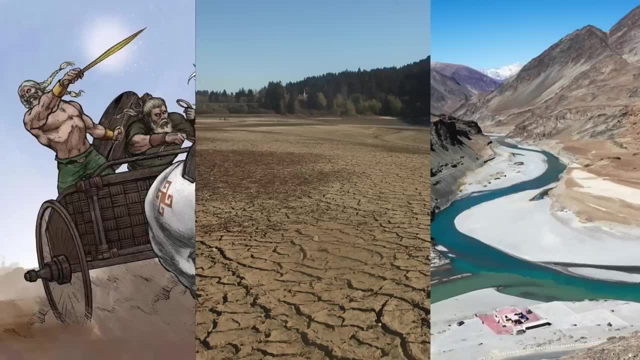 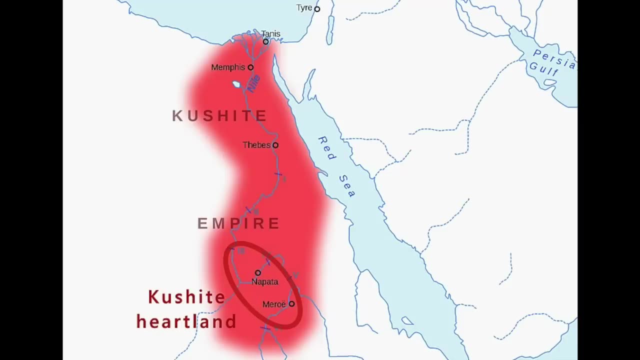 collapsed, maybe because of the arrival of the Indo-Aryans, maybe because of droughts and the changing course of the Indus, or maybe they all just got rolled into one big shitshow. who knows Nubia? By Nubia I really mean the Kingdom of Kush specifically, not any of the cultures that. 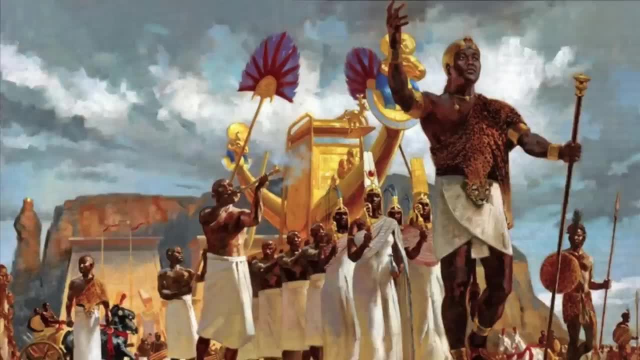 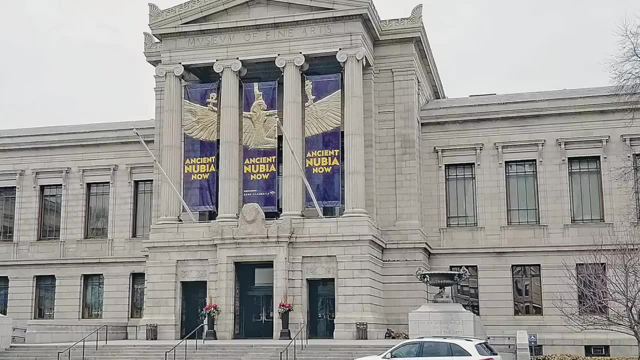 preceded it, like the A-group or the Kerma culture. I feel like Kush is becoming increasingly better known. There have been a bunch of exhibits dedicated to it recently, and I'm sure most people have heard the fun fact that Sudan technically has more pyramids in it than 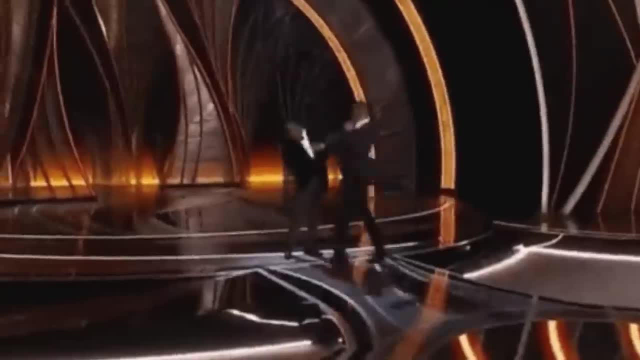 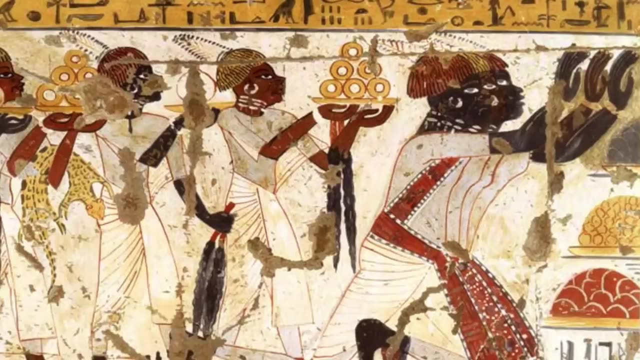 Egypt, which is true sort of, And apparently Will Smith was gonna star in a movie about it at one point, so that's cool. Nubian civilization was heavily influenced by Egypt, since it controlled Nubia for centuries during the Middle and New Kingdoms. but it would be unfair to say 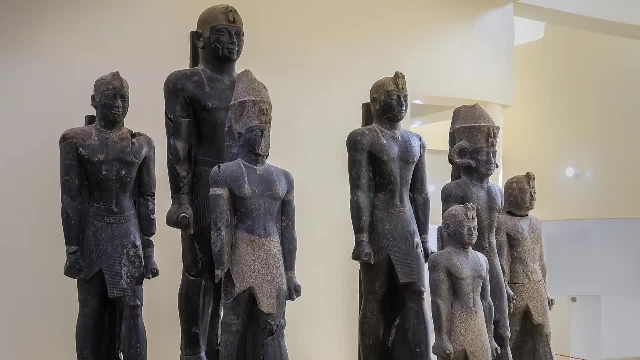 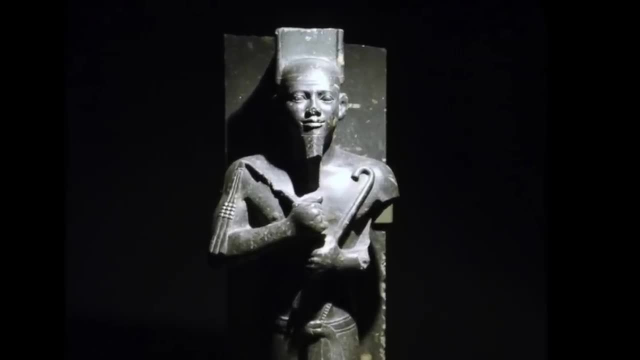 it's just derivative of it. A line of Kushite rulers even conquered Egypt in the mid-eighth century BC after it had fractured into different small kingdoms, and that line of Kushite kings became Egypt's 25th dynasty, ruling until 656 BC, when they were kicked out by the Assyrians. 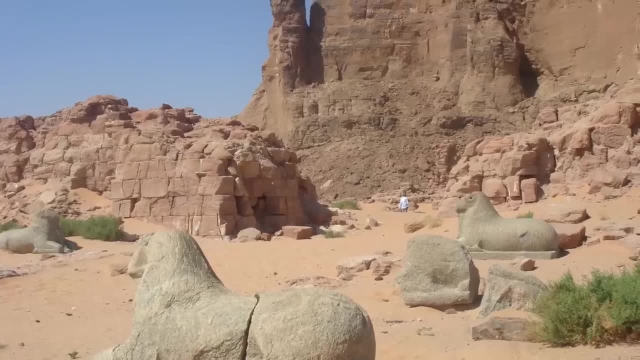 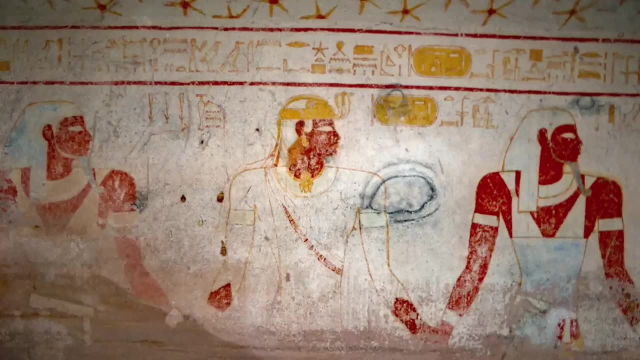 Their capital was initially at the city of Napata, next to a mountain sacred to the god Amun called Jebel Barkal, and at the nearby cemeteries of El-Kuru and Nuri. they buried their kings on a mountain called Jebel Barkal and at the nearby cemeteries of El-Kuru and Nuri. they buried their kings on a mountain called Jebel Barkal. 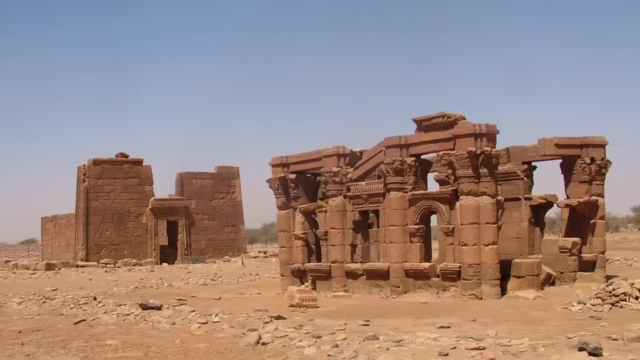 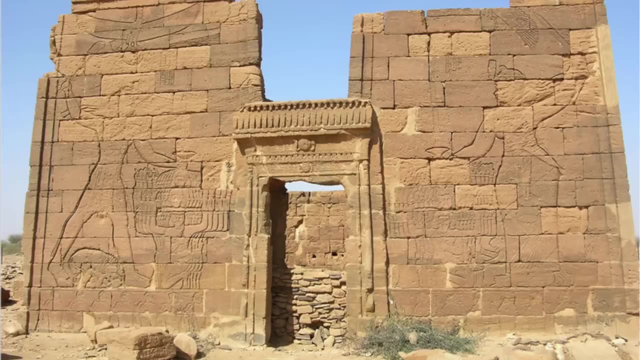 under steep-sided pyramids with lavish burial goods. They built a bunch of other really cool monuments elsewhere too, like the colossi of Natakamani, the temples of Naka and Musawat es-Sufra, which I specifically like because it has an 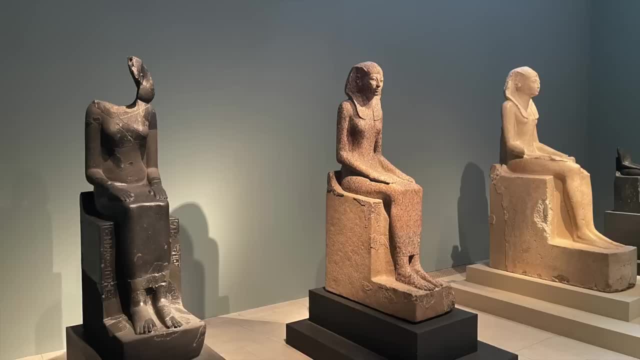 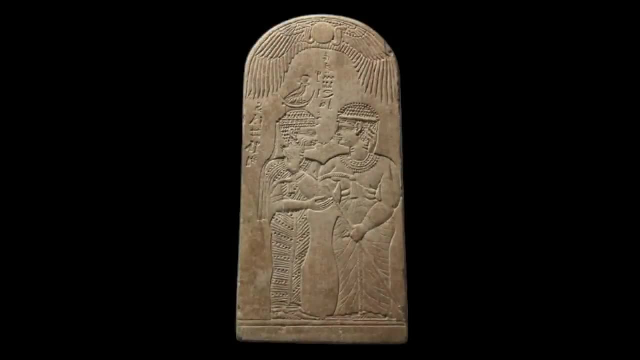 elephant sphinx, which I think is really cool, among many others. Unlike in Egypt, where female pharaohs were exceptionally rare, female rulers were far more common in Kush, since the throne was inherited matrilineally and queen mothers. known as Kandakis were considered to be the most powerful rulers in Egypt. After Napata was sacked by the Egyptians around 591 BC, they moved further south to the city of Meroe and erected even more pyramids there. 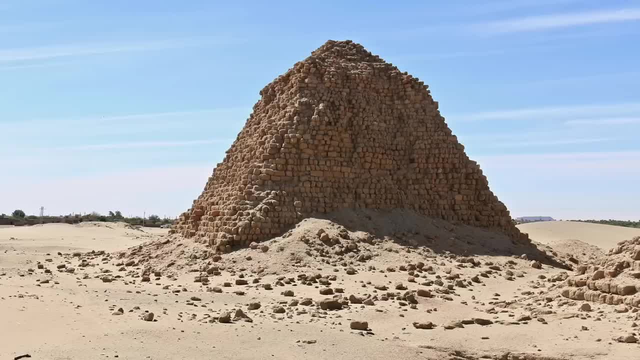 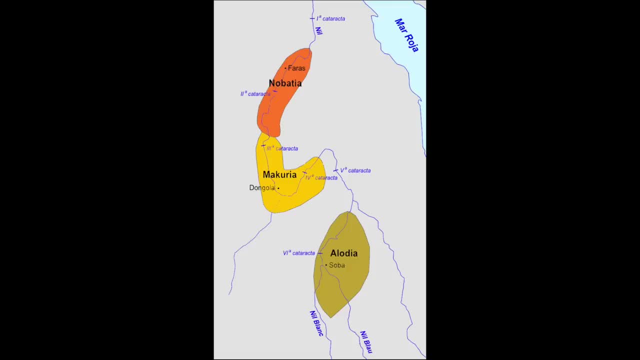 And here they even developed their own hieroglyphic script known as Meroitic. But eventually Meroe fell in the 4th century AD and Christianity took hold. The kingdom of Kush was succeeded by three smaller, staunchly Coptic, Orthodox kingdoms. 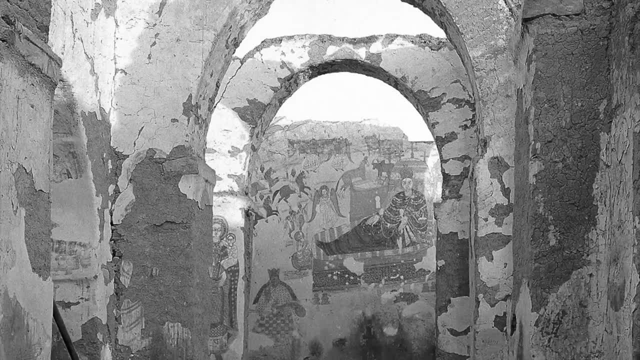 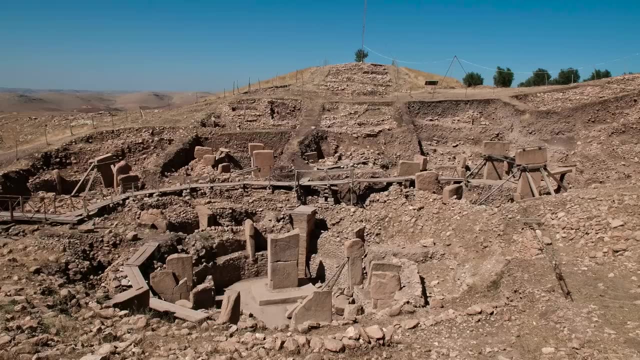 Nobatia, Alodia and Makurana, The latter two remaining independent and Christian into the 15th century. Gebekli Tepe. Gebekli Tepe is an extraordinary site on a mountaintop in southeastern Anatolia that 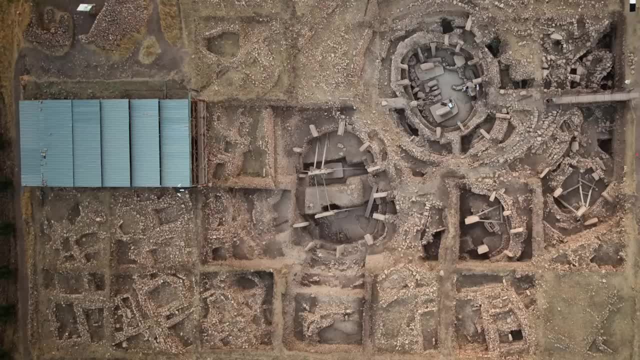 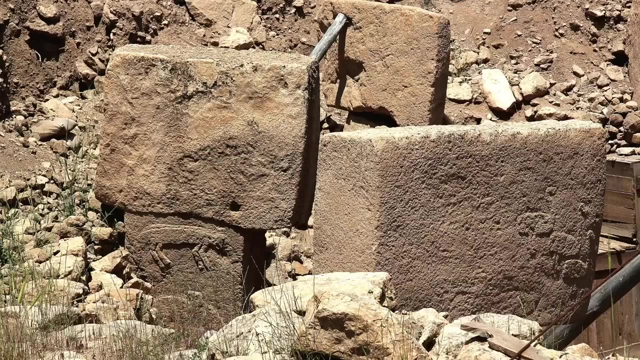 might very well be the oldest temple in the world. It's made up of a number of circular enclosures filled with enormous T-shaped pillars decorated with all sorts of symbolic imagery, like birds and scorpions, and lions and tons of other. 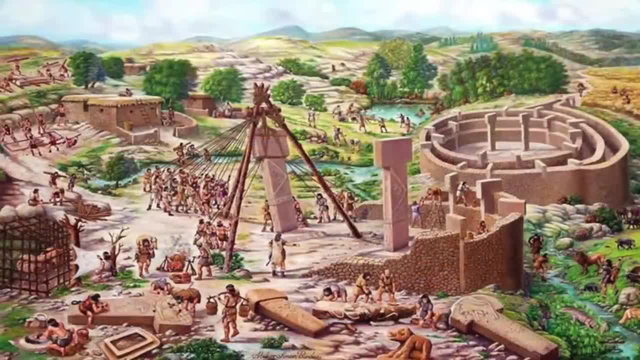 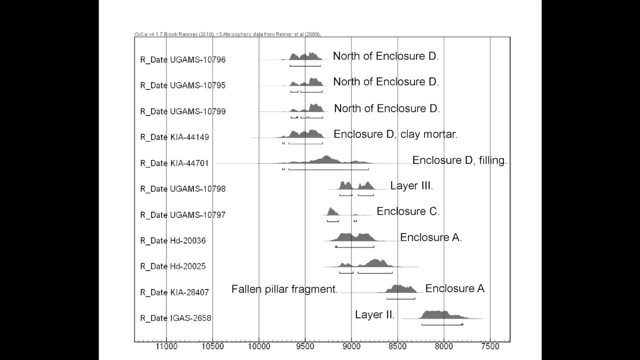 stuff. It was built somewhere between 9,500 and 8,000 BC, so that's like 11,000 years ago. based on radiocarbon dating of the plaster and charcoal found there, so it's by far the oldest thing. 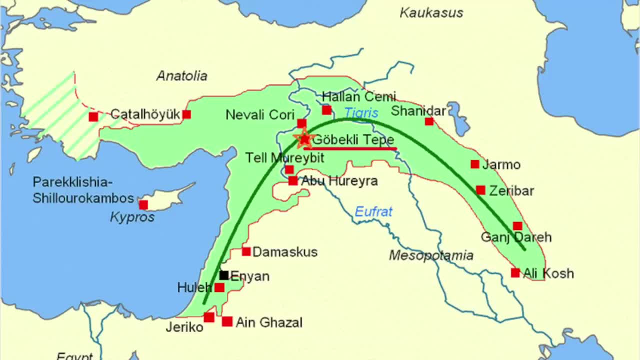 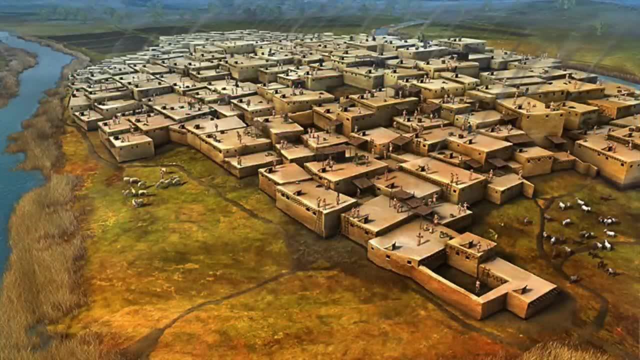 on this list. It was made during what's dubbed the Pre-Pottery Neolithic Period, which lasted from 10,000 BC to 6,500 BC, when the first ever villages started to appear and agriculture really started being adopted in earnest for the first time. 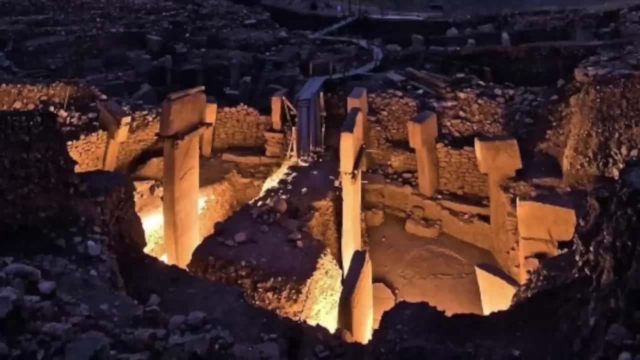 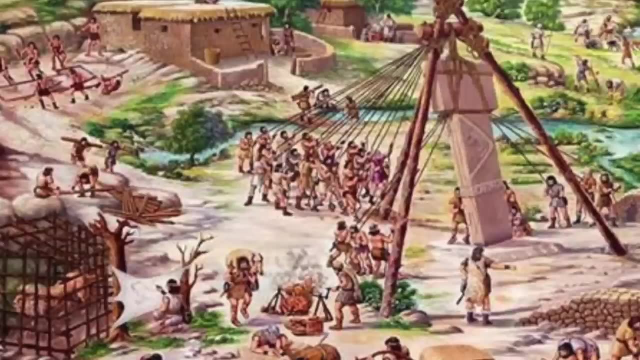 All around the Fertile Crest. In addition to being a sanctuary, it was also a settlement site, with a rainwater collection system and big stone vessels probably used for brewing beer. But there's still no evidence that the people who made this practiced agriculture, which 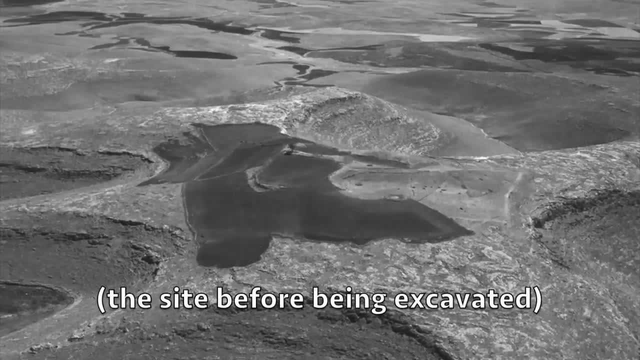 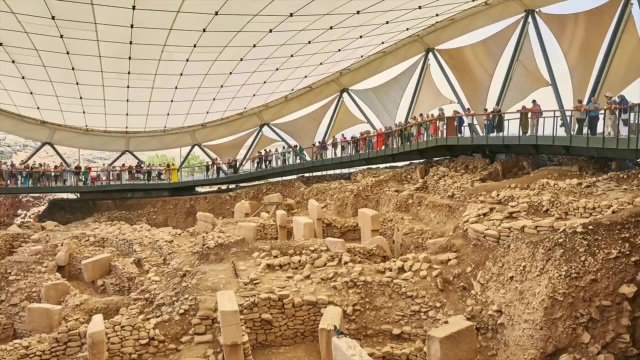 makes it all the more impressive. It was only really discovered in the 90s by the late German archaeologist Klaus Schmidt. but because it's so exceptional, I think a lot of people know it by now. And this isn't the only site of its kind. other sites in the region are also filled. 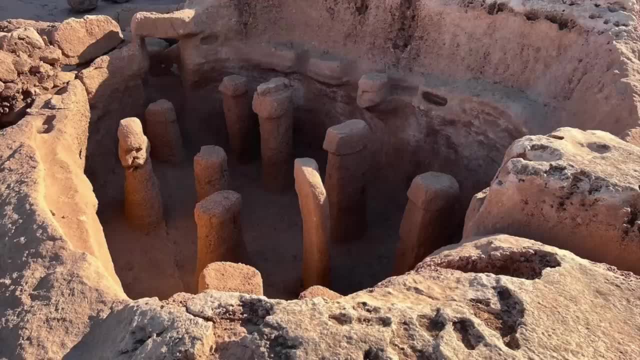 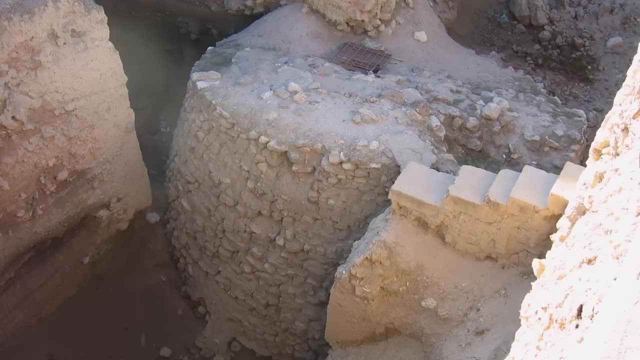 with the same sort of T-shaped pillars. Like Karahan Tepe and Pre-Pottery. Neolithic sites further afield have revealed just as fascinating stuff, Like this tower from Jericho in Palestine, which might be the oldest piece of monumental architecture in the world. 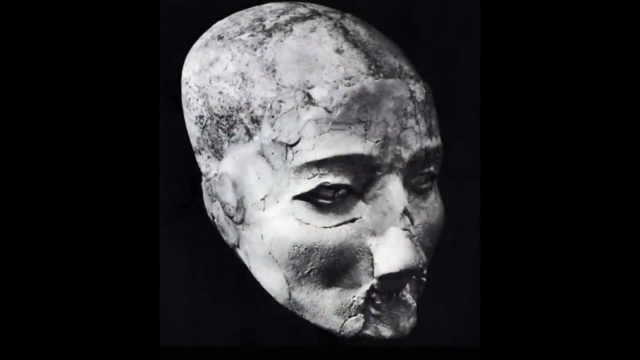 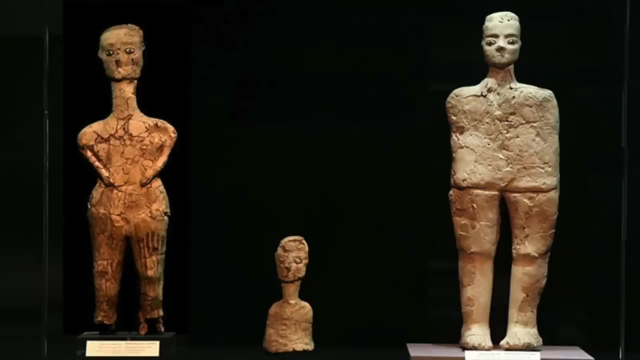 And also found at Jericho are these skulls covered with plaster to imitate the faces of the people they once belonged to, which have also been found at a bunch of other sites. And I can't mention the Pre-Pottery Neolithic without mentioning these weird statues straight. out of a fever dream, made of plaster and reeds from a tree. And I can't mention the Pre-Pottery Neolithic without mentioning these weird statues straight out of a fever dream, made of plaster and reeds from a tree. 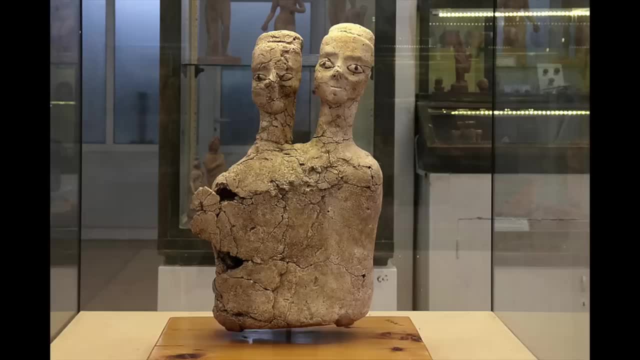 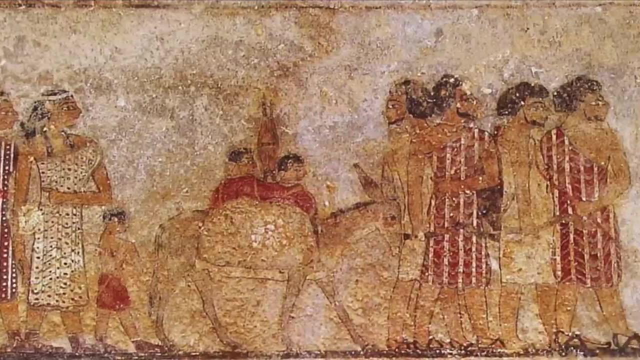 And I can't mention the Pre-Pottery Neolithic without mentioning these weird statues straight out of a fever dream, made of plaster and reeds from a tree Like theseெ Canaanites. Canaanite is the catch-all term for semitic speaking peoples who inhabited the southern 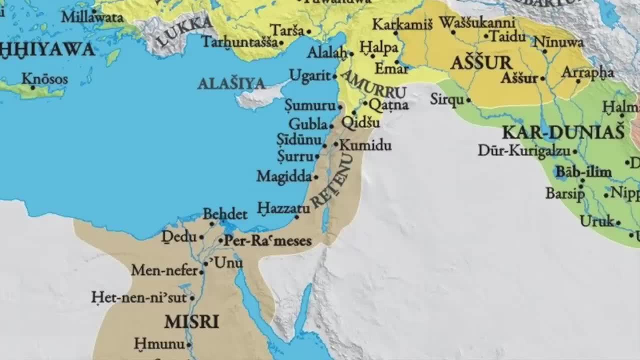 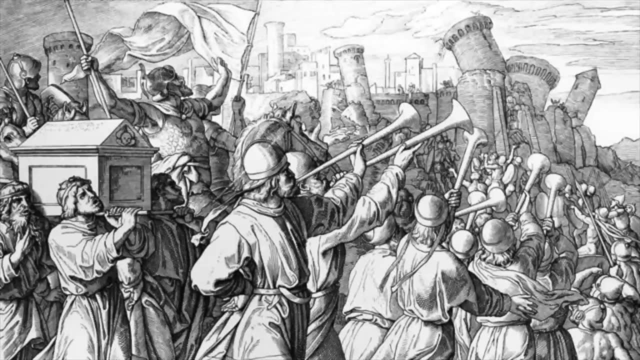 Levant during the third and second millennium BC, during the bronze age. They're mentioned in the bible a whole ton of times because they're the people Joshua had to kick out of the promised land so the Hebrews could settle there after the exodus. 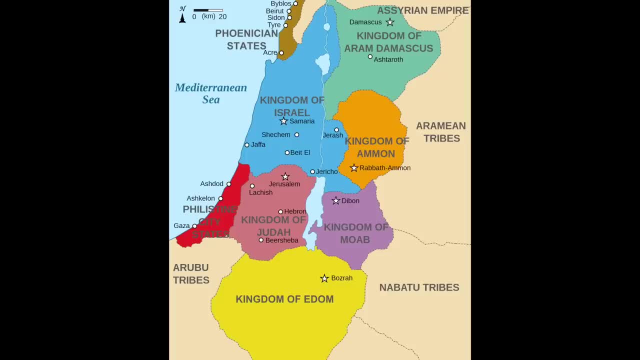 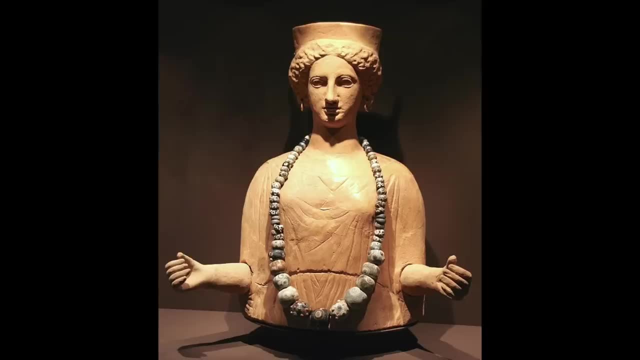 even though in reality, the Hebrews, along with all of their weird neighbours like Moab, were actually most likely ethnically Canaanites themselves. The Phoenicians were also Canaanites, but I didn't want to group classical North Africa with the Bronze Age Levant. 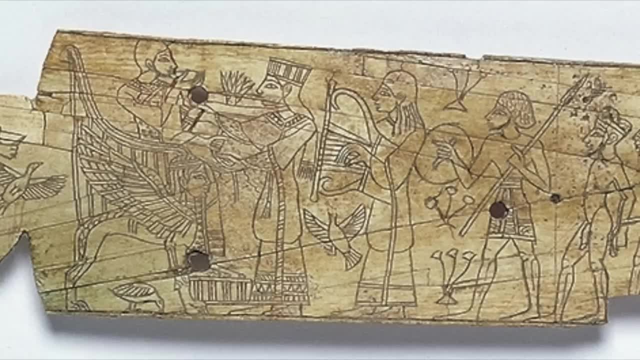 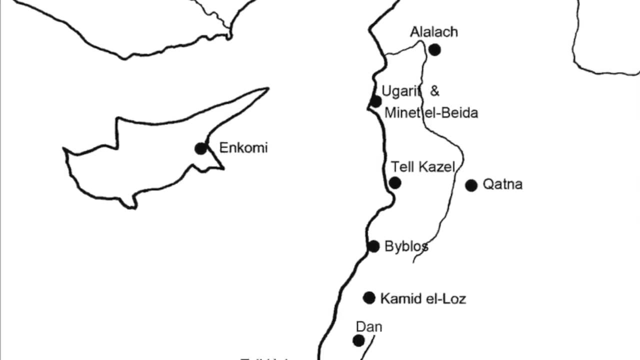 so that's why I divided them. They were heavily influenced by the Egyptians and Mesopotamia and they were a real crux of Bronze Age trade networks. But, as I alluded to, they weren't a united whole. They were divided into a ton of different, often warring, city-states. 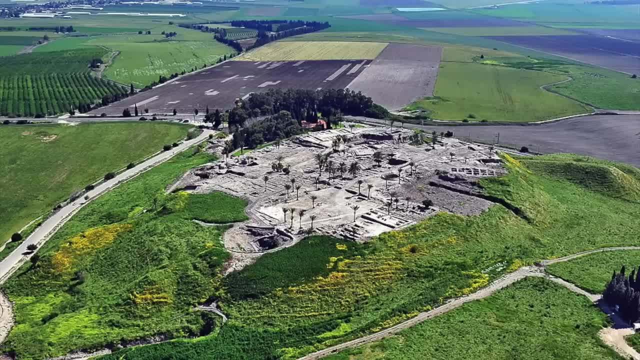 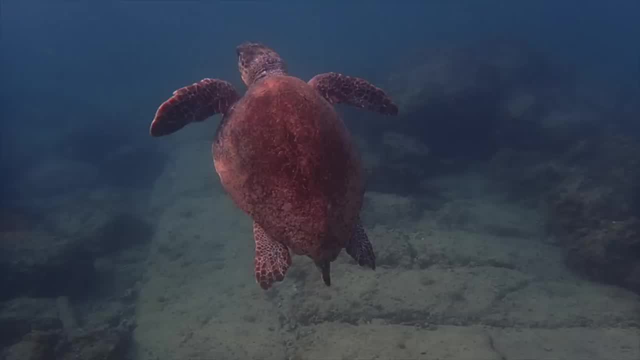 Some important ones being Hazor, Gezer, Megiddo, where the word Armageddon comes from Lachish, Beit Shein, Byblos, where the term Bible comes from Tyre, Sidon, Shechem and Ugarit. 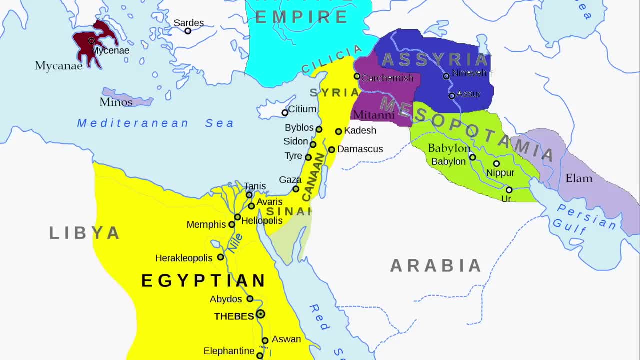 But Ugarit was so unique that I actually have it listed here separately. Most of these were under the suzerainty of the pharaoh during the Egyptian New Kingdom, although right before that, during Egypt's second intermediate period, a group of Canaanites known as the Hyksos actually conquered Lower Egypt for a time. 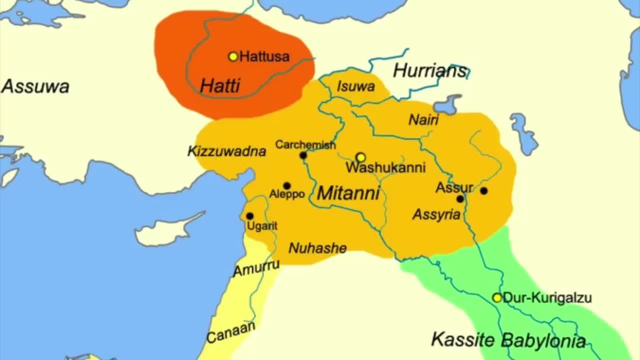 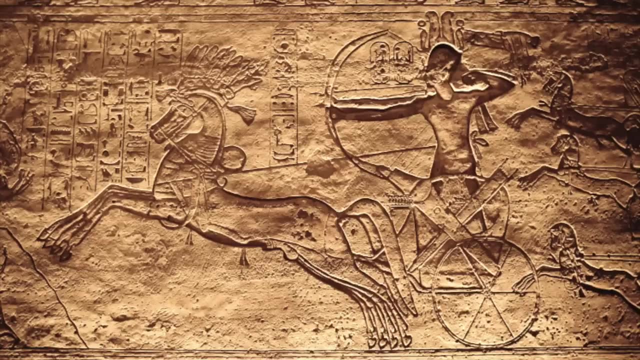 The kingdom of Mitanni and the Hittites from the north also had stakes in the region and the aim of a lot of the campaigns directed by great New Kingdom pharaohs like Thutmose III and Ramses II were meant to combat their influence in the region. 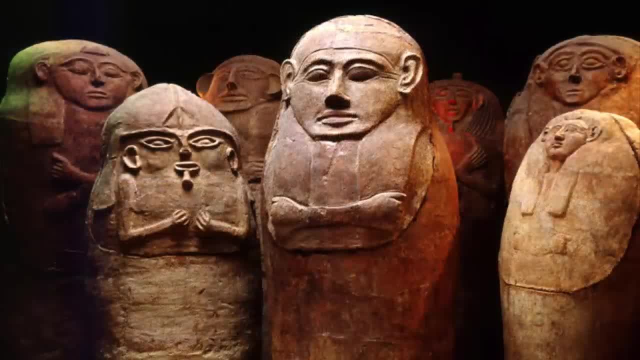 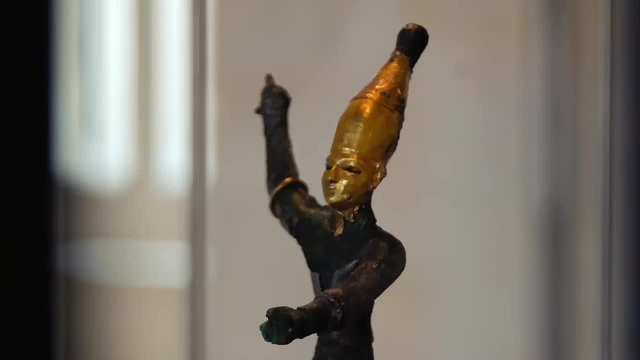 I think the most telling signs of Egyptian influence are these strange pseudo-Egyptian clay anthropoid coffins and the fact that their gods, like Baal, famously often wear Egyptian headdresses, and just the sheer amount of Egyptian stuff found in the Levant. 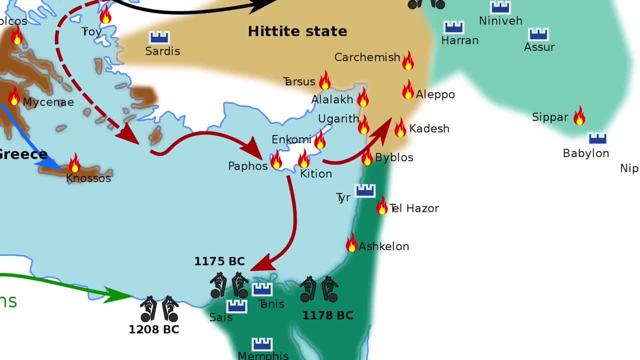 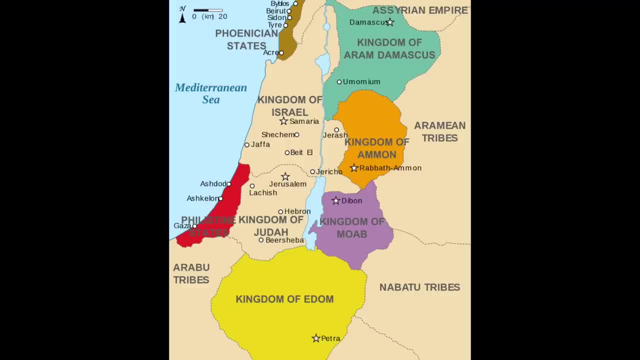 But eventually the Egyptians just had to pull out during the Bronze Age collapse, when they were being swarmed by the Sea Peoples. And at this point, at the beginning of the Iron Age, the Canaanites coalesced into various kingdoms. 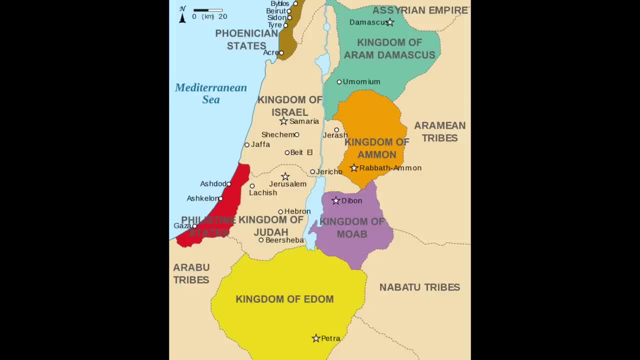 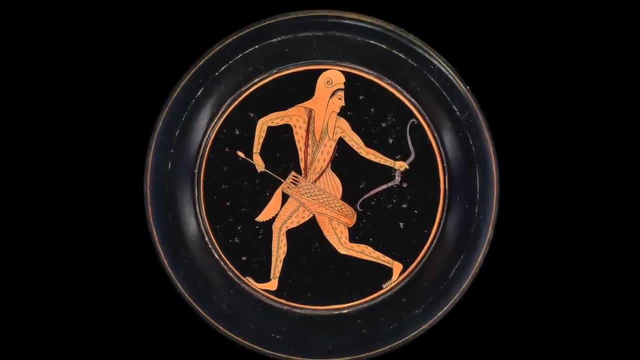 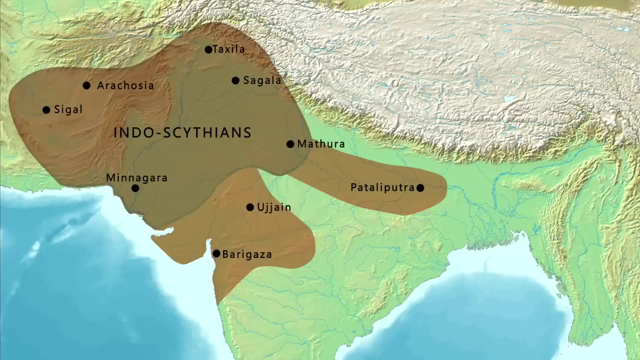 like Judah Israel and its many strange neighbors, Which I'm not gonna cover, The Scythians- These Eastern Iranian nomads played a huge role in the history of Siberia, Central Asia, Eastern Europe, the Balkans, the Near East and even India. 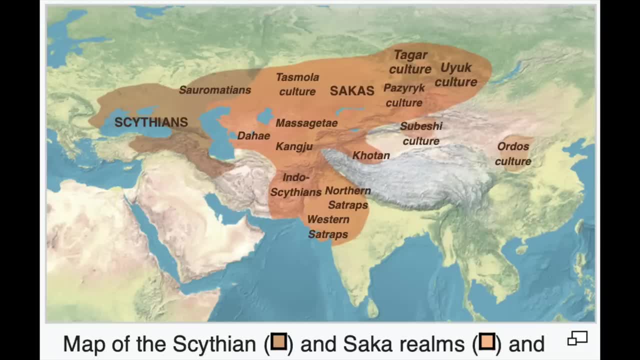 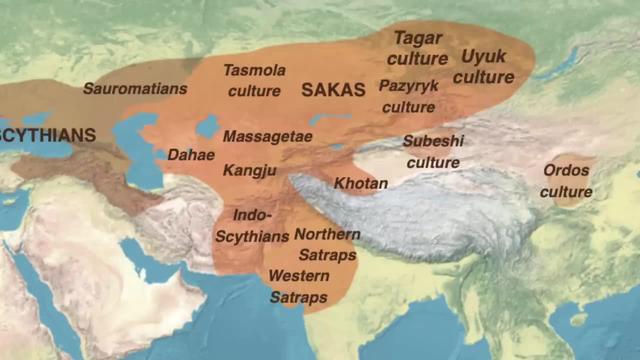 So they had quite a far reach. They're divided into two closely related groups: The Scythians, who dominated the Pontic steppe between the 7th and the 13th century, and the Sakkas of the Asian steppe. 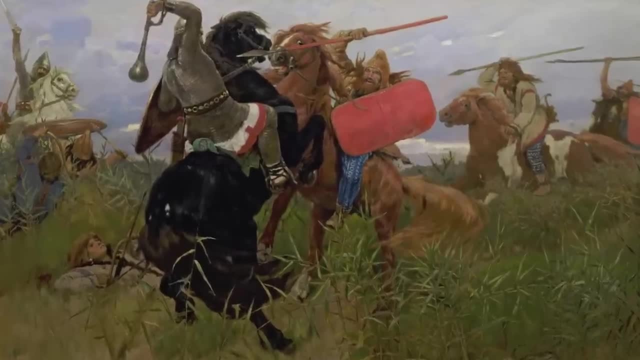 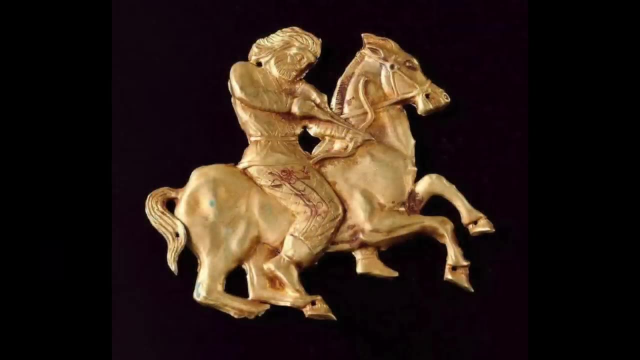 And they lasted a bit longer. They're especially well known in Eastern Europe for the huge role they played in its history, So that's why I put them here. They were known far and wide as fierce mounted archers who lived as nomads across the Eurasian steppe. Interestingly enough, according to my man, Herodotus, the Scythians in general never washed their bodies. Instead, they would just throw hemp on a fire and close within a tent and immerse themselves in the vapor, which they obviously also got high on. 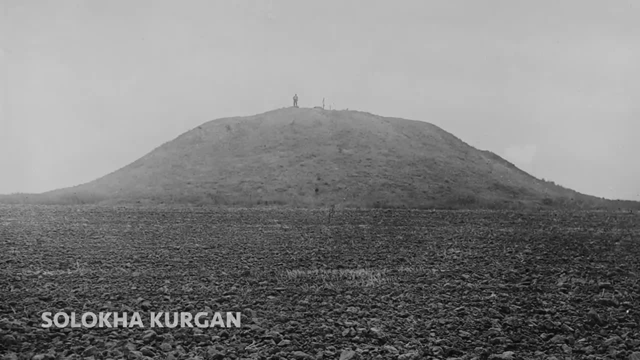 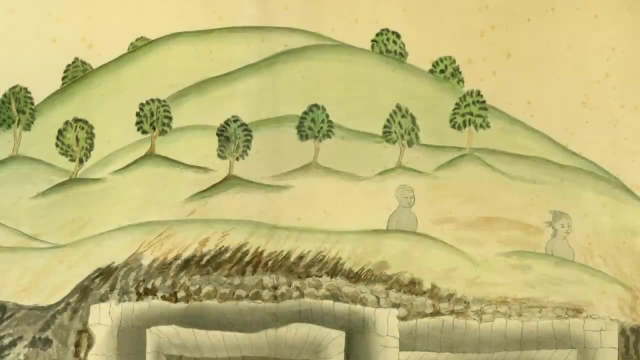 They left behind huge burial mounds or kurgans filled with lavish burial goods, like the Arzon kurgans, the Bazarik burials and the Issac kurgan, And they sometimes set up stelae. 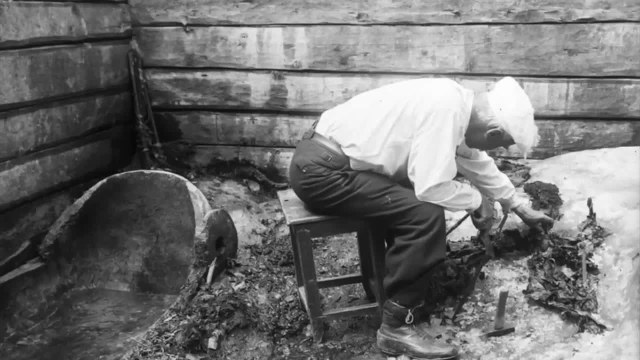 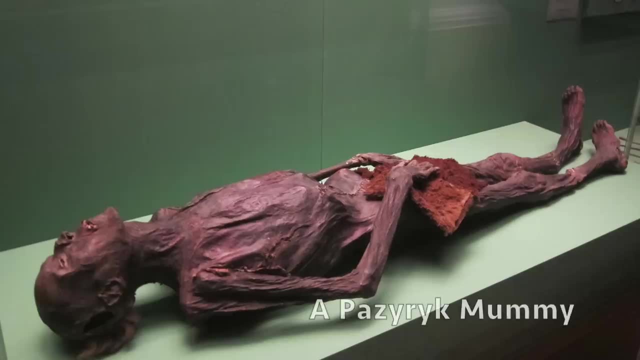 depicting the deceased next to these kurgans. Due to the preservative effects of the Siberian permafrost, which has famously preserved woolly mammoths, and the fact that they deliberately embalmed their deceased, a bunch of Scythian mummies have been discovered. 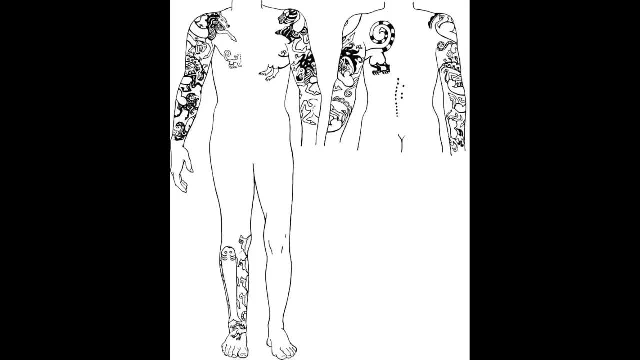 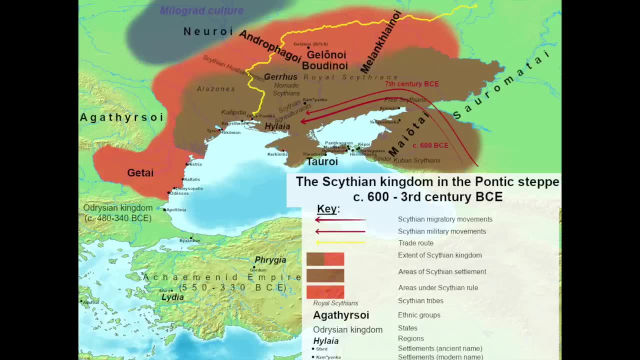 And they've attracted a lot of attention because some of them were covered in tattoos Which some people have actually replicated on themselves. While the Scythian Scythians were in what's now Ukraine, the Sakas also formed kingdoms in the Tarim Basin. 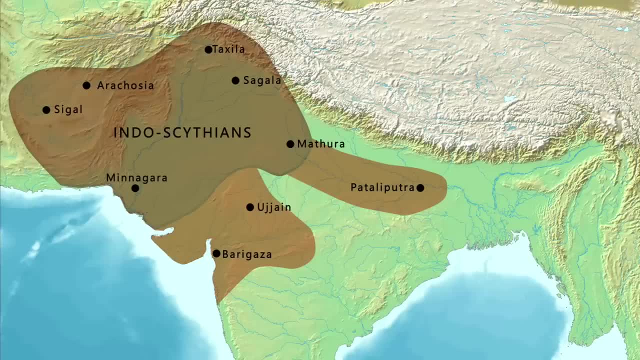 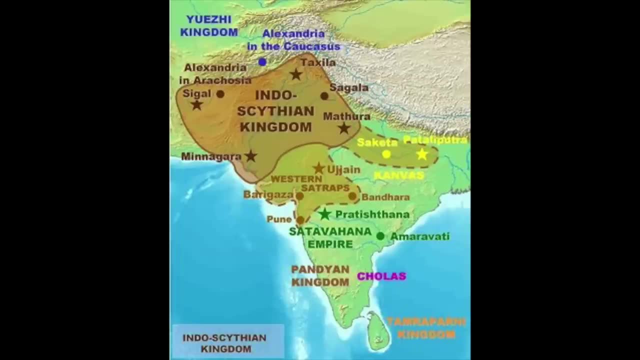 like Khotan and Kashgar and became Buddhist. Some even made their way to India And, after crushing the Indo-Greek kingdom, these so-called Indo-Scythians formed kingdoms in northwestern South Asia, One of which whose rulers were referred to as the Western Satraps. 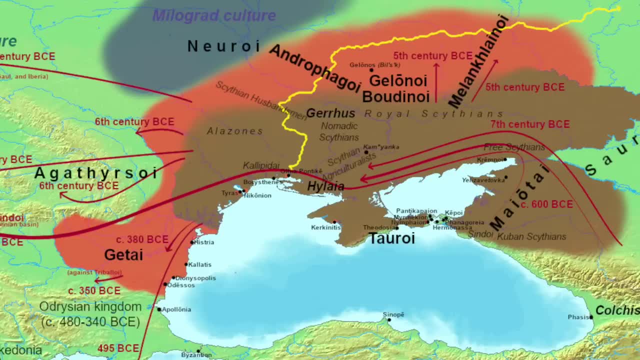 lasted until around 400 AD, But far before that. the Scythian dominance on the Pontic steppe came to an end in the 3rd century BC, when they got BTF'ed by the Celts, Germans and Sarmatians. 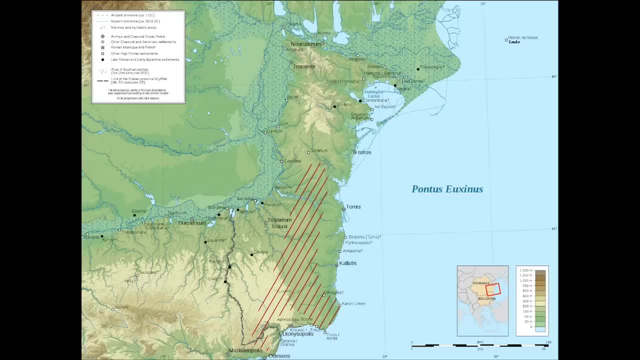 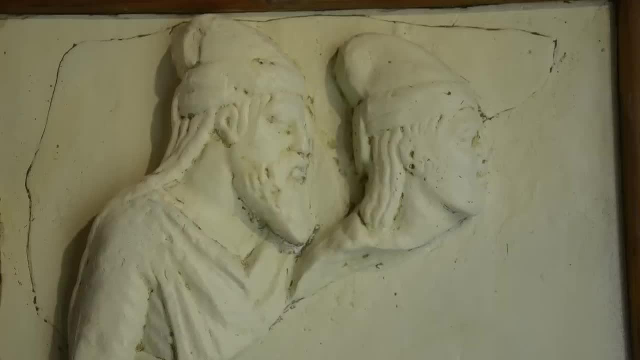 But they still ran two little kingdoms in the Crimea and along the Danube, both called Scythia Minor, where they became sedentary and Hellenized. But after a few centuries they were eventually just assimilated by their conquerors. 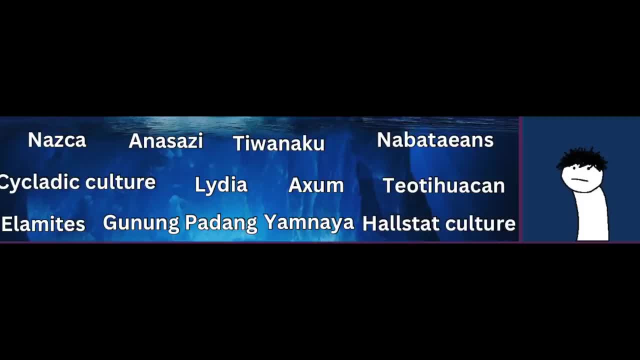 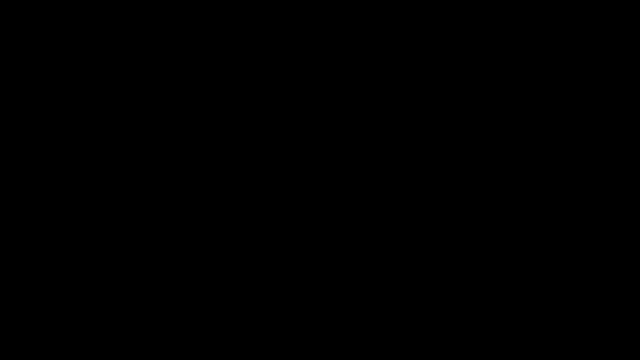 Level 3. Okay, so we're finally under the water with this one, and the guy next to us is looking a bit disheveled and greasy. So let's see what we find: The Early Cycladic Civilization. This civilization existed in and gets its name from, 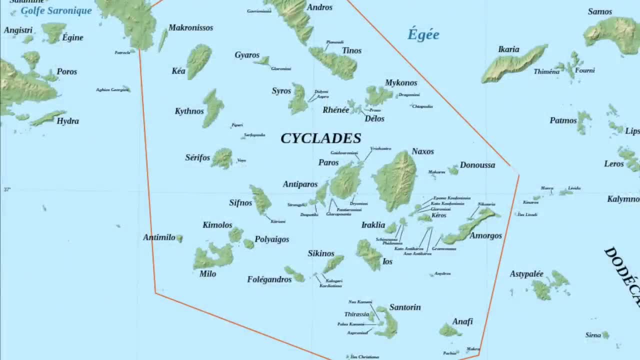 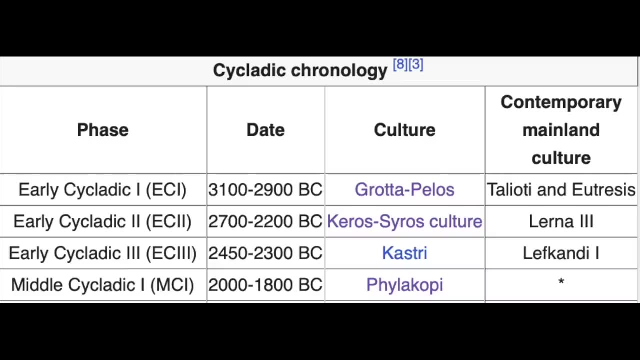 the Cyclades, a group of islands in the Aegean just off Greece which are rich in minerals, ores and fine fine marble. It emerged in the Early Bronze Age, around 3200 BC, and it's divided into two phases. 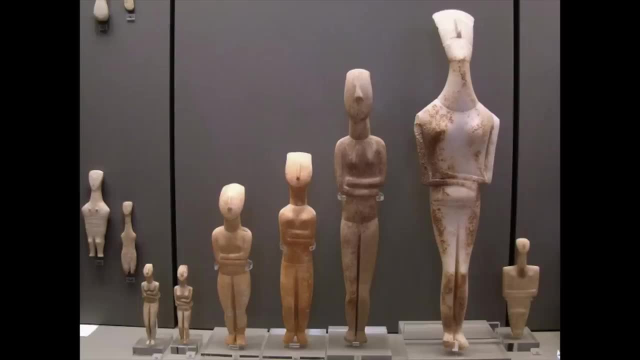 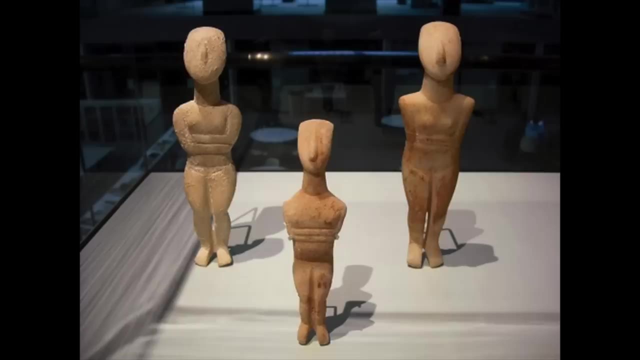 the Grotopylos period and the Keroseros period, when it reached its zenith And the population boomed. These are also known as Early Cycladic I and II. They're best known for mass-producing these strangely abstract marble figurines. 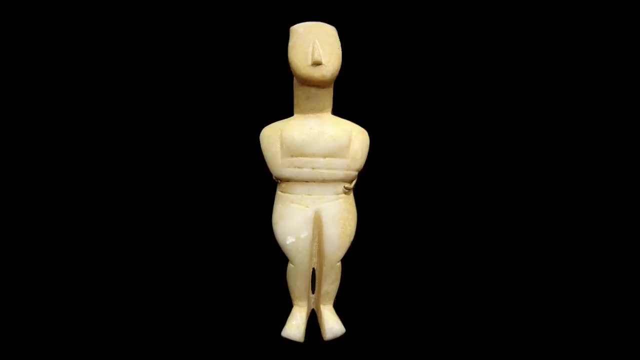 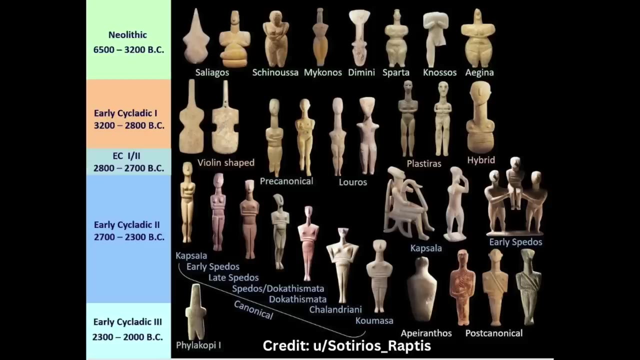 the most common type of which is a full-length female with folded arms, the so-called folded arms figurine, which comes in all sorts of different varieties, made in different places at different times, But they made some other types of figurines too. 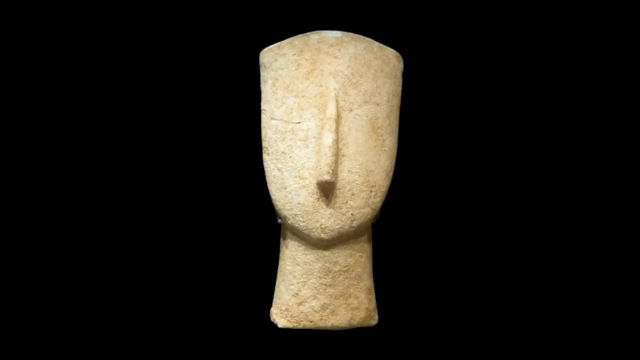 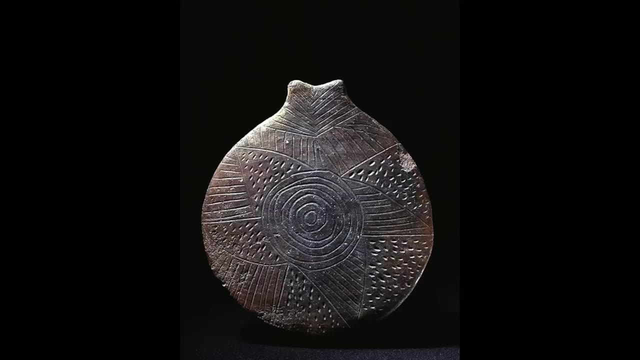 like this harp player. Their faces look eerily blank, asides from their noses, but traces of paint on them suggest that they were once actually painted. Less well-known, but just as interesting are these elaborate frying pans. they made out of terracotta and stone. 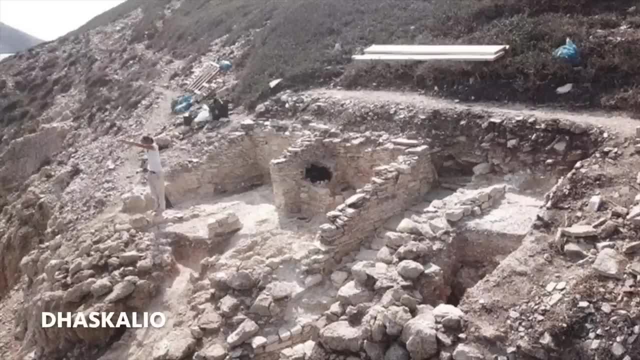 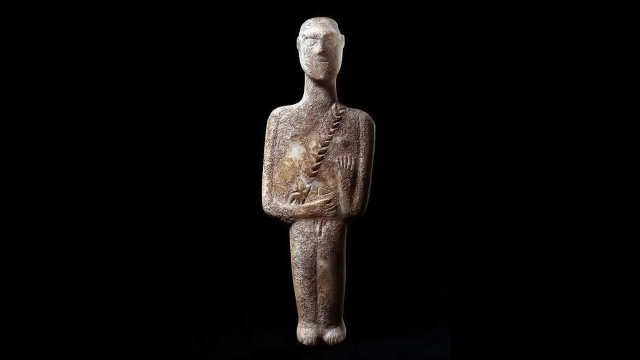 and no one knows why they made them. At the end of the Early Cycladic II period, old settlements were abandoned and new, heavily fortified ones built in remote locations, took their place, And this also coincides with male figurines with baldrics and daggers being produced. 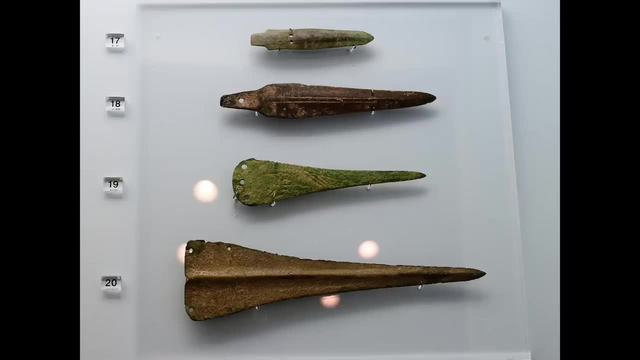 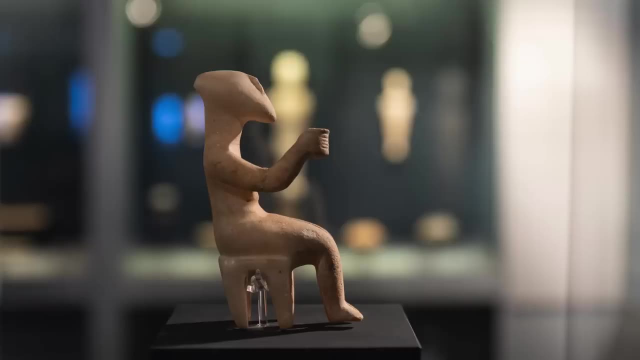 which suggests that there is some unrest, possibly due to conflicts over resources and trade. But their sites weren't just ravaged in antiquity. Early Cycladic sites have suffered from intense looting, as private collectors are desperate to add the figurines to their collections. 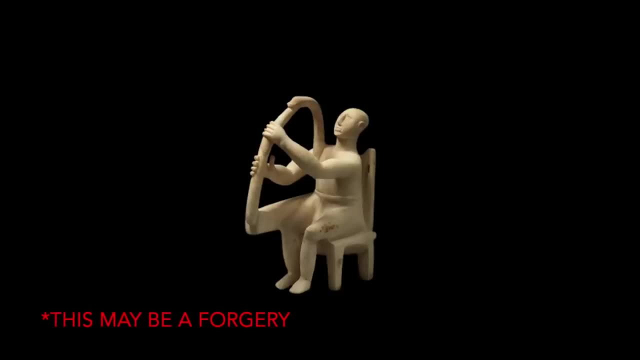 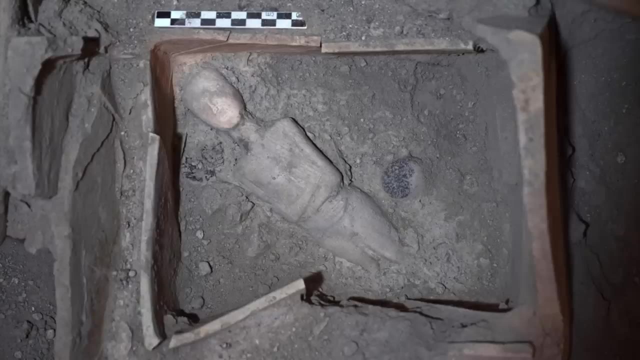 And for the same reason, the market has also been flooded with tons of forgeries of them, So we don't know exactly which context the vast majority of these figurines came from, though a lot of the excavated ones come from graves, and some of the ones displayed in museums may very well be modern forgeries. 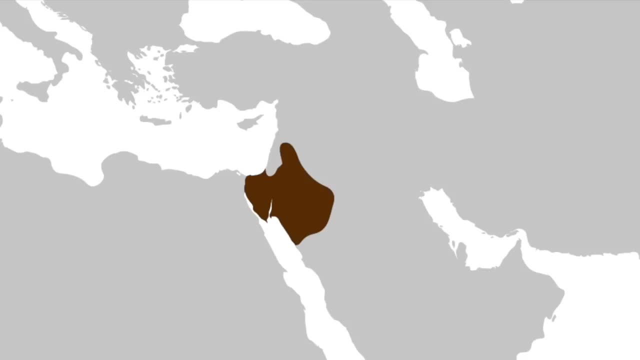 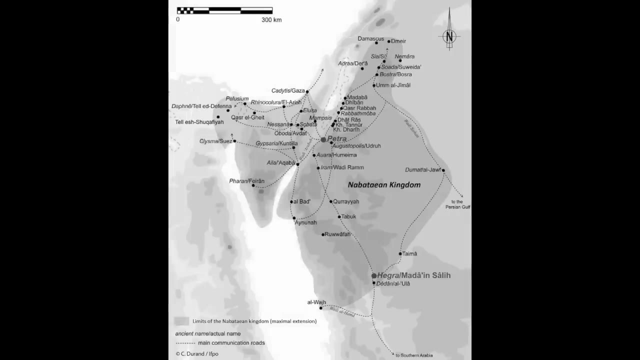 The Nabataeans. These guys were Arabs who lived in what's now Jordan, Israel, the Sinai and northwestern Saudi Arabia, who were organized into a single kingdom, The Kingdom of Nabataea, whose capital was the city of Petra. 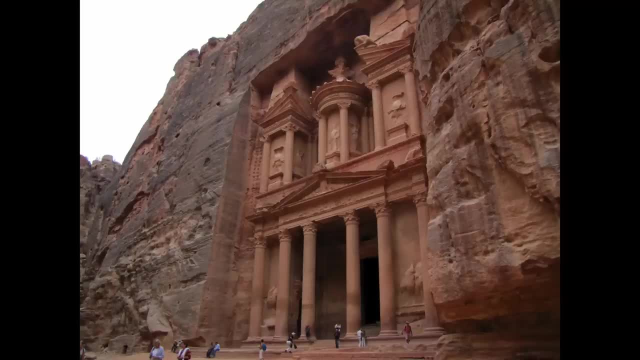 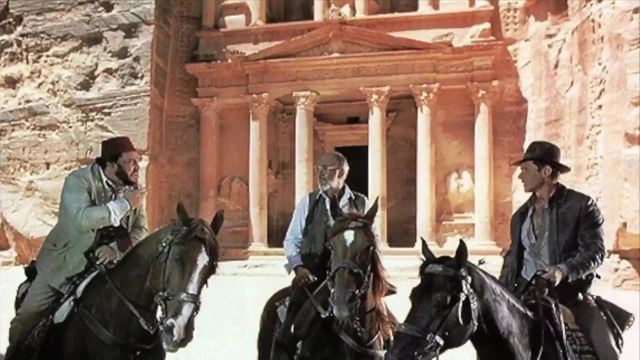 most famous for featuring enormous funerary monuments cut into the very walls of the sandstone canyons where the city was built- You've probably seen it if you've ever watched Indiana Jones and the Last Crusader- because its most famous building, known as Al-Qasna- 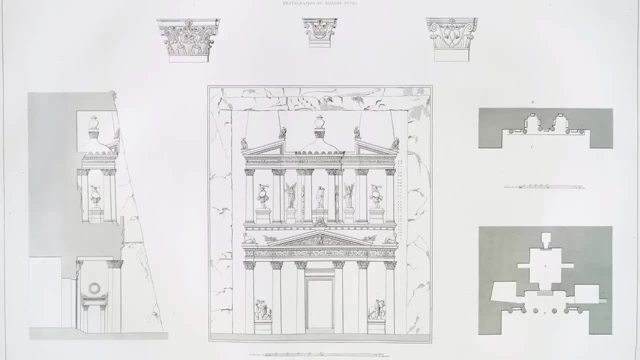 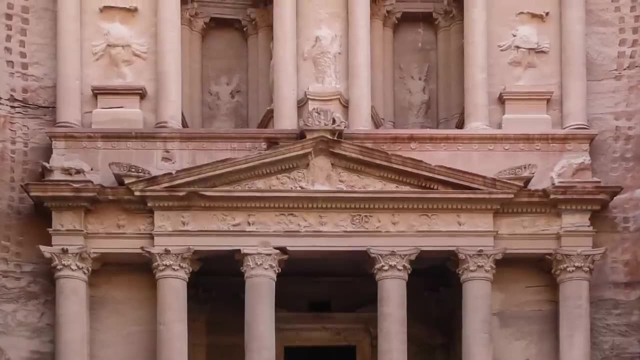 or the Treasury, was where the Grail was. It was most likely a mausoleum dedicated to the Nabataeans' greatest king, Aretas IV, of the early first century, but it actually got its name because the Bedouins of the region believed it was filled with a pharaoh's treasure. and that's why the urn at the very tippy top is riddled with scars from their bullets. The Nabataeans were able to build such amazing monuments because they were stinking rich off of taxing the incense caravans linking southern Arabia with the Mediterranean. and they only built Petra in the middle of the desert because it was along that caravan route, and they built incredibly elaborate waterworks, cisterns, aqueducts, to make it more hospitable. They also built other impressive cities, like Hegra, further to the south in what's now Saudi Arabia. and Avdat now in Israel. Their kingdom was already thriving by the late 4th century BC, but its first known king ascended the throne in 168 BC. From that time until its fall, it was notable for playing a very important role in the politics of neighbouring Judea. 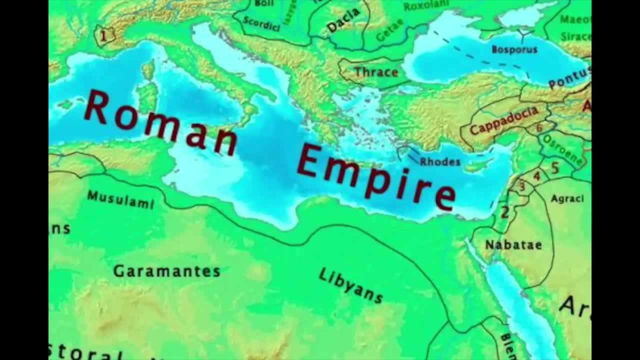 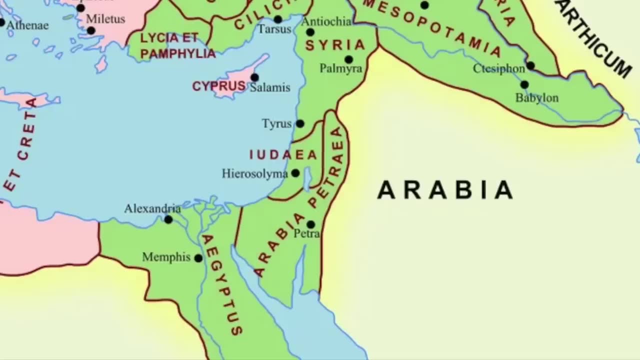 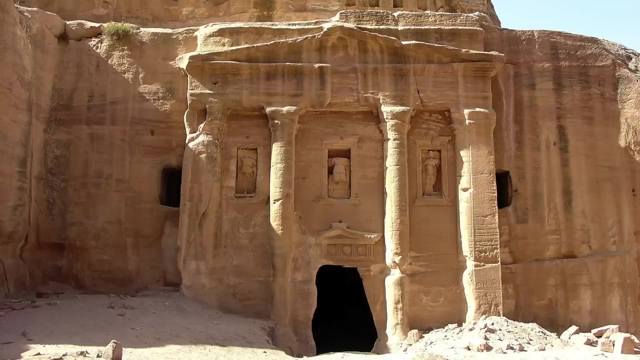 and for managing to fend off the Romans for centuries. But of course it was eventually annexed into the Roman Empire in 106 under Trajan, then becoming the province of Arabia, Petraea, and thereafter it underwent a steady decline because it didn't have the same significance to the Romans or to the incense trade as before. 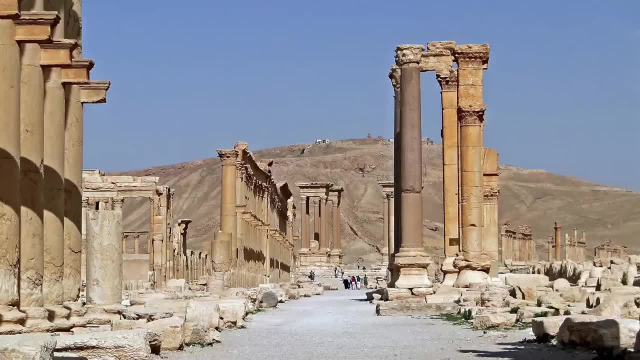 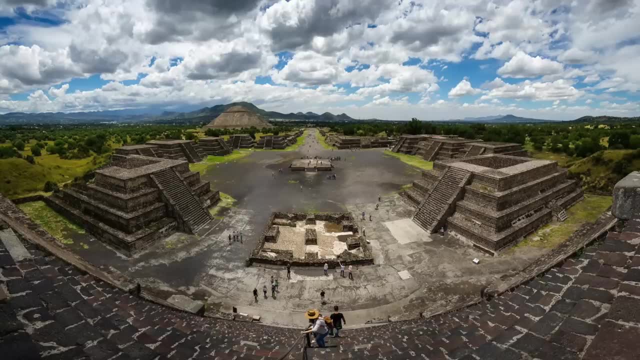 and it was eclipsed by Palmyra, further to the north, Teotihuacan. Some people were surprised by the fact that Teotihuacan is this far down, because among people familiar with Mesoamerican history it's very well known. 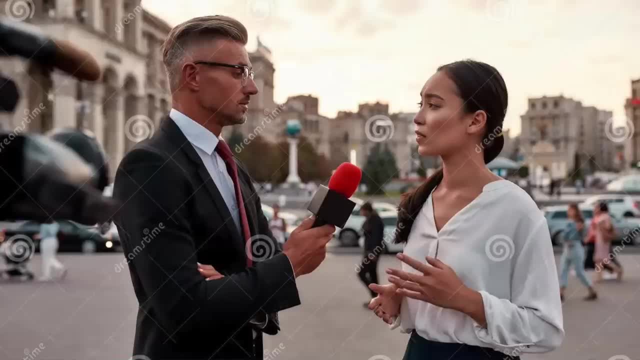 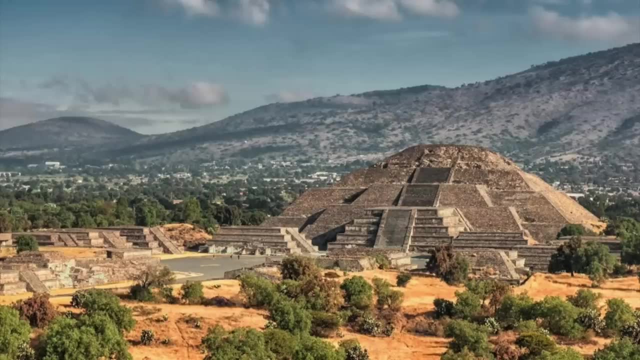 and of course, anyone living in central Mexico knows about it. but if you asked any random person on the street about it anywhere else, they'd probably have no idea what you're talking about. But it's a spectacular, ancient city just 40 kilometers northeast of Mexico City. 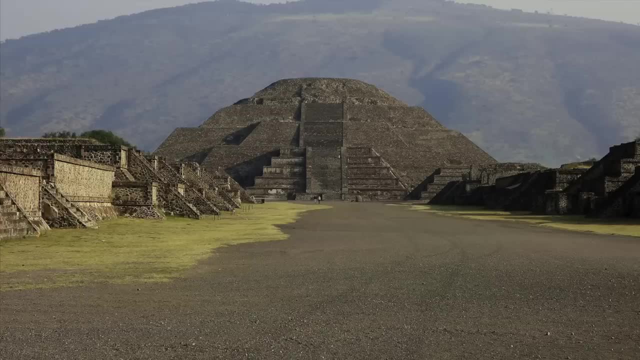 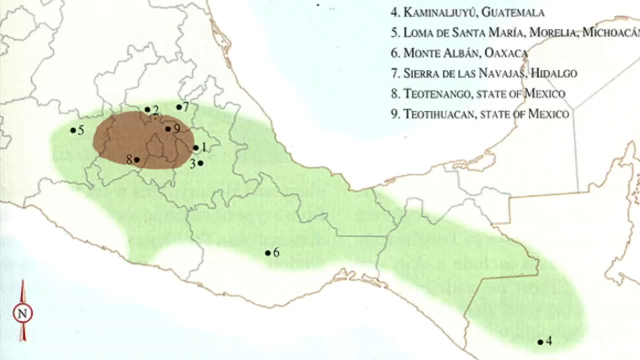 and long after it was abandoned, the Aztecs were so in awe of it that they referred to it as the birthplace of the gods, or Teotihuacan. It totally dominated Mesoamerica and had one of the biggest populations of animals. 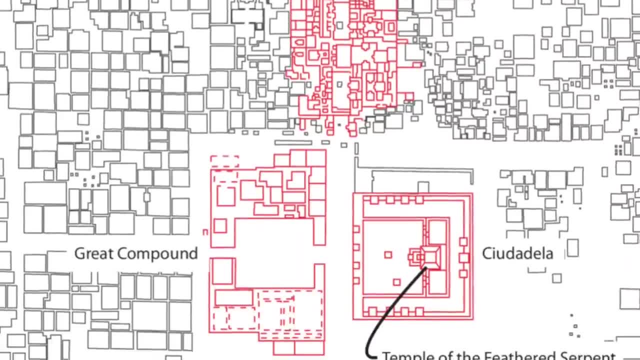 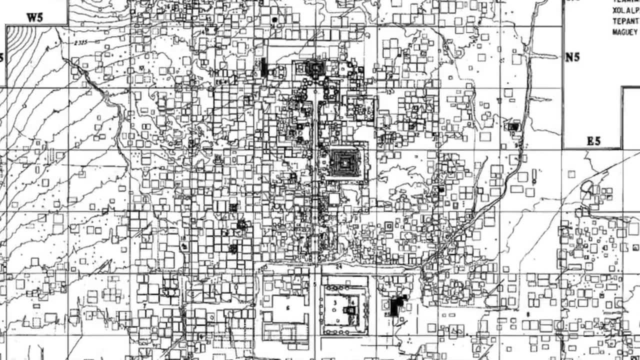 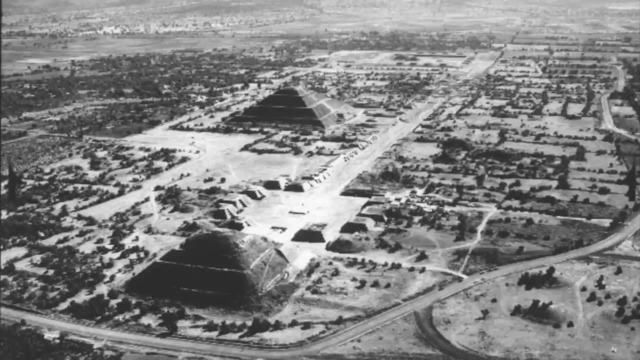 in any city in the world, at its height between 400 and 600 AD, holding between 1 and 200,000 people. It was a very well-planned city comprised of a complex grid filled with multi-level apartment buildings, But the two most notable structures at Teotihuacan are, of course, the two enormous pyramids there. 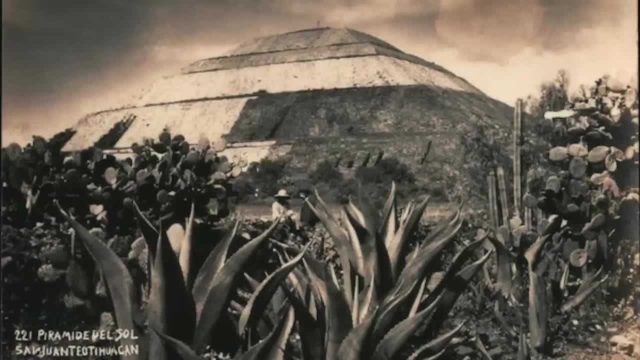 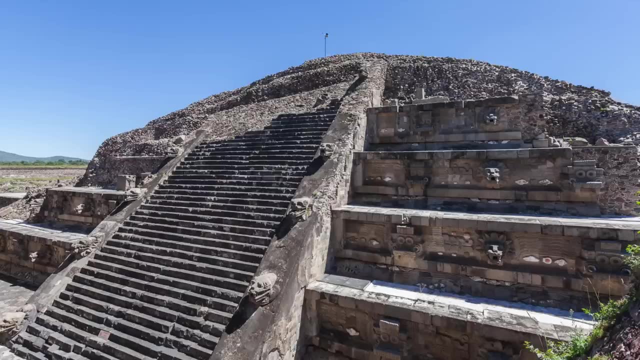 the Pyramid of the Sun and the Pyramid of the Moon, the former of which is the second biggest pyramid in all of Central America, Which makes sense. just look at it. The site's third largest pyramid, the Temple of the Feathered Serpent. 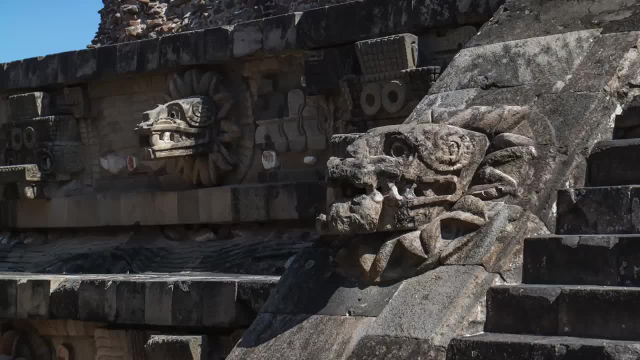 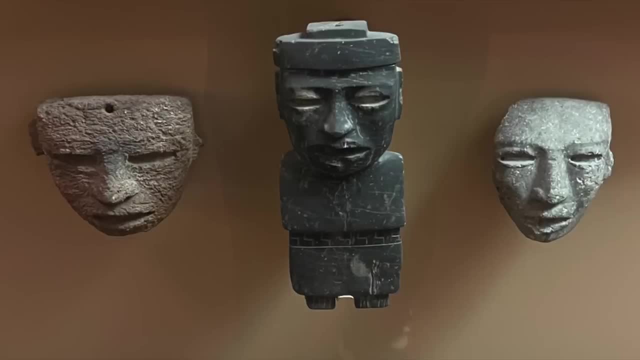 is covered in- you guessed it- feathered serpents, and hundreds of sacrificial burials have been found beneath it. The city is also famous for having produced huge quantities of distinct greenstone masts and for the beautiful murals painted onto its more upscale residences. 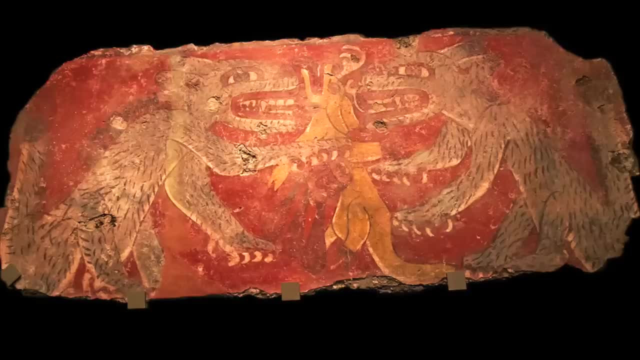 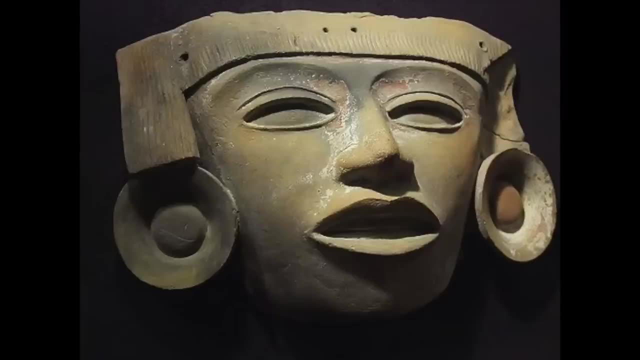 Somewhat strangely, these don't really ever depict anything political, and no inscriptions were written in Teotihuacan, so we don't really have a clear picture of what their government looked like, or even if they had kings. But either way, 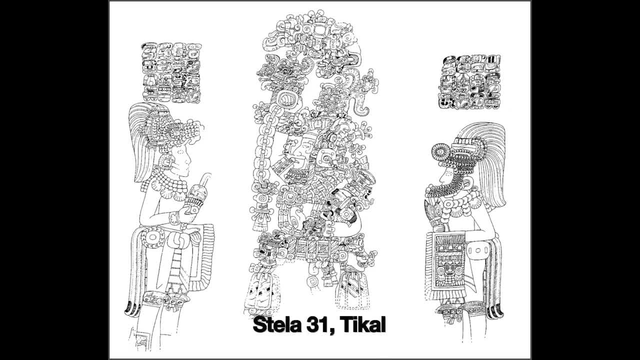 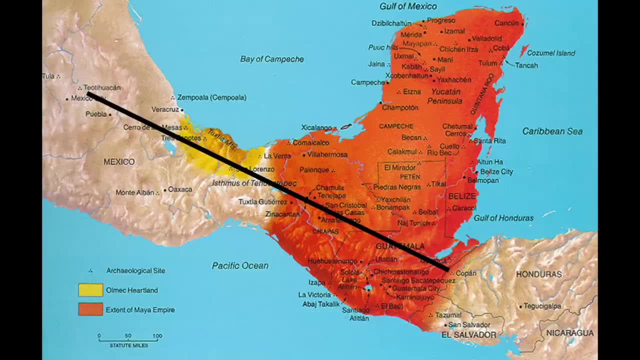 the city has heavily, heavily influenced the Maya, and people from Teotihuacan were able to install themselves as the rulers of the great Maya cities of Tikal and Copan, hundreds of miles away from Teotihuacan. This was during the 4th and 5th centuries. 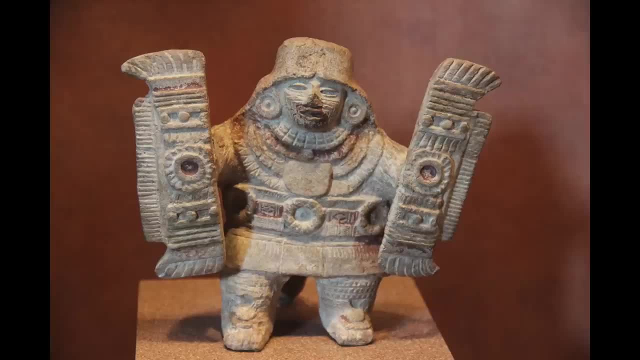 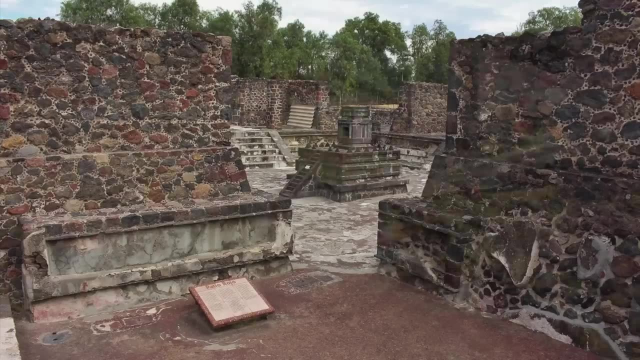 But we still don't know if Teotihuacan really formed an empire per se. In the mid-7th century. the dwellings of the ruling class in particular were recurrently ravaged and razed, possibly reflecting an invasion or even an internal revolt. 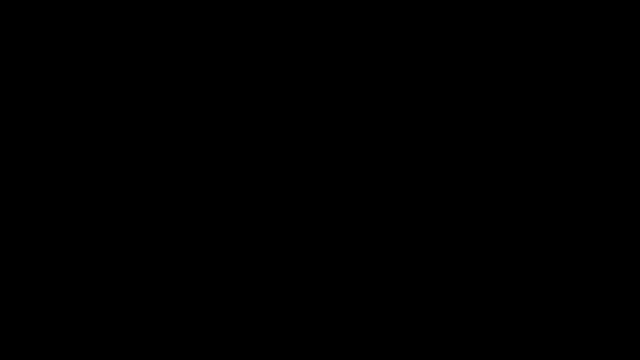 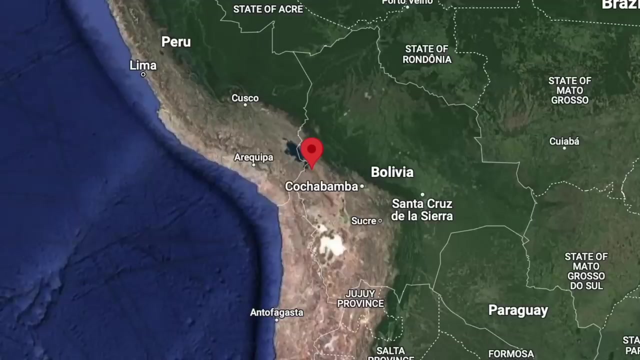 But either way, the city was eventually abandoned. Tiwanaku, Like Teotihuacan, it's a single grand city and a civilization to boot. It's located on Lake Titicaca, one of the highest lakes in the world, in Bolivia. It emerged sometime between 200 BC and 200 AD, but it was preceded by other major city-states in the Lake Titicaca Basin, like Chiripa and Pucara. It's 12,600 feet above sea level and the Altiplano or high-altitude plains surrounding the lake. 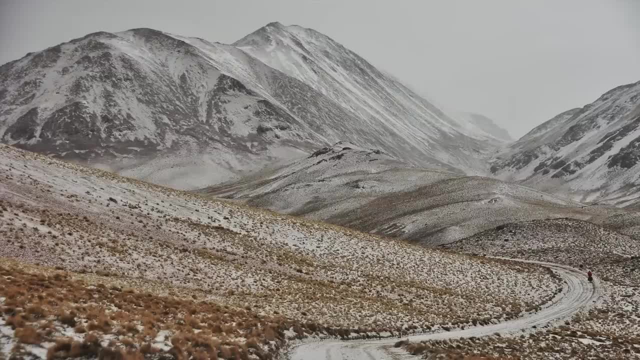 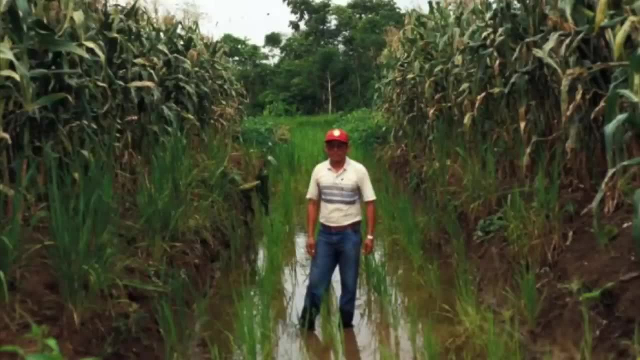 are pretty inhospitable. So to circumvent this, the people of Tiwanaku used something called raised-field agriculture, which was able to sustain a higher crop density than usual and kept the crops warm during the Altiplano's frigid nights. 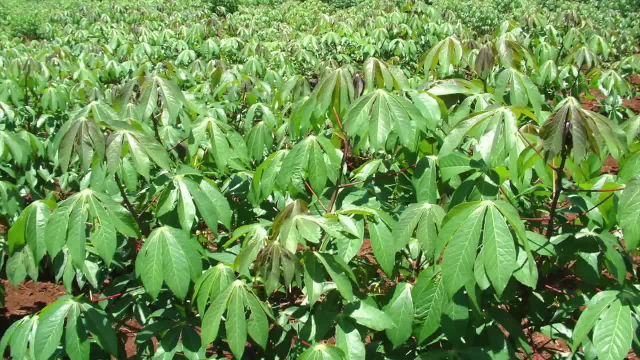 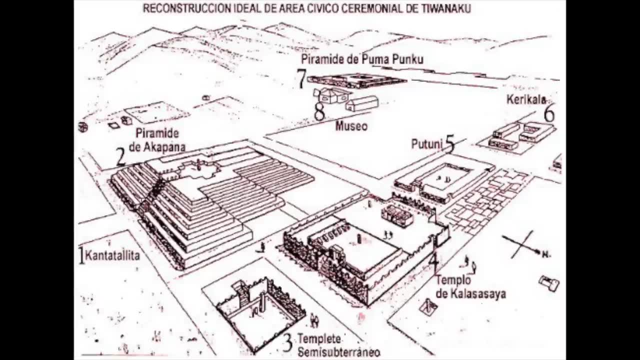 And despite how banal it sounds, the surplus food this system created was the thing that fueled the monumental building projects which define Tiwanaku. A bunch of them are clustered into a ceremonial center, once separated from the rest of the site by a big moat. 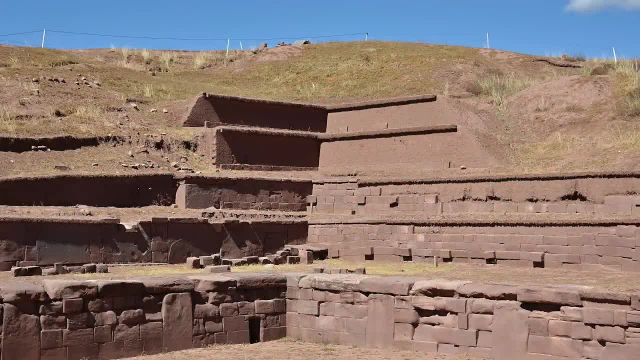 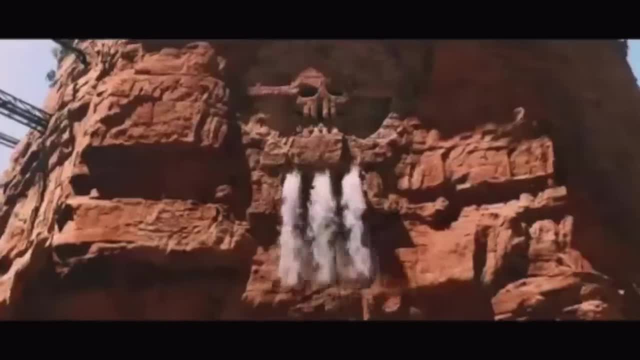 like a large, badly-eroded pyramid known as the Acapana. It featured big drainage canals which made it resemble an artificial mountain spring, Which sort of reminds me of that thing from Mad Max. you know It also features a semi-subterranean temple. 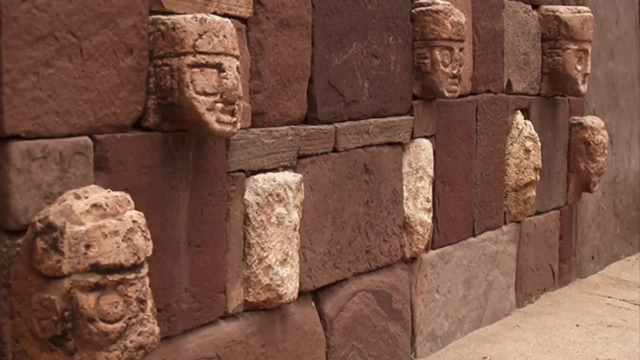 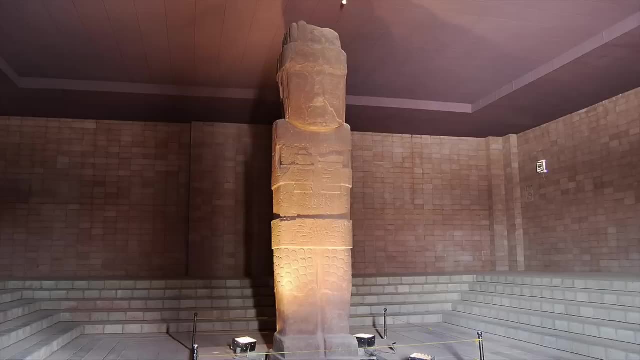 whose walls are lined with stone heads, like that temple from the beginning of Raiders of the Lost Ark, Except they don't shoot poison arrows. luckily for the tourists, This temple is also where a huge, seven-meter-high statue known as the Bennett Monolith. 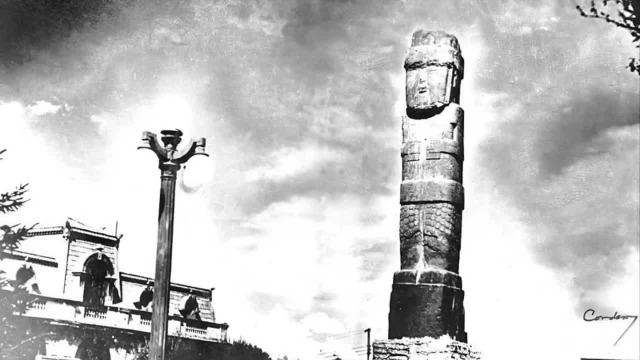 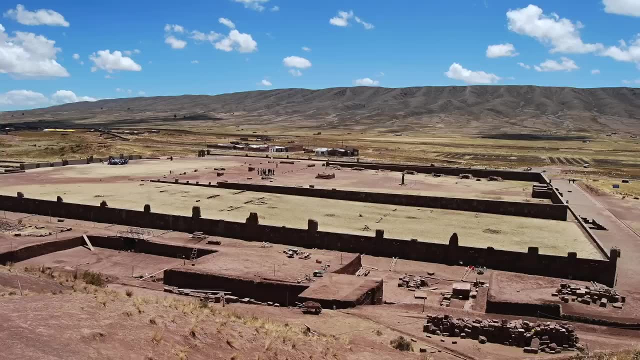 once stood. For decades it was displayed in La Paz and it's now in the site museum, notably holding a snuff tray for sniffing hallucinogens. And finally, there's the Kalasaya, a huge temple complex featuring more colossal statues. 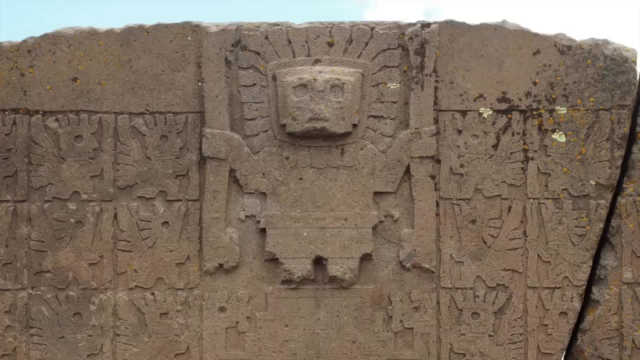 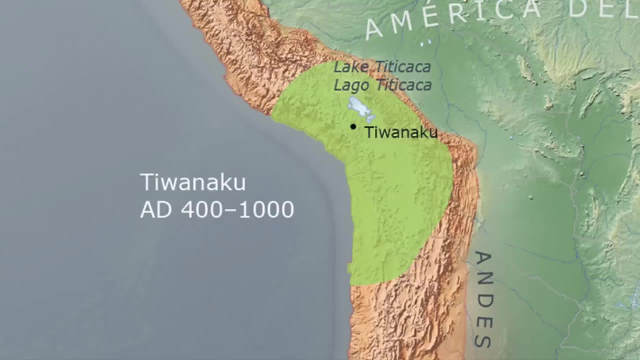 and the magnificent Gate of the Sun. As amazing as they are now, imagine them once covered in gold. Outside the ceremonial center there's also another pyramid called Puma Punku. Tiwanaku formed one of the first empires in the Americas. 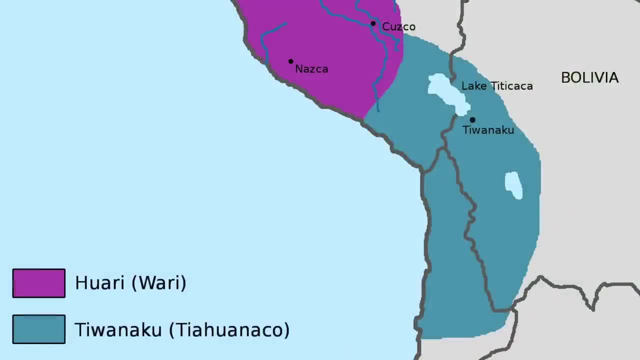 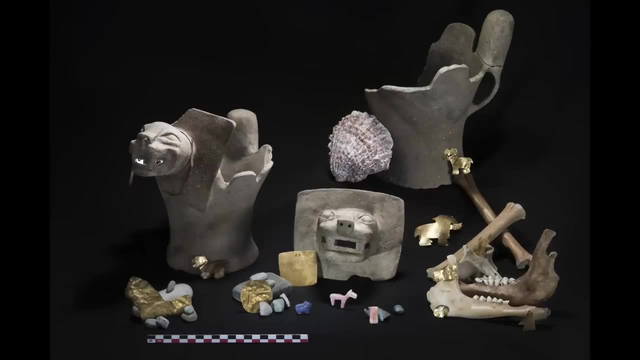 reaching its zenith between 500 and 1000 AD, when it created tons of colonies and trading posts and just proliferated its culture absolutely everywhere across the region. it was in. One of the main goals of this empire building was to secure various luxuries for the elite. 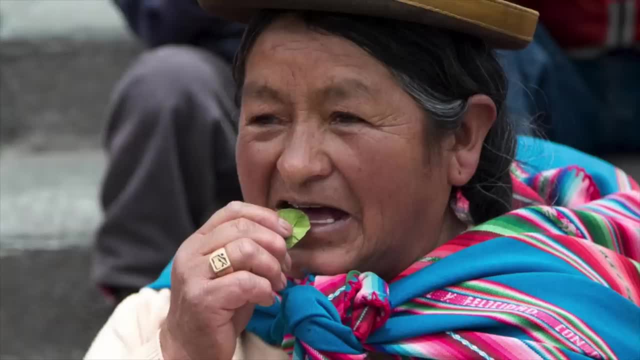 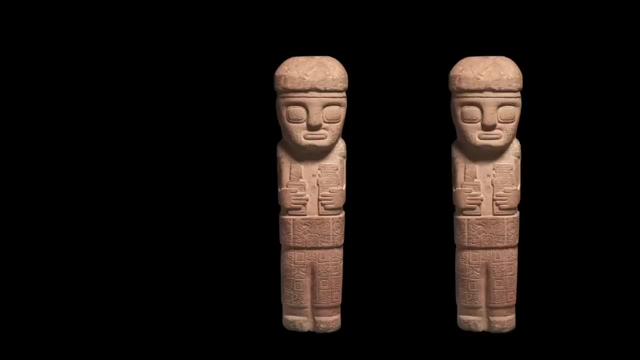 like coca leaves and we literally have statues of Tiwanaku elites chewing coca. But ultimately, the city was also able to sustain a population of up to 70,000 people, even though, as mentioned before, it's 12,000 feet above sea level. 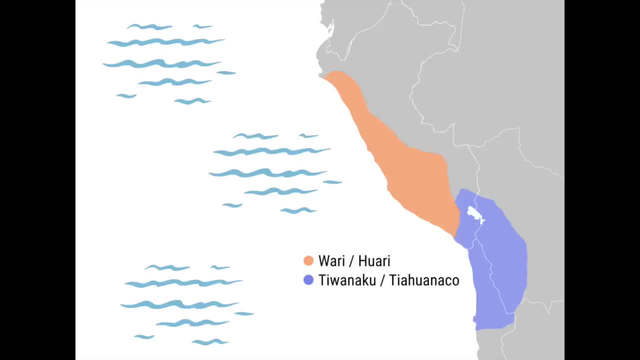 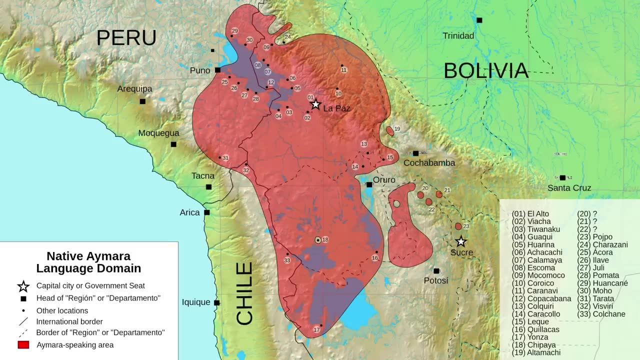 It greatly influenced the succeeding Inca and while they were around they were rivals of the Wari Empire. but it collapsed around 1000 AD from an onslaught of various Aymara kingdoms and a severe drought, which also helped bring down the next civilization on this list. 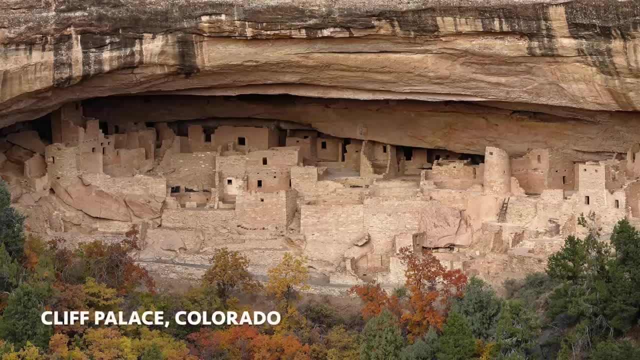 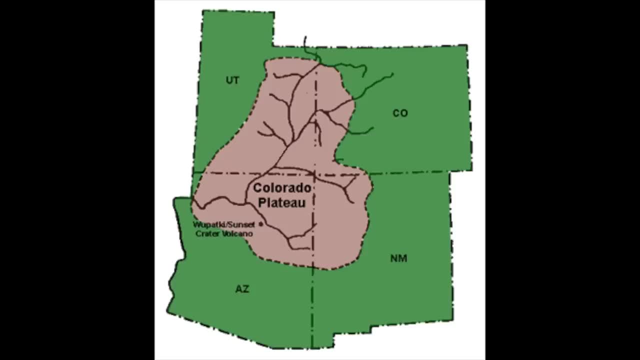 the Anasazi, also known as the Ancestral Pueblo. I put them here because they're pretty well known in the American Southwest where they lived. More specifically, they lived in the Colorado Plateau, where the four states of Colorado, Utah. 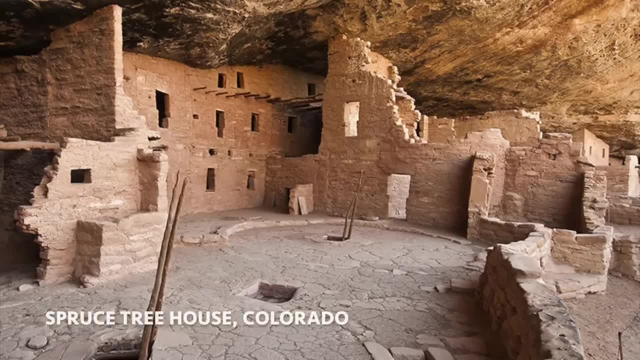 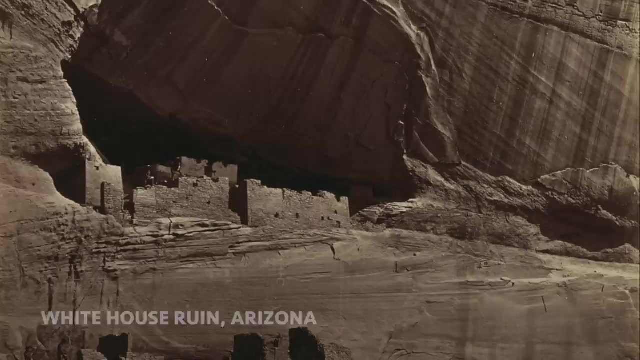 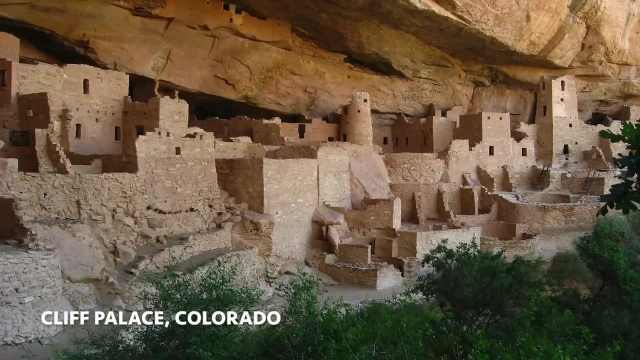 Arizona and New Mexico come together And they're well known because they left some pretty amazing monuments behind, Most famously the massive and incredibly evocative defensive cliff dwellings they created, which are now located in various national parks, like Cliff Palace and Mesa Verde National Park. 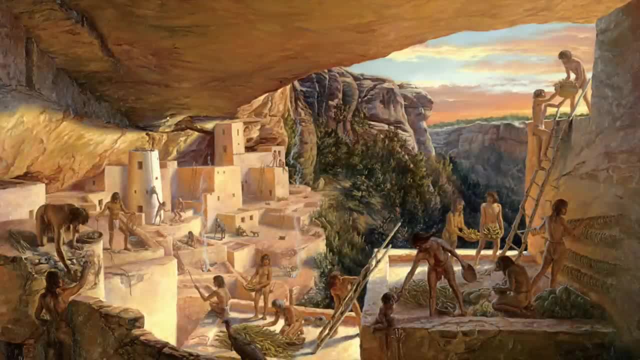 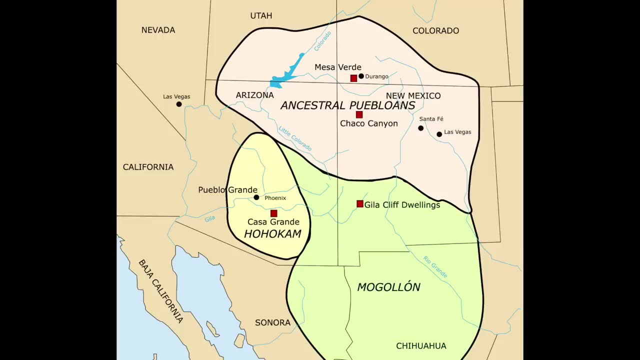 They're incredible multi-story complexes that once housed hundreds, even thousands, of people. They're also one of the primary prehistoric archaeological traditions in the Southwest, along with the Hohokam and the Mogollon, a region also referred to as Oasis America. 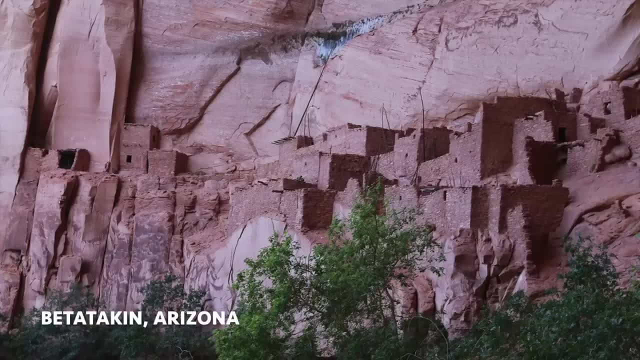 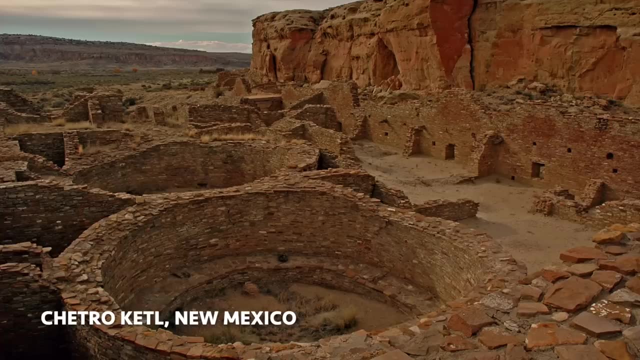 You know, like Mesoamerica, I'm pretty sure the Anasazi are the best known of the bunch, given all the monuments they left behind. In addition to the cliff dwellings, they created so-called great houses, the largest of which being Pueblo Bonito. 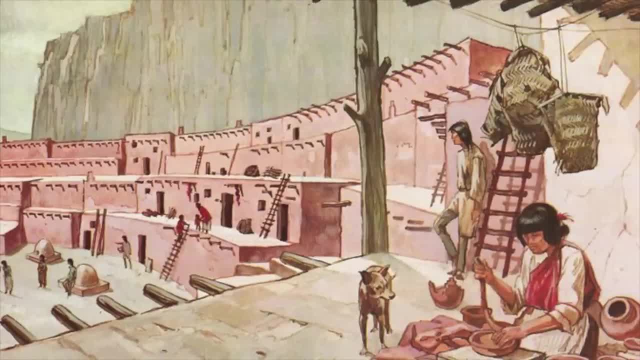 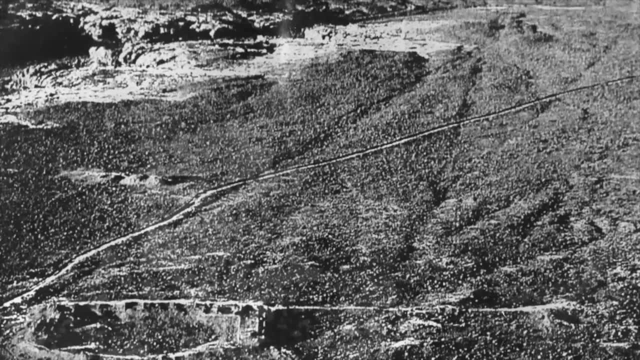 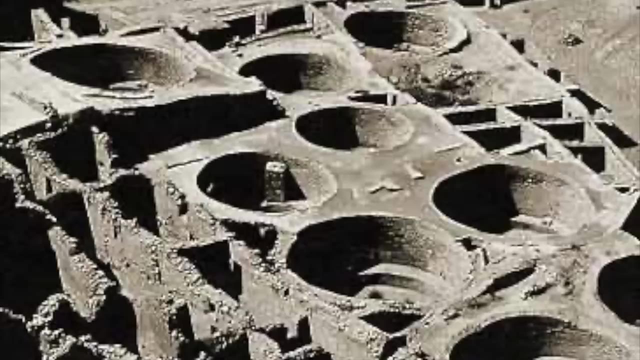 with 700 rooms in it and one standing at five stories tall, And they also built vast road networks connecting them all, which facilitated the transport of far-flung luxury goods like macaws and turquoise. Their lives were centered around, usually semi-subterranean ceremonial structures called kivas. some of which called Great Kivas, are truly vast. They emerged as a distinct civilization in the 12th century BC, but they started actually building pueblos around 750 AD, But eventually in the 12th and 13th centuries AD. 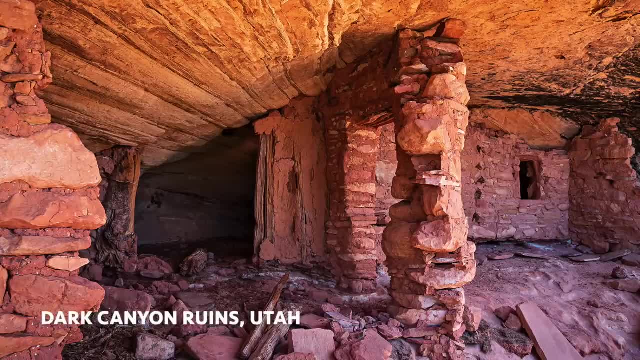 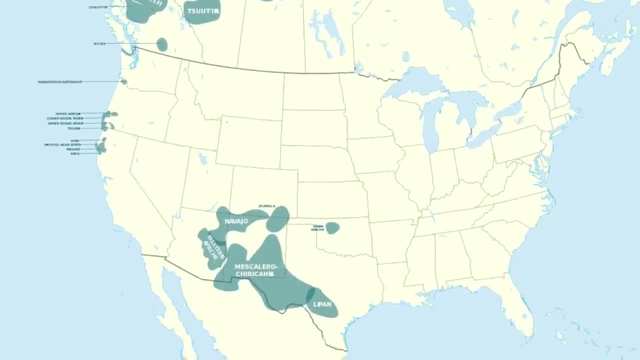 they abandoned their established communities, probably due to a mixture of the climate, becoming more arid, environmental degradation, as well as Numic and Athabascan-speaking migrants. In fact, the modern Pueblo object to them being called the Anasazi. 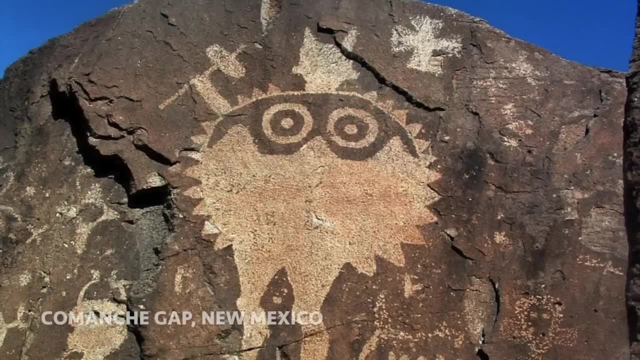 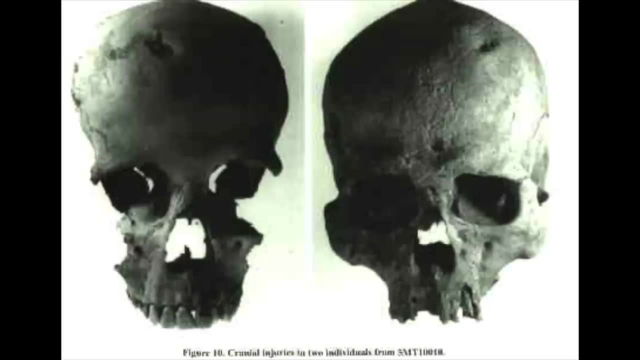 because it's a Navajo word meaning something like ancient enemy. But whatever happened was pretty horrible. For instance, at Cowboy Wash in Colorado, seven dismembered bodies were found that may very well have been cannibalized. Ultimately, they were forced to migrate towards the south and east. 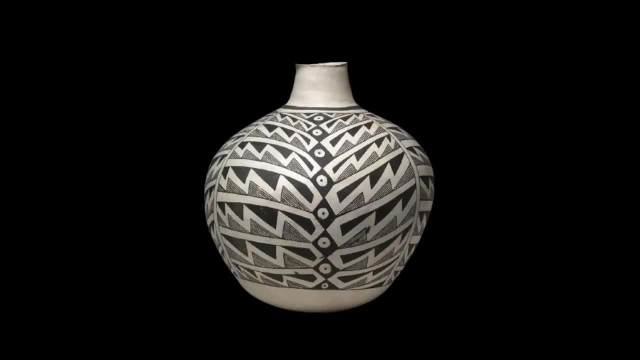 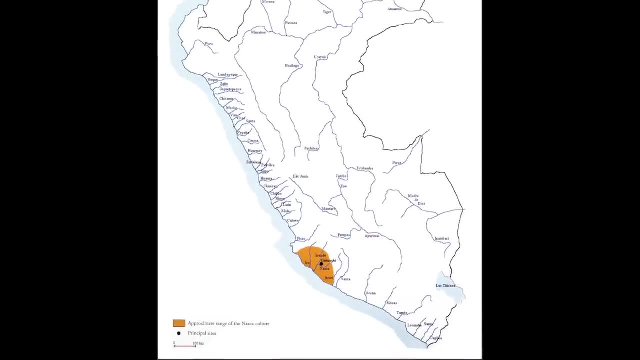 further into New Mexico where the modern Pueblo live. They also made really cool pottery- The Nazca. The Nazca lived along the harsh desert coast of southern Peru. They emerged as a distinct culture in the 1st century AD, succeeding the Paracas culture. 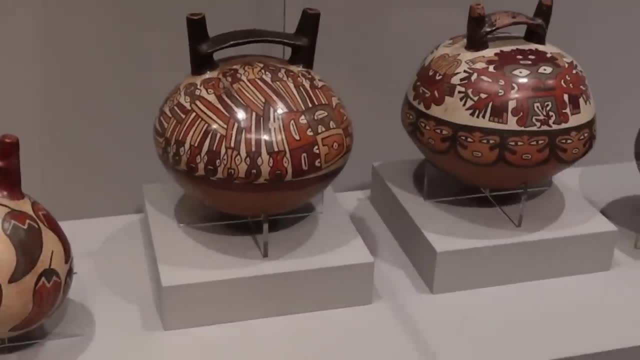 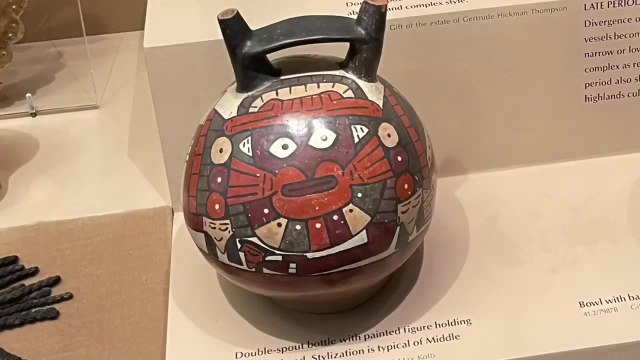 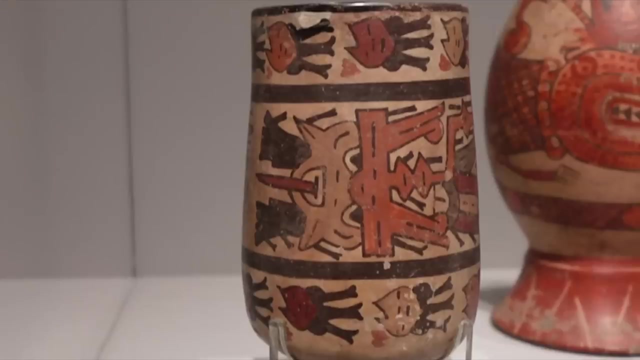 They created amazingly vivid pottery, which is one of our only windows into their mythology and ways of life. They bear images of bizarre beings like the creatively named anthropomorphic mythical being, the horrible bird and the mythical killer whale. They also really liked headhunting, for some reason. 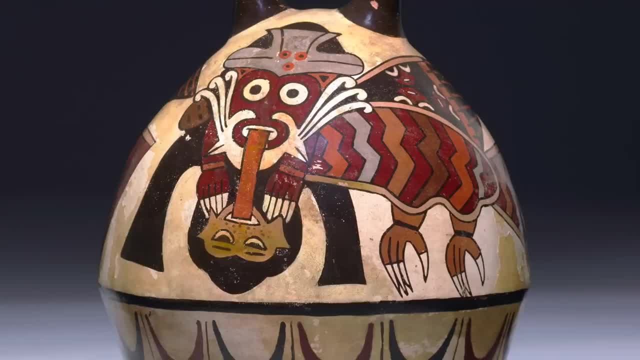 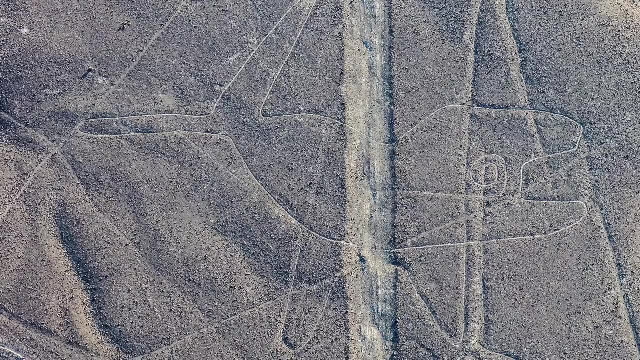 and you can spot decapitated heads on nearly every bit of pottery they made. But of course, they're most known for being behind the Nazca lines, enormous geoglyphs, most famously depicting animals, but also depicting humans, plants and insects. 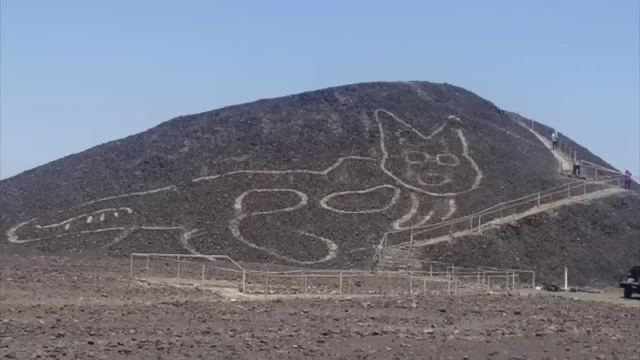 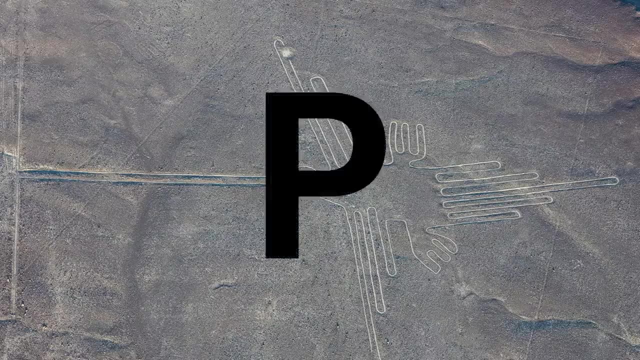 along with spirals and even just massive linear designs, which their forebears, the Paracas, also built. So how were they built and why? People look at them and think that it would have been impossible to make them without being able to see them from the air. 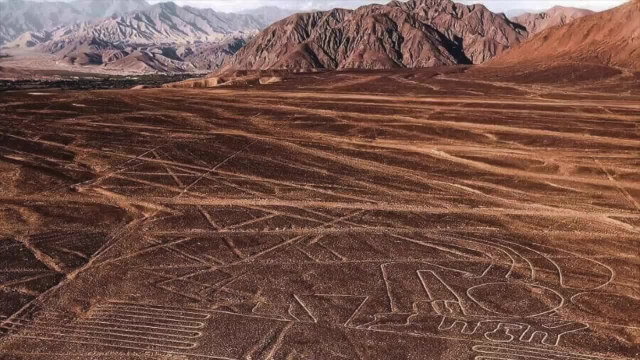 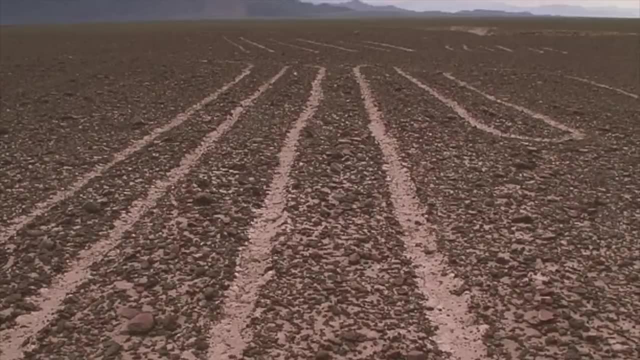 which has fueled a bunch of conspiracy theories. and it's true that they were only really rediscovered by pilots in the 20th century. but all they did was clear the stones covering the desert surface to create certain patterns using simple surveying tools. 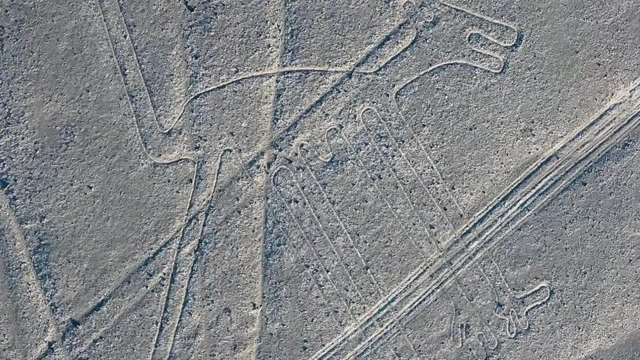 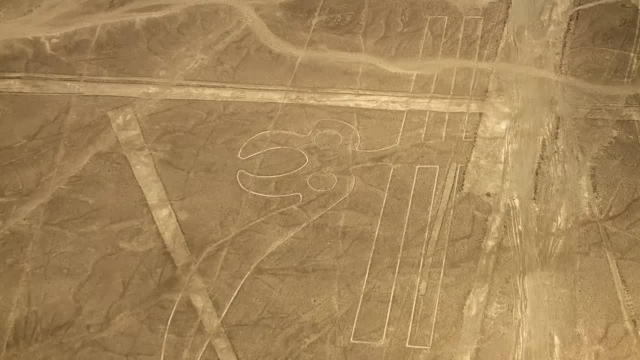 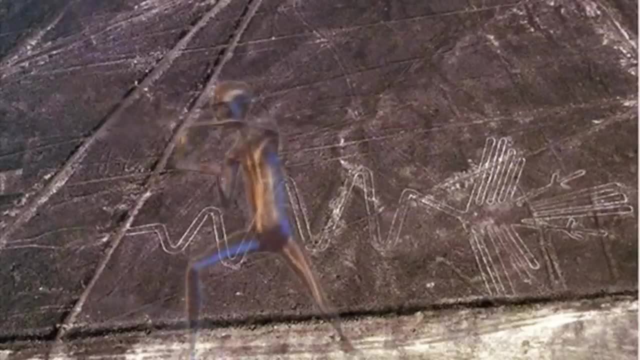 The real question is: why were they built? And a bunch of theories have been put forward to explain it, like that they were processional pathways, ceremonial centers, a massive astronomical calendar that they follow underwater aquifers and, of course, that they're runways for alien spaceships. 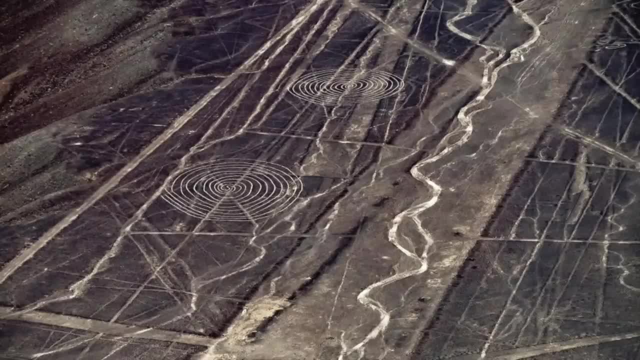 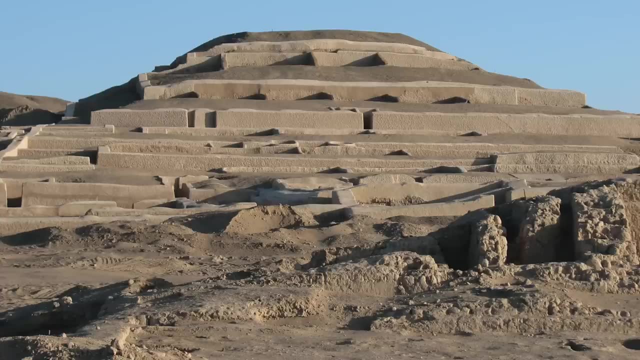 But with the exception of the alien landing strip theory, the jury's still pretty much out on that one. No one really knows why they built them. Until 450 AD, the culture was dominated by a ceremonial and pilgrimage center known as Cahuachi. 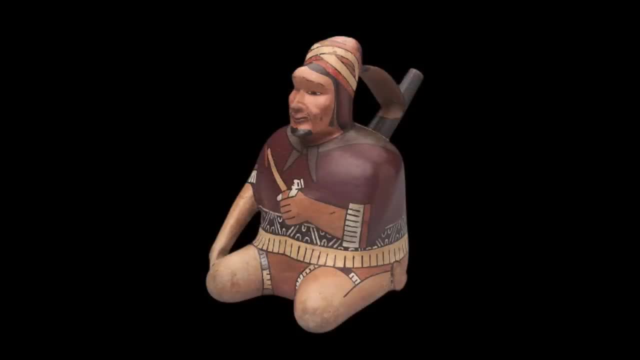 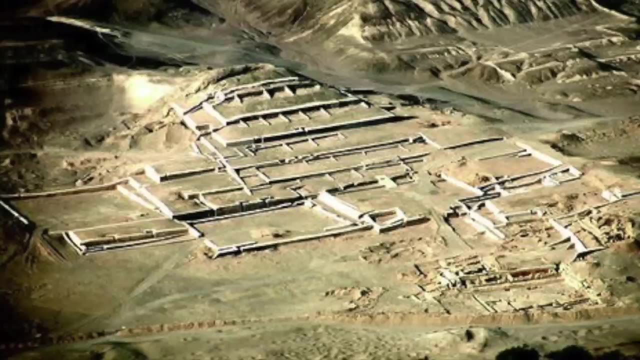 and it was loosely controlled by some sort of theocratic authority. After 450, the culture sort of collapsed and Cahuachi was abandoned along with the old religious order. This marks the end of what's known as the early Nazca period. 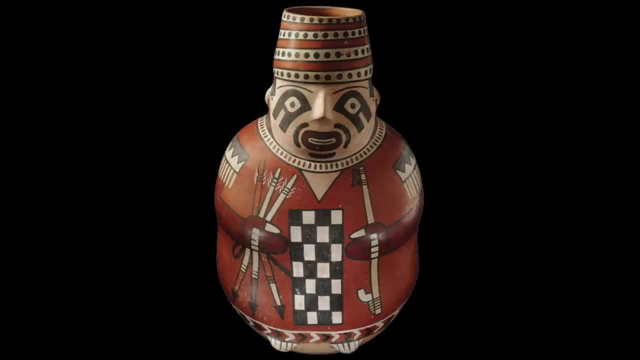 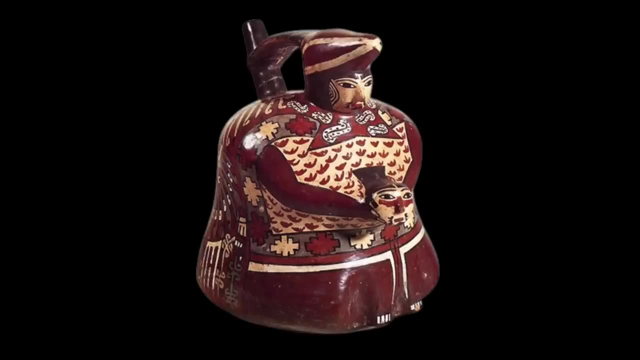 By 550, the Nazca reemerged, with local warring chiefs in charge. Warfare starts being the main focus on pottery, and head hunting somehow became even more important than before. They also mummified the heads. They also started building something known as puquillos. 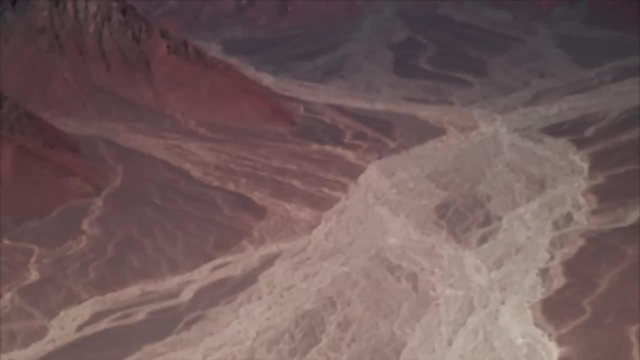 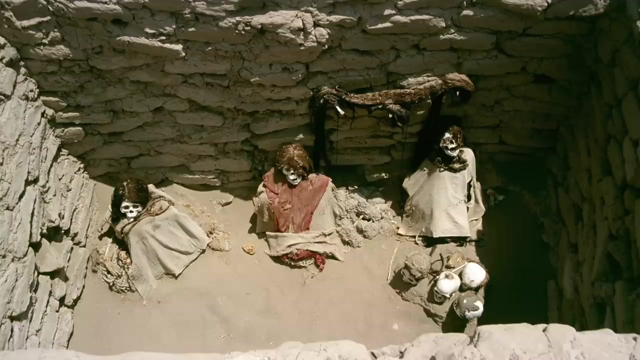 which are underground aqueducts built as the climate was becoming way more arid and rivers more unreliable. Those corkscrew-like depressions you see on the top are actually access shafts. The Nazca culture collapsed for good sometime between 750 and 800 AD. 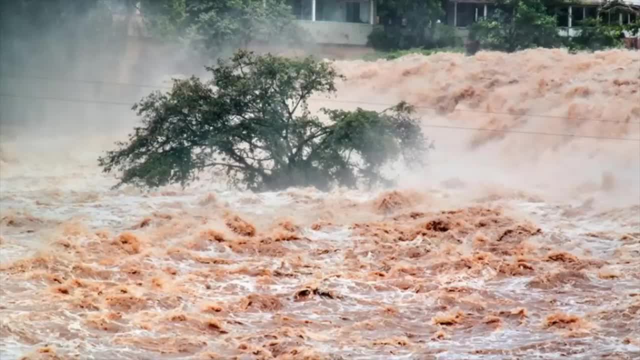 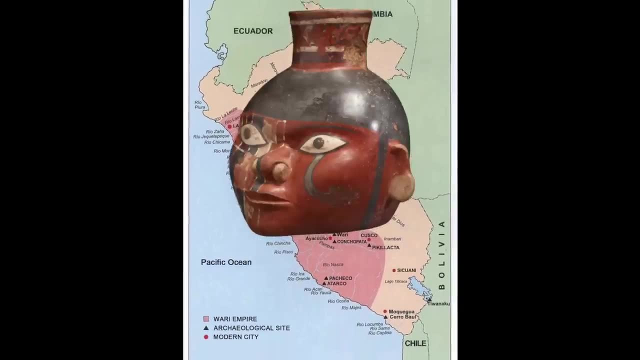 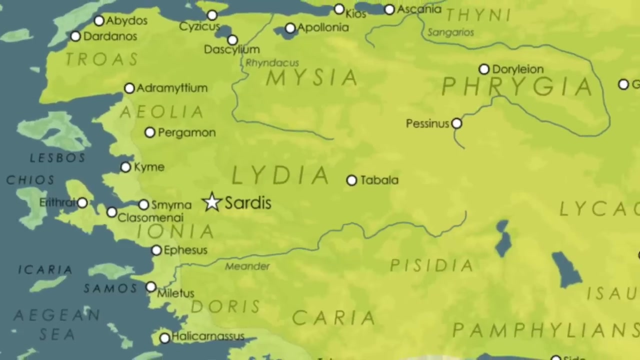 possibly due to the effects of El Niño flooding, exacerbated by deforestation, and eventually the region they occupied was taken over by the Wari Lydia. Now we're returning back to the old world. Lydia was a kingdom and region in western Anatolia. 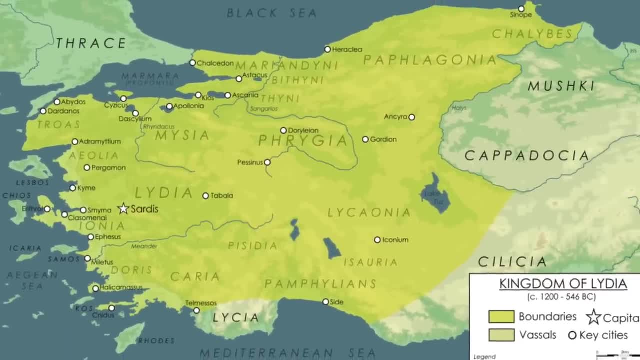 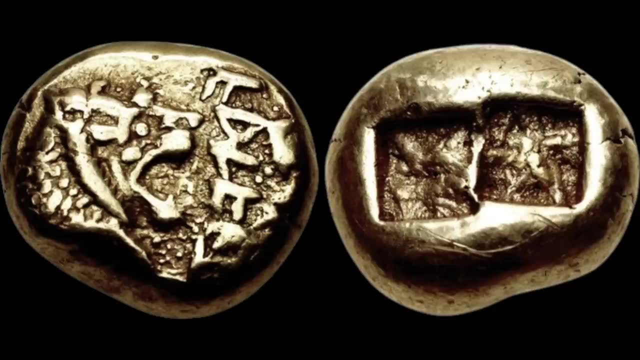 which flourished in the 7th to 6th centuries BC. It's most well known for minting the world's first proper coins out of a natural alloy of gold and silver called electrum, and it's also known for its last independent king. 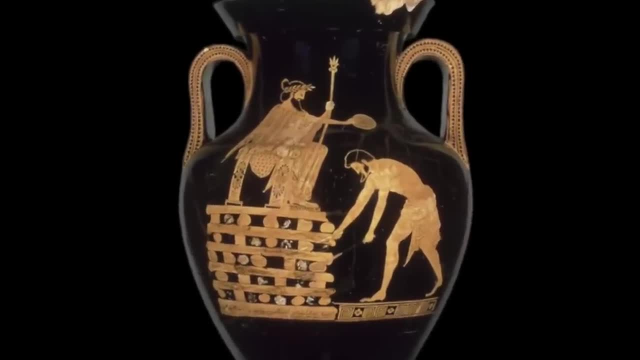 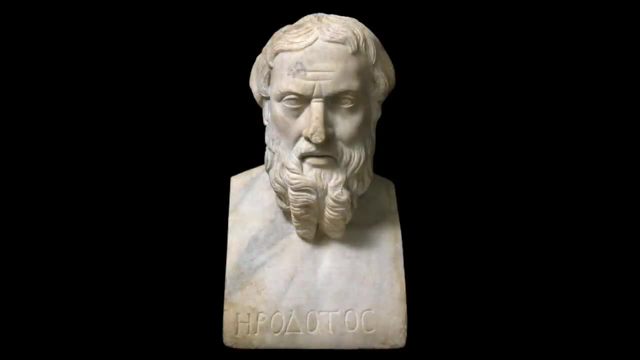 Croesus, who was the richest man in the world in his day. His dynasty, the Myrmnad dynasty, was founded in a really bizarre way, and it's one of the first things mentioned in Herodotus' histories, The last king of the previous dynasty. 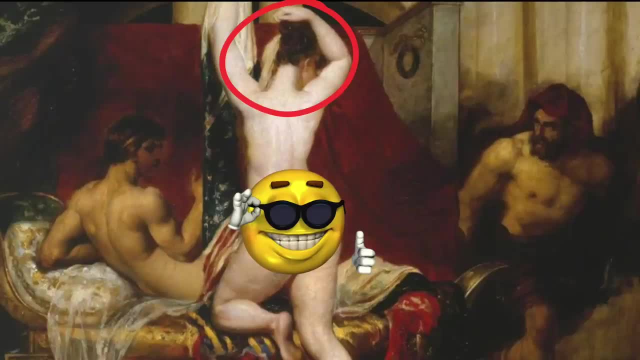 Candaules thought his wife Nisia was the most beautiful woman in the world and to prove it to his friend and bodyguard Gyges, he pressured him into hiding in her room to watch her undress. Nisia found out and, understandably, 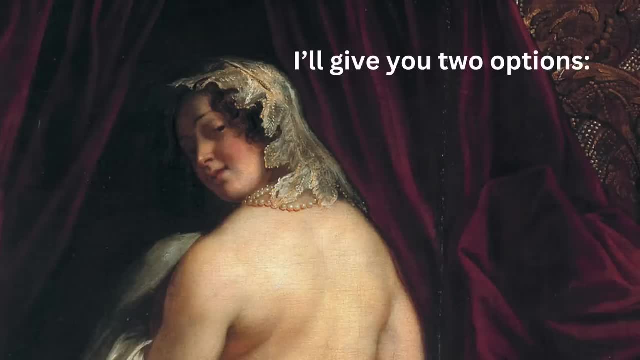 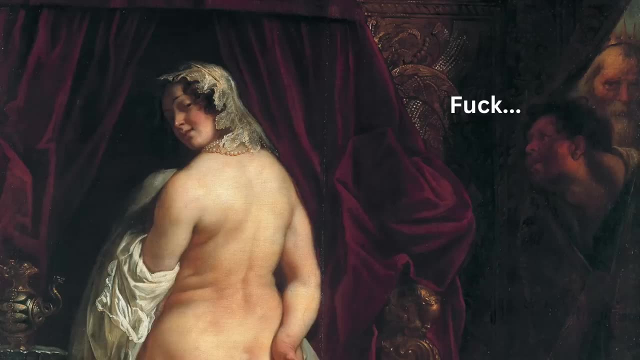 was a bit angry. so she offered Gyges two choices: Murder Candaules and usurp the throne with her as his wife, or be executed. She claimed that he raped her. Let's just say, Gyges pulled a real Griffith and killed his friend in exchange for power. 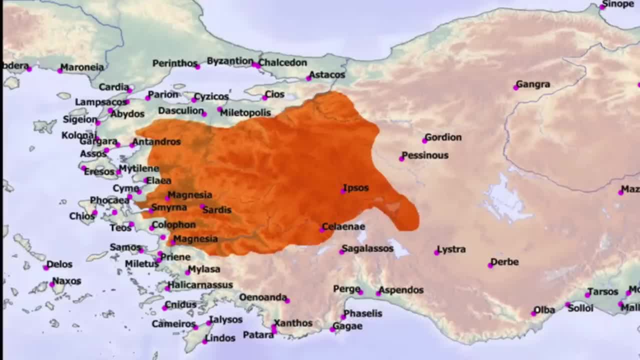 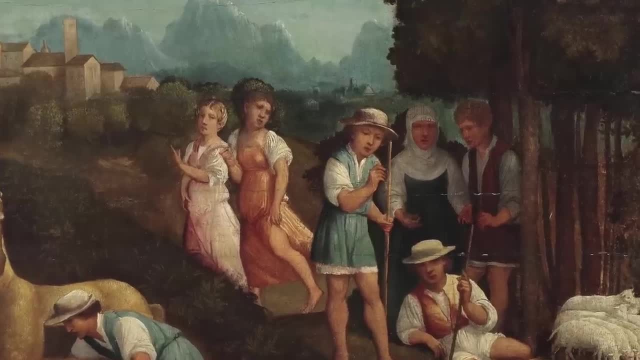 starting Lydia on its path to becoming a great empire by campaigning against the neighboring Cimmerians and Ionians. Plato, on the other hand, told a different tale: that Gyges instead usurped the throne using a magical ring that was able to turn him invisible. which might sound familiar. Croesus was the last king of Gyges' dynasty and even though he expanded Lydia to its greatest ever extent, he was defeated by Cyrus the Great of the Persian Empire in 547 BC at the Battle of Thimbra. And after his capital, Sardis, was captured, Lydia was incorporated into the newfound Persian Empire. Croesus famously asked the Oracle of Delphi whether or not he should go to war against the Persians in the first place, and the Oracle responded by saying: 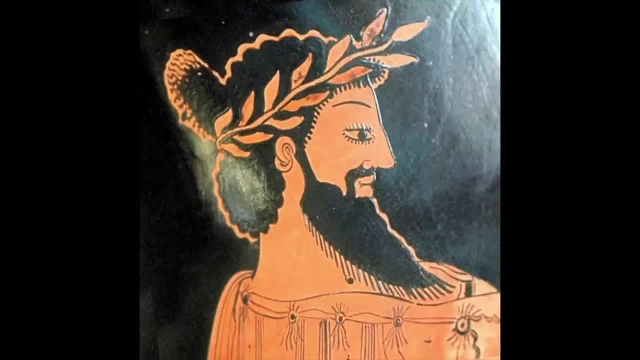 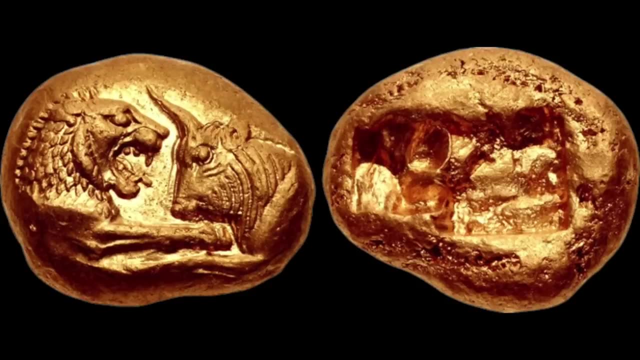 that if he did, he'd destroy a great empire, And Croesus went ahead with the war not knowing that his empire would be the one he'd go on to destroy. Besides its coins, Lydia's greatest legacy is constituted by the hundreds of truly enormous burial mounds. 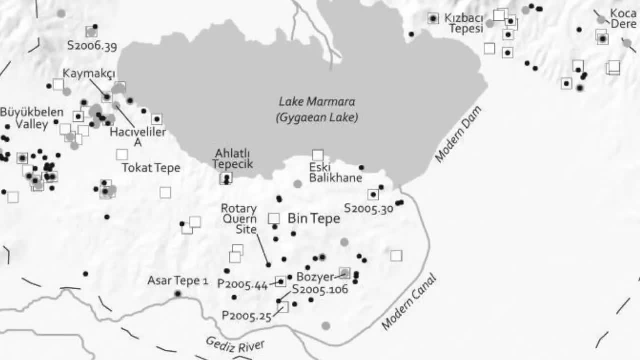 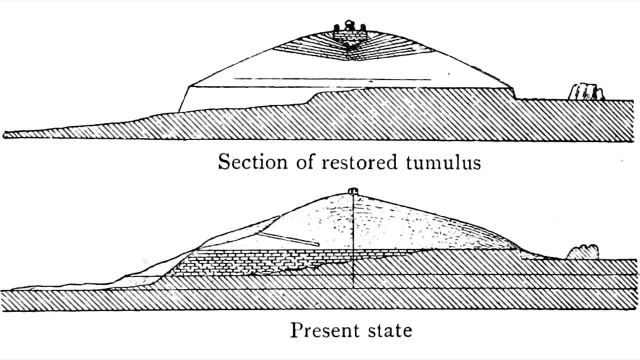 they've built near Sardis, especially at a site called Bintepi. Three mounds in particular dominate the site: The Tumulus of Aliades Croesus' father, which was supposedly mostly funded by prostitutes, Kamyarik Tepi, the burial chamber of which hasn't ever been located. 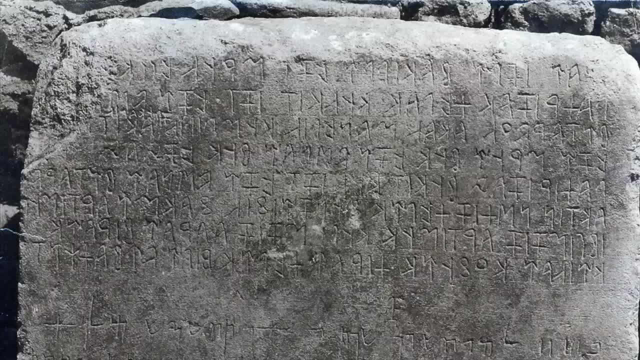 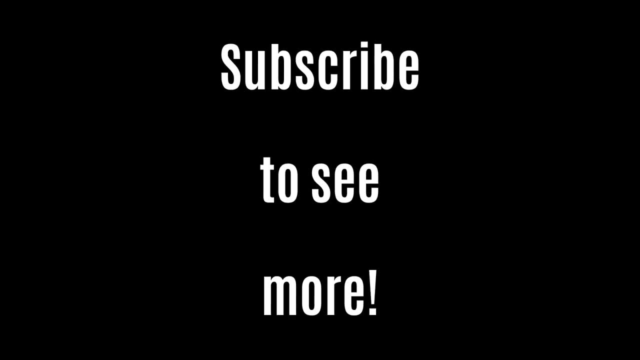 and Kyrmoutaf Tepi. Lydia also had a language which was used up until the first century BC. that's only been partially translated. So that's it for part one. I was originally going to cover six more civilizations in this video. 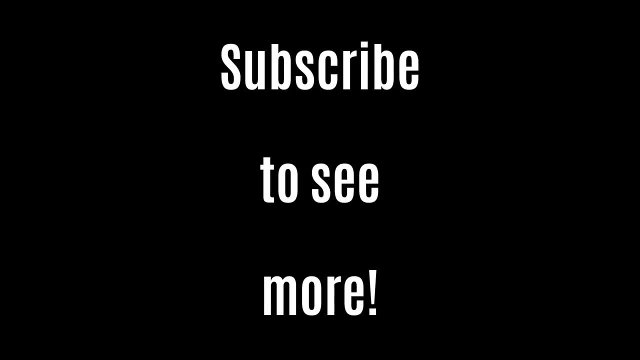 including the Elamites, Gunung Padang, the Yamnaya, the Halstead culture, Aksum and the Philistines. but I'm just getting tired of my own voice, so I'm going to end it off here.